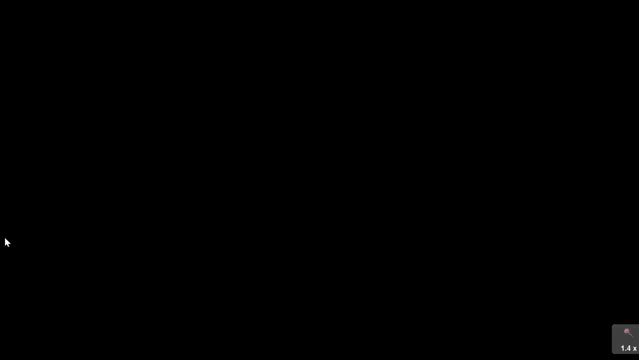 which I assume you might be knowing, but I just want to make sure that whenever I work on these questions, we are on the same page. So let us look at the basics here, and the first part is: whenever you are dealing with moments now, when you define moment of a force, remember it is moment of a force. it. 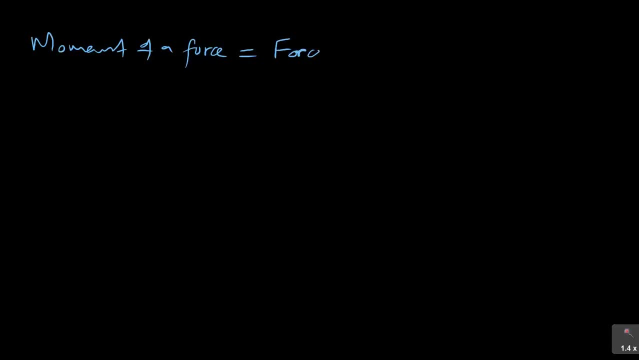 is equal to force, which is the perpendicular force. in this case, it is perpendicular force times the distance from the fulcrum, or the pivot times distance from fulcrum. Okay, Okay. So now what are we talking about when we are talking about the moment of a force? 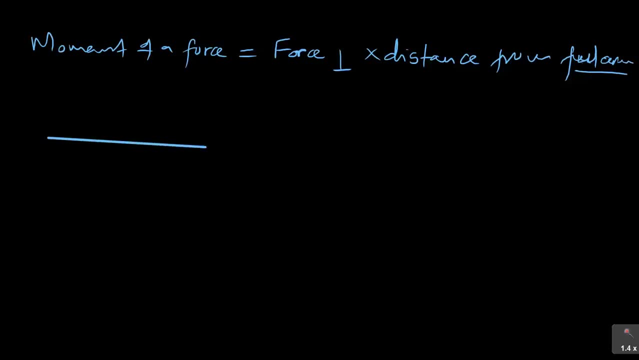 Suppose I have a beam. a beam is like if I have got my beam, like that usually they say, they will say it is light. a light beam meaning it does not weigh much. So this beam, it will have some pivot, which is the fulcrum. 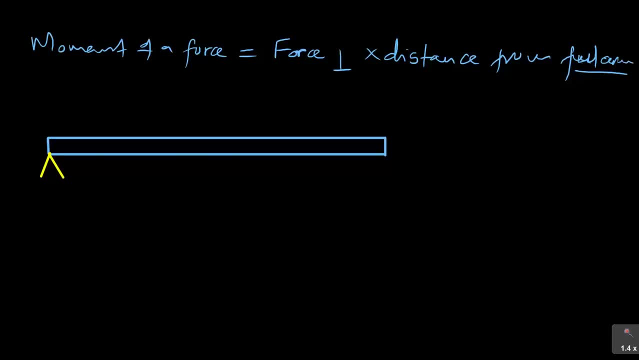 That is what we mean when we are talking about the fulcrum, So this beam will have a pivot where it is supported. So this is the support. and when we are now talking about the distance from the pivot, so we are saying we have this particular beam and the distance of this beam I will 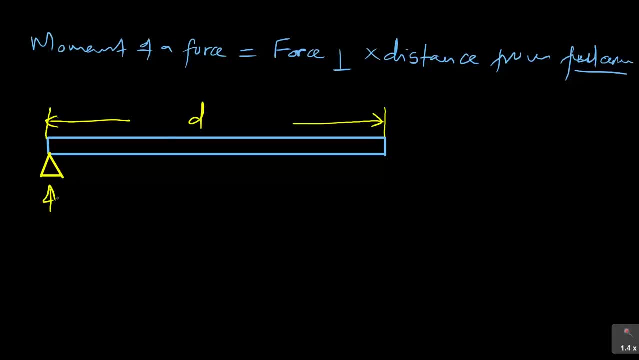 call it d. this is the distance from this point, which is the fulcrum. Okay, So this is the moment by the fulcrum, or the support, And then sometimes we say the pivot, that is where this beam is supported. Now you can see that this beam, the force, is directed upwards. 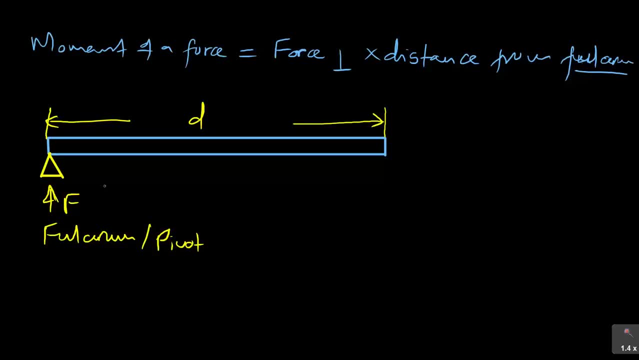 And because of that, that's why we say perpendicular force times distance. So when we are talking about the moment of a force, we are saying it is force times the distance. So you can see where the force is. The force is being applied at this point. 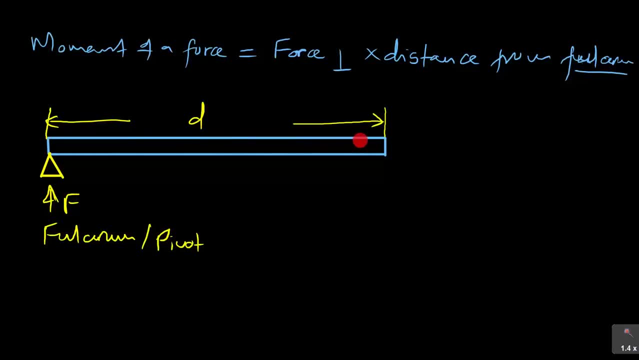 So this is where the force is applied And the distance, this is the distance that we are referring to. So when you are saying force times, distance from the fulcrum, if you know the distance that is from this point, that is where the distance is. that up to that point, and you 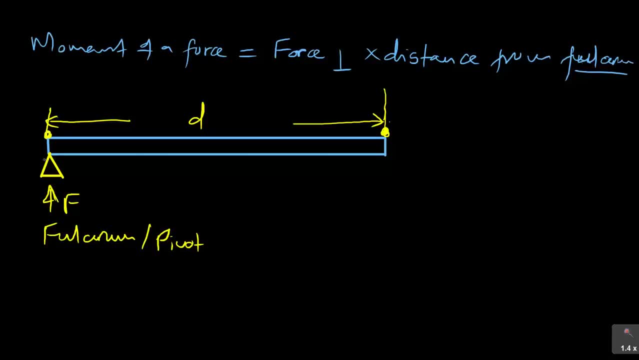 multiply by the force that is applied due to- at this point, due to the support. we call that a moment of a force. But now Another thing that I want to emphasize: If you look at this beam, if you let go of this beam, you will see that this beam is 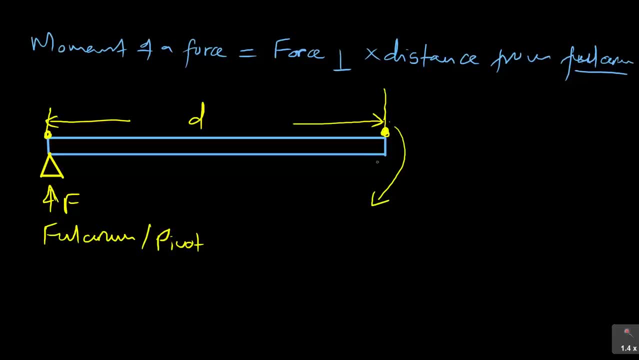 going to start falling this direction because there is no support here. So it will start falling this direction and you can see the direction that it is taking. It is taking this kind of direction and we call that clockwise, Because we'll be taking clockwise moments and anti-clockwise moments. 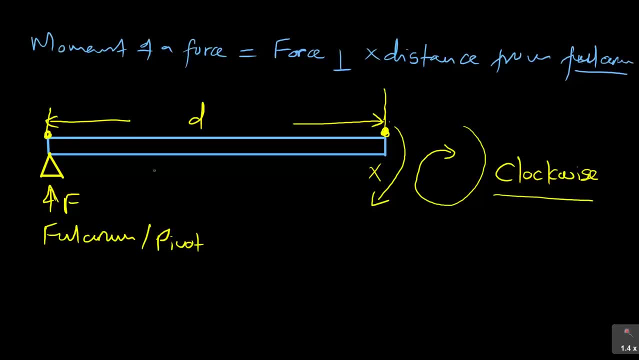 So when we're talking about clockwise, we are saying, If I remove or if I don't have a support at this point, what will happen? if only the support is at this point, You will see that the beam will go downwards here, And when it is going downwards we call that a rotation, that it will take and that kind. 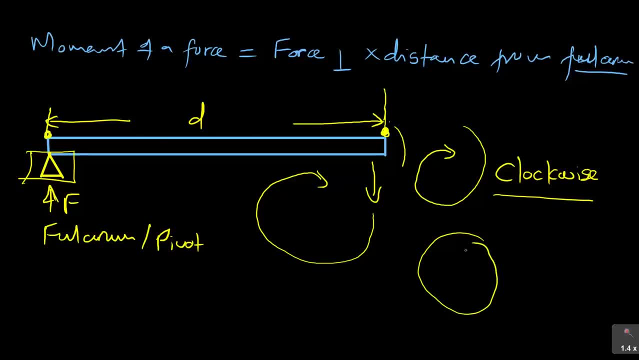 of a rotation. You can see that if you have a clock and you have your 12,, you have your 6,, you have your 3, and you have your 9. And you have your 9.. And if this is the clock, remember the clock is moving in this direction. 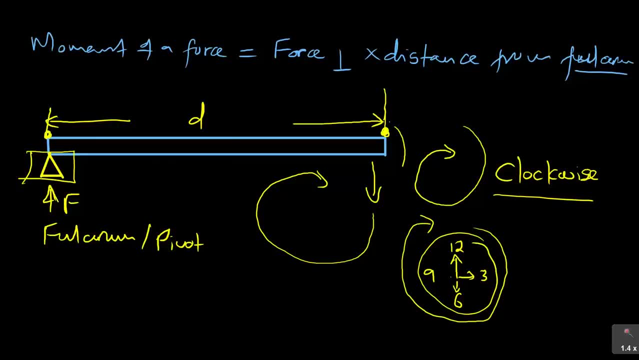 So from 12 to 3 to 6 to 9.. So you see, that is how the clock is moving. So that's what we mean when we say clockwise direction. Now, if I do the opposite part now- And by the opposite part is if I remove the support at this end- 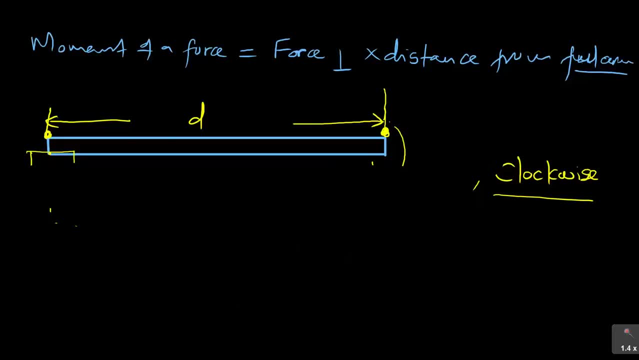 And I put the support On the other side. let me leave that for now, If I remove the support And instead I put my support now, at this point. So this is now my support. Now the question is, what will happen to this beam. 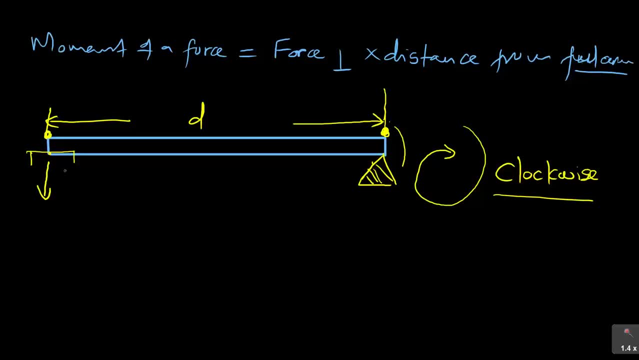 This beam will start moving in this direction, meaning it will move more like in that kind of rotation. Again back to our clock. If I have my clock, 12.. And I have my 6,, my 3, and my 9.. 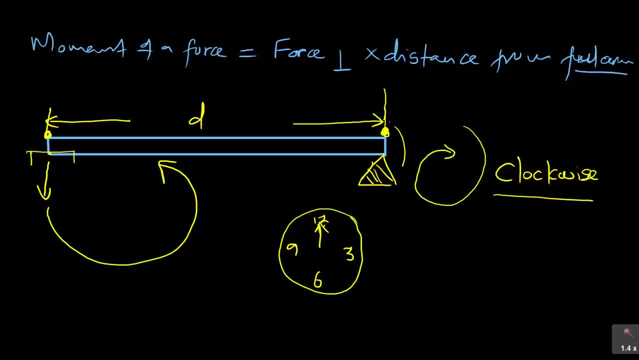 So now you see that the beam is changing movement. It is starting from 12,, going to 9,, going to 6,, going to 3.. So the movement now of the beam is in this direction. as you can see The direction that it is moving, 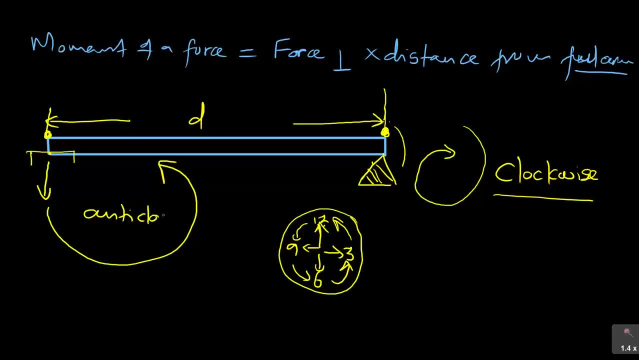 So we call this anti-clockwise, Okay, So this is anti-clockwise rotation. So whenever we are talking about clockwise and anti-clockwise, remember we are looking at what the beam or how the beam is going to behave if we remove a support at that point. 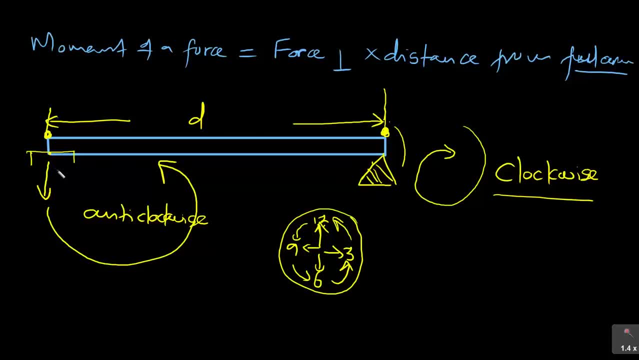 and consider the support on the other side, For example. if the support is removed from this point and only the support is on the other side, this beam definitely will move down, And when it is moving down, You look at the distance that it is doing. 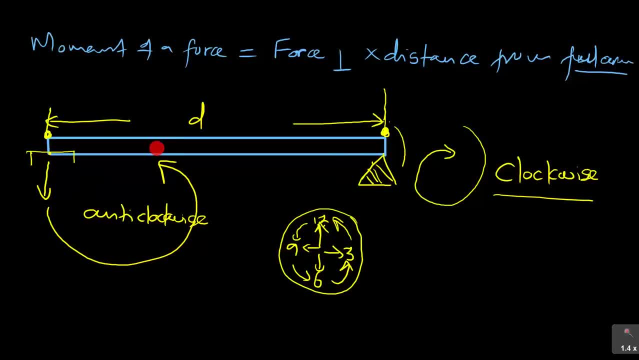 We are saying that movement is an anti-clockwise movement. The opposite is true. If you put the beam on the other side, if you put the beam on the other side like that and then you remove that support, this beam will start moving down here and that movement 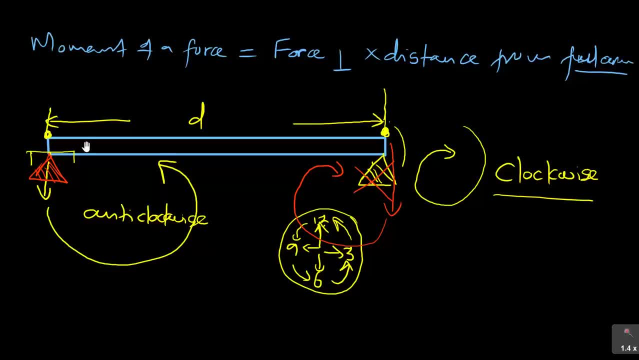 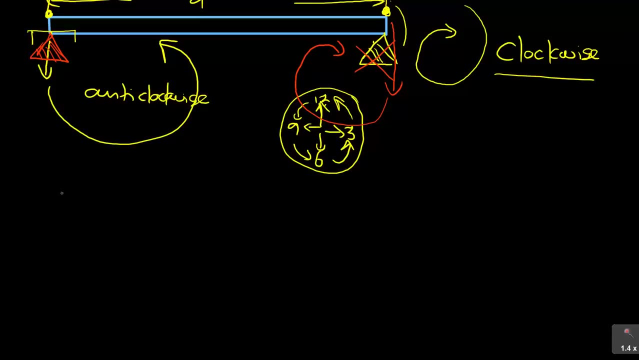 is called now clockwise, So in our calculations, Or in our calculations, Okay. So in this method, we are going to be looking at, in this case, the sum of moments. So another thing that I'm bringing in is the sum. 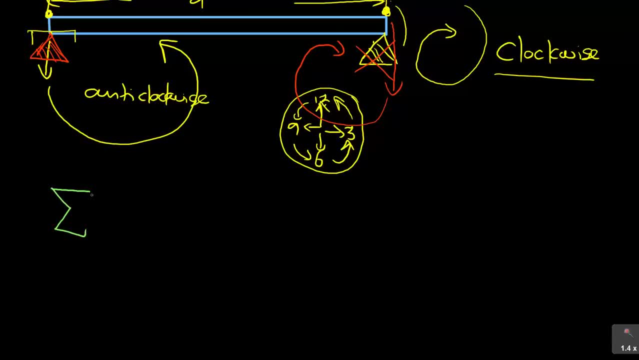 So if I'm saying sum of moments or sum of clockwise moments, So it'll be, this sign means sum of. That's what this sign means. So if I say something like this And then I do a rotation like this, I'm saying: this is sum of clockwise moments, right. 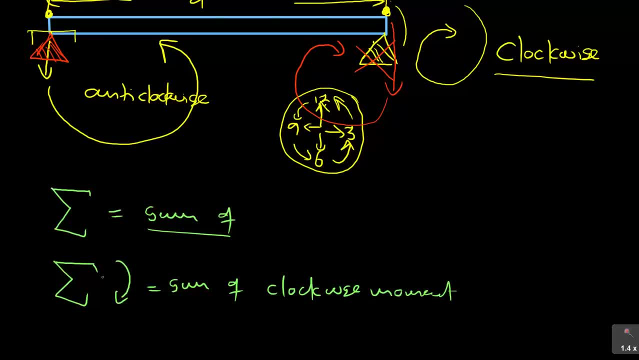 And then if I do the other one, whereby I'm saying like this and then I'm doing that, I'm saying sum of anti-clockwise moments. So remember, Okay, So remember, such is very important, so that whenever we're working, you'll be able to. 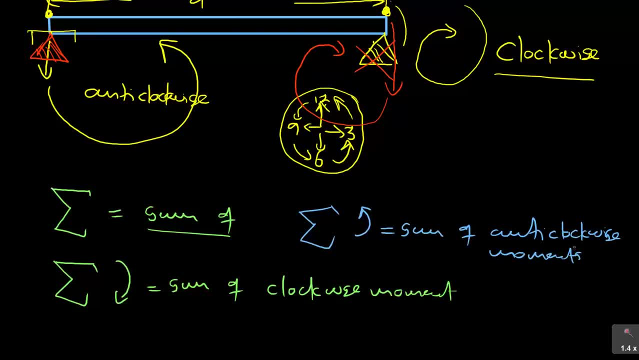 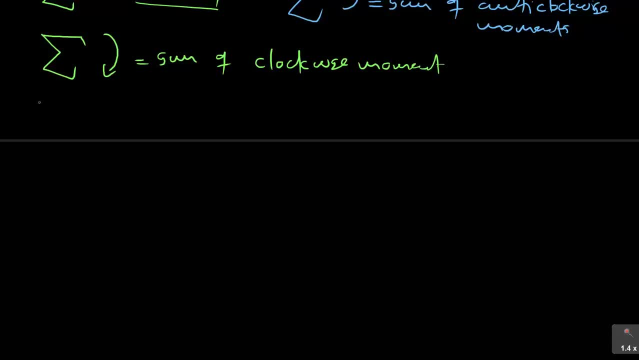 remember why or what is what. So this is what it means. And then, if you look at this, we are now coming to the law of moments. And how do you state the law of moments? The law of moments say, sum of clockwise moments is equal to sum of anti-clockwise moments. 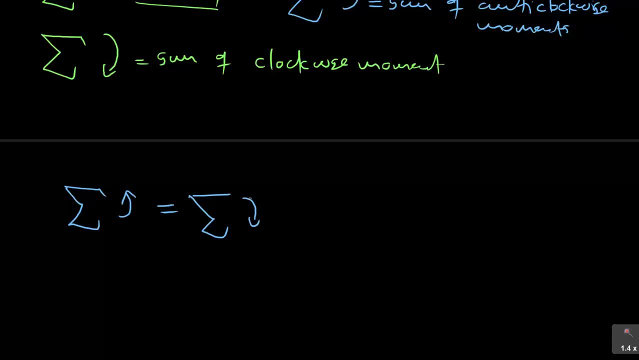 So remember that We are saying: sum of clockwise moments is equal to sum of anti-clockwise moments. That's what we're meaning Now, the last thing that I want to bring to your attention again, so that we finalize this part, Let me again have my beam. 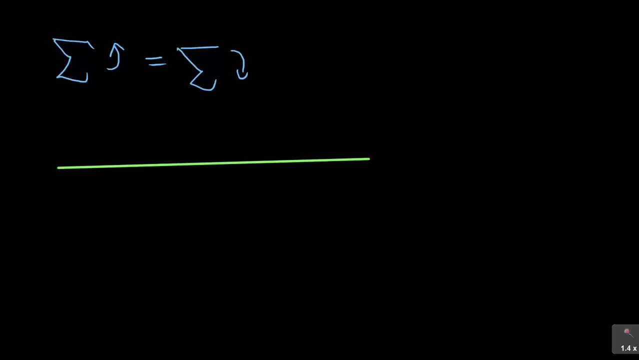 So if I have a beam like this, this is my beam and it's light, it's a light beam. And now if I have forces that are acting on this beam, For example, I can have a force that is acting at this end of the beam. 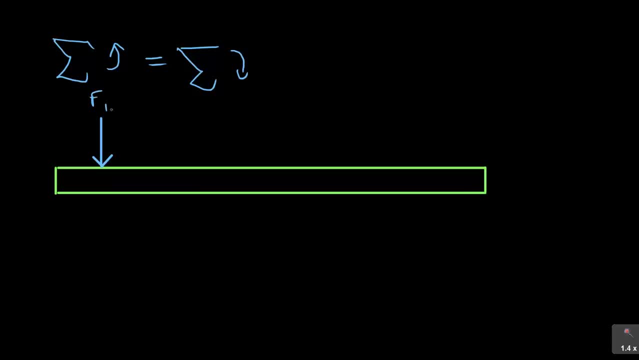 So that force, I'll call it F1.. So you can see when a force is acting like that and I have maybe a support on the other side of the beam. So now this particular force is going to push this beam going down and you can see again. 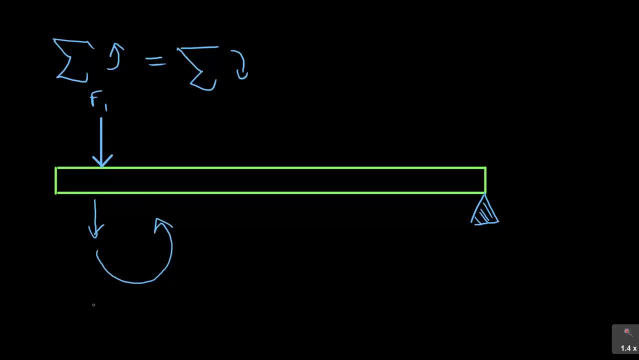 it is anti-clockwise rotation. So that will be a force that will cause the beam to rotate anti-clockwise. Are you seeing that? Now, let's say I have got another support somewhere here. I have my other support on this beam. Now I have a force here. I'll call it my force 2.. 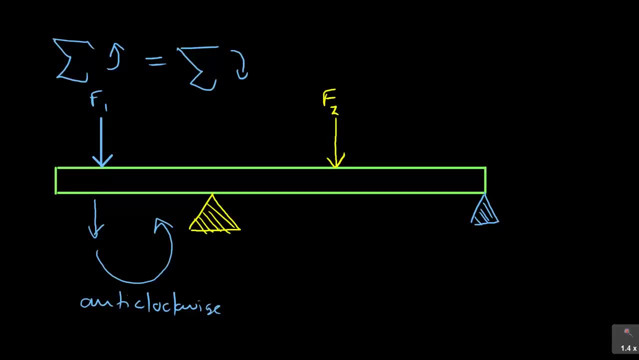 That is acting on this particular beam. And now, if I ask you to say what is the effect of force 2 on this beam, You can see that force 2 is pushing this beam in this direction. You can see that, if this is my line of reference. 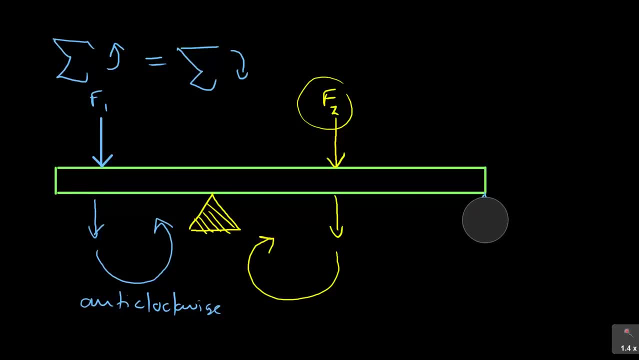 So if I remove this, let me just remove this force, If I remove that. and I ask you, what is the effect of F2 on this beam? That is acting on this particular beam, particular beam, and you are using this as my pivot. this is my pivot, you can see. 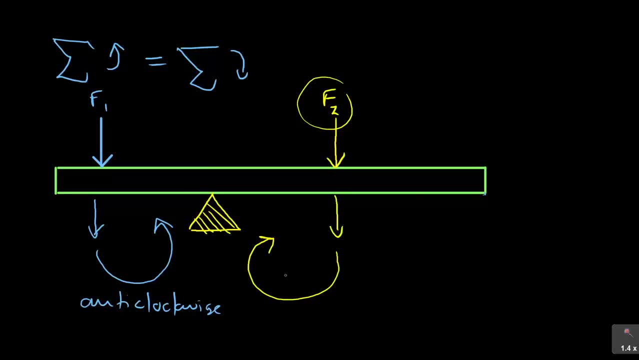 that it is going to push this beam down and we'll call that a clockwise force. so this force will be pushing this beam in a clockwise direction. I hope you are able to say that. so whenever you are talking about moments, about, you need to tell us which support I talking about. so at this stage, I'm using this support and 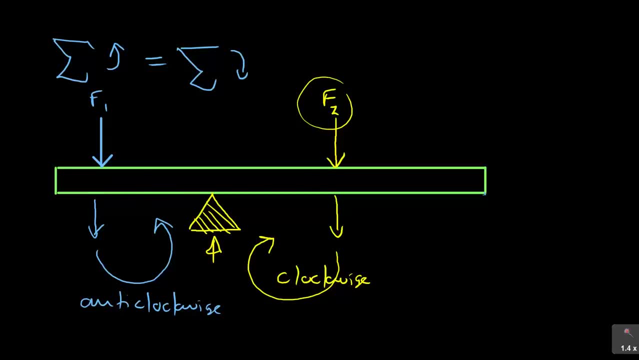 when I'm using this support. you can see that these two forces, f1 and f2, are going to have two effects about the pivot. so the first one is going to push. as you see, it's going to push the beam downwards and rotate it anticlockwise. 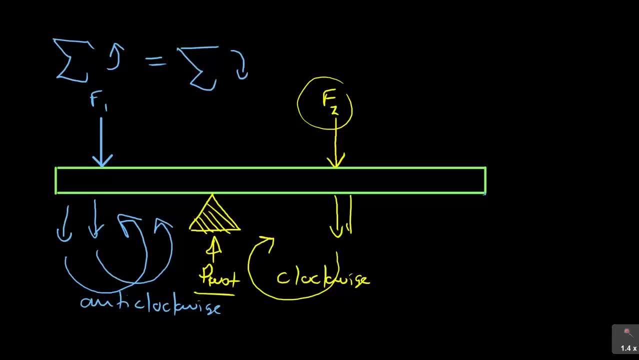 and the second one is going to push the beam also downwards but make it rotate clockwise. so that is very, very important. so whenever you're seeing moments about a pivot, you need to first identify which support are you dealing with. if you are dealing with this support here, if I'm dealing with this, 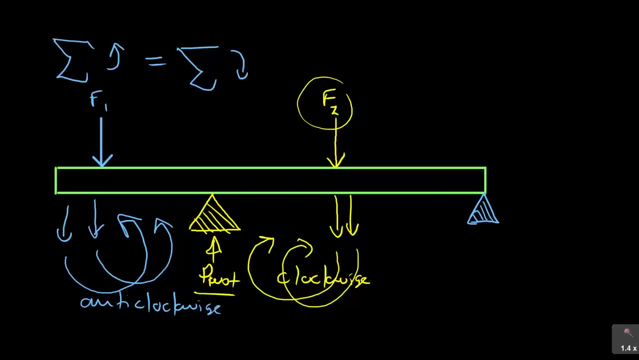 support. what I must do is I need to first ignore this particular support and ask myself what will be the effect of these two forces about this side or about this pivot. so you can see that the first force will push this beam downwards and the rotation is anti-clockwise. so remember. 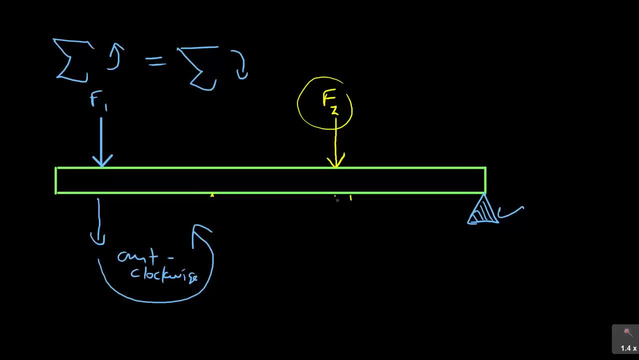 such, and you look at the second force, f2, it will also push the force downward. and when it's pushing downward, the rotation is similar. also here, it is anti-clockwise. so you can see now, these two forces, they've got the same effect. about this end. they will have a similar effect, but when I change them and I put 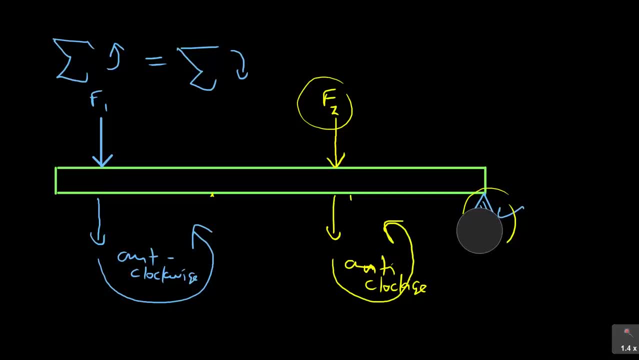 them if you remove that and I change my pivot to say my pivot is now somewhere here. you saw that the same in a different scenario or case, whereby the first force, which is this f1 will have the same anti-clockwise. but if you look now at f2, f2 now has changed in this. 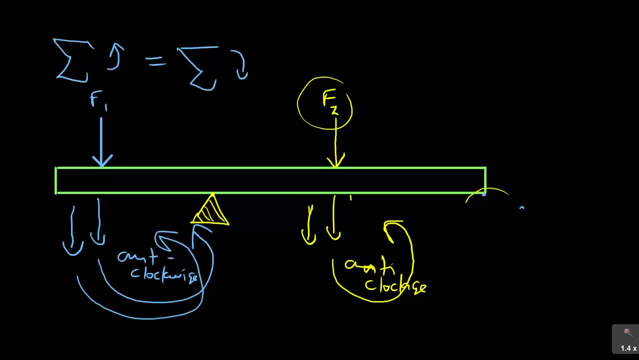 case f2 is making the still going downwards, but it is making this beam to rotate, now in a clockwise rotation. so you need to be careful and you need to be aware where is the beam and what is the effect of that force, whenever that beam is going to be. 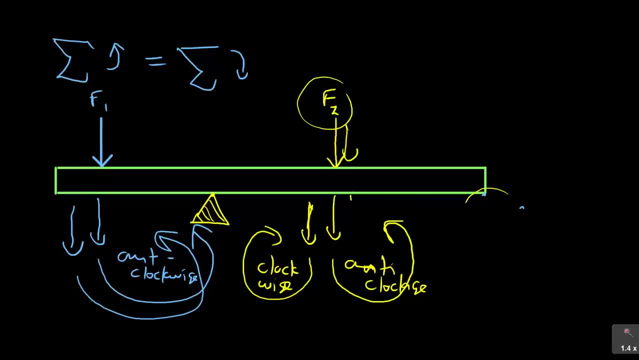 turning. so remember, when I'm pushing this thing down like that, I will cause it to rotate like clockwise along that. so it will be more like I'm saying here, just to show you in a way, just that my diagrams will be good. but I just want to. 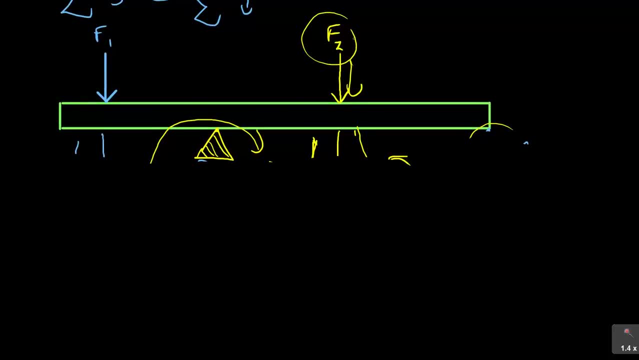 show you what it means about that. for example, f2, f2- if I have my f fulcrum like that. so this effect of f2, you can see what it will do. it will keep pressing down. so this is my f2, so you see where it's rotating. so I can. 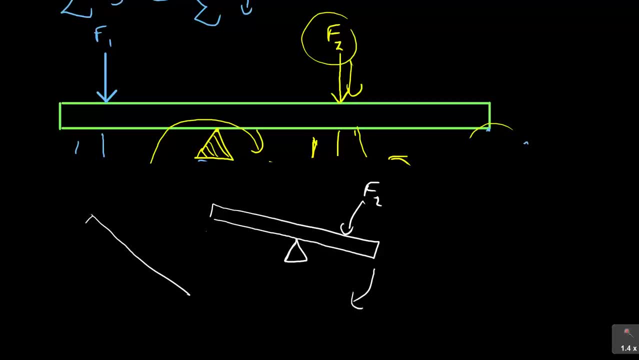 continue drawing it now further. that is my f2. so you see what it keeps doing. that's my f2. and then that's what it's doing is making this beam to rotate. and now, if you look at f1, what it does, f1, in a way, is doing the opposite. so f1 is 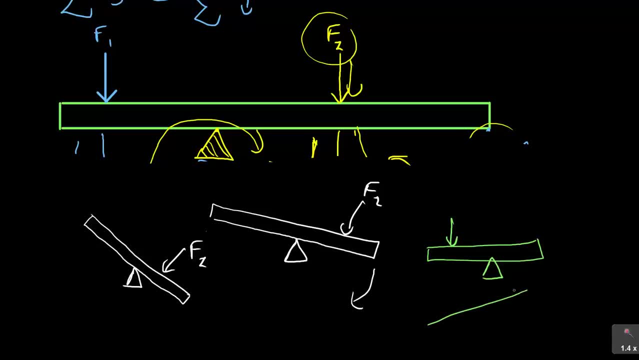 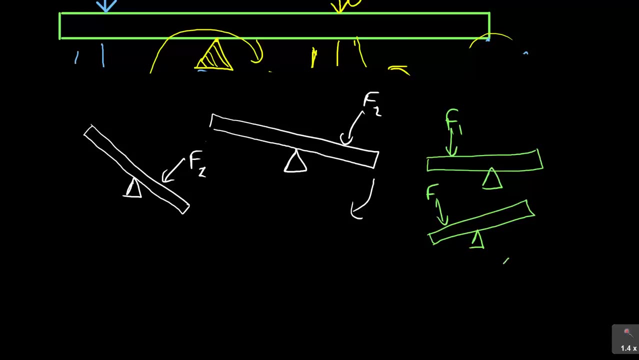 pushing this direction. after some time you will have f1- this is f1- pushing in that direction. so again, if f1 continues, you see something of this nature like that. so you have got now f1. so now, if you look at the direction, you can see that. 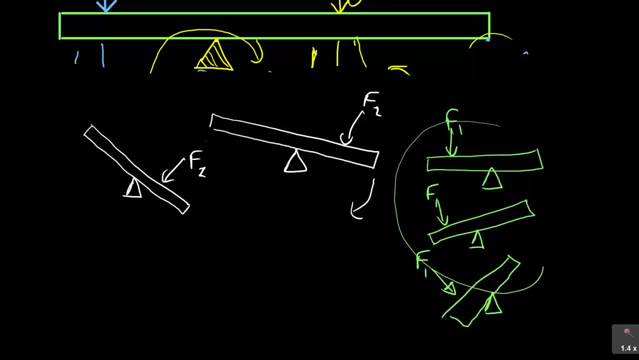 this direction is an anti-clockwise direction. that is happening and if you look at f2- f2- the direction is clockwise direction. so those are the basics that I wanted to bring to you so that, whenever we're looking at calculations, you will be able to understand what we are dealing. now let us look at. 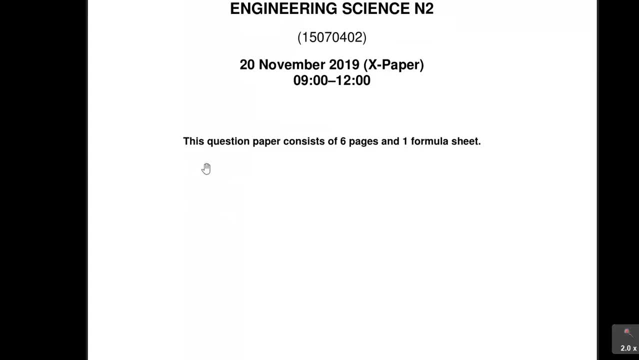 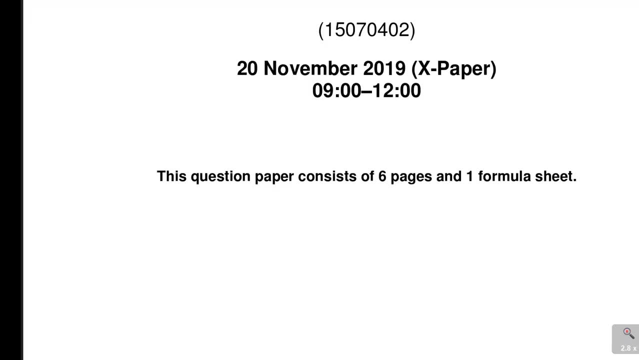 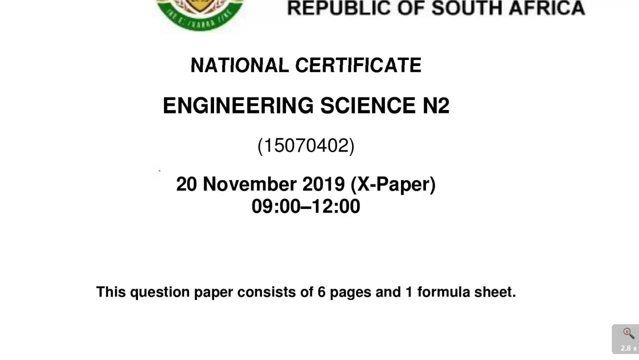 a few examples. as I was saying, this is a question that was written in November 2019 and in this question, as you see, it was a November 2019 question. that's what I'm bringing to you guys. I bring you practical questions that you can even. 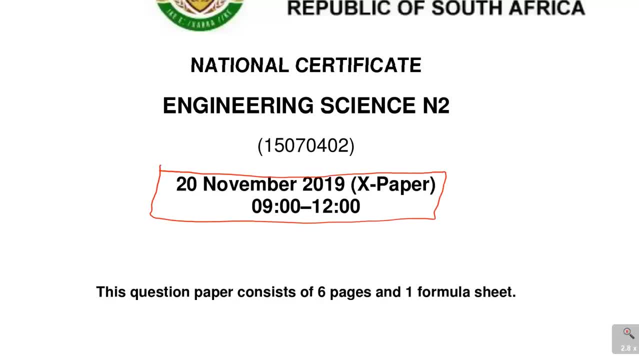 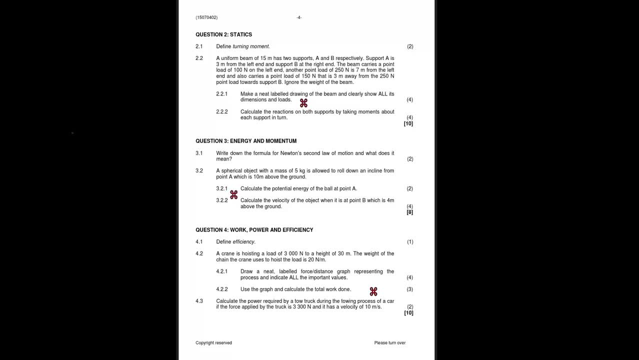 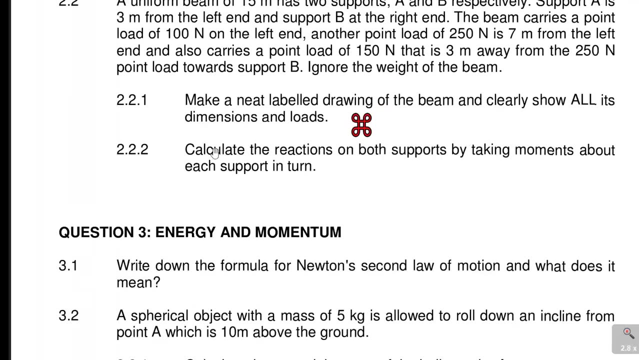 use for your exams. so this is November 2019 and this question I'm only focusing on a force, which is question number two, and question number two is statics. so if you look at your paper, usually it's arranged in that format. question two mainly talks. 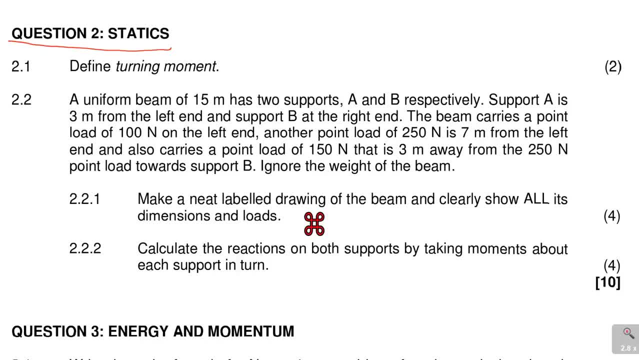 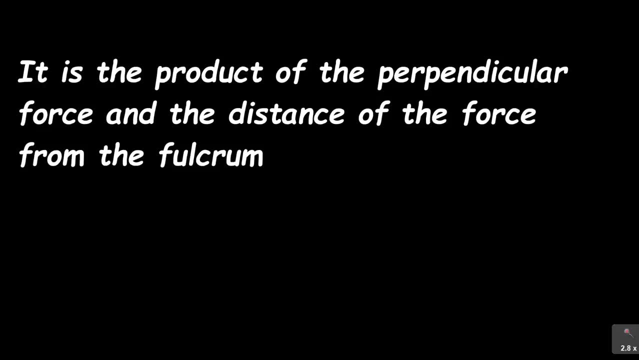 about statics. so if you look at this question, question number two, and then the first part, it's statics. it says, question two, point one: define turning moment. so you need to know the definition of a turning moment. so I'm not going to write that one, but I've already have it. it says we did talk. 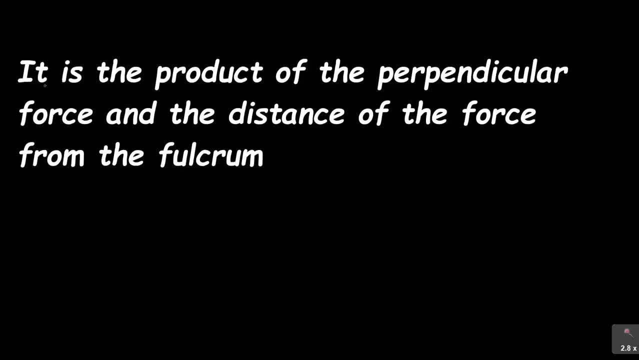 about it to say: how do you calculate? that's what it means. how do you calculate the moment or the turning moment of a force? we are saying it is the product. you can see that. we are saying it is the product of the perpendicular force and the distance of the force from the fulcrum. that is the first part that we 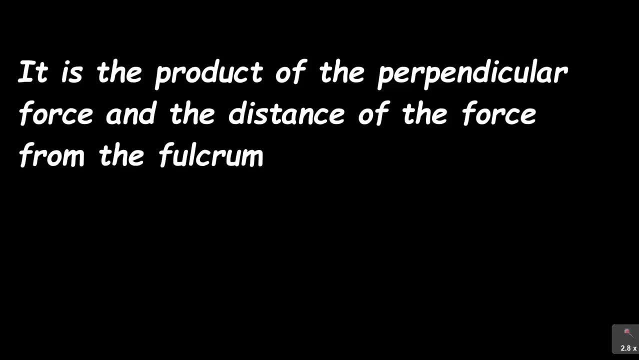 looked at to say whenever you are dealing with this moment of a force, we are saying it is the product, so moment is equal to the product of the force times. we are saying that force is the perpendicular force times, the distance from the fulcrum, and we did look at it to say you are having your 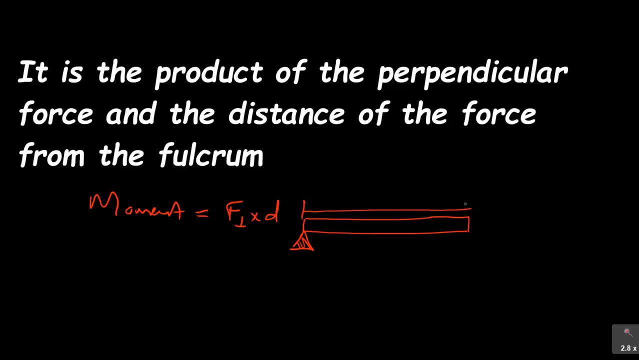 fulcrum there and then you have got your distance here. so now that force F is, that is the force and distance, is that? so if you multiply f times d, we are talking about as the moment, and the units is newton dot meter. so these are the units. remember, f is a newton, distance is: 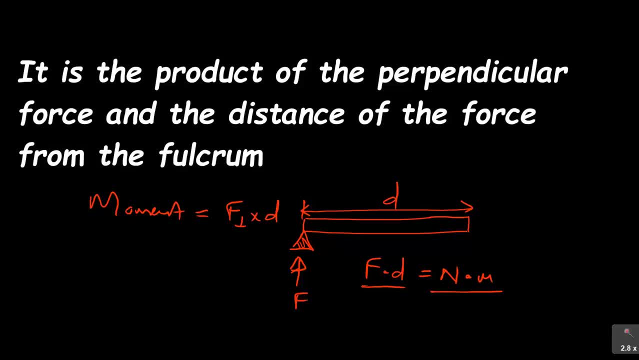 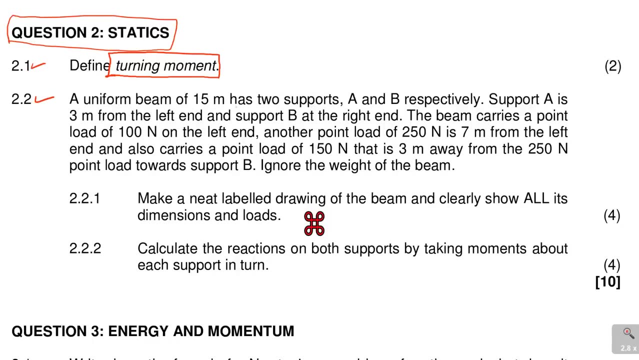 measured in meters. so this is the units of that particular force. so it is the product of the perpendicular force and the distance of the force from the fulcrum. so that is that part of the definition. and then 2.2. it says a uniform beam of 15 meters has two supports, a and b respectively. 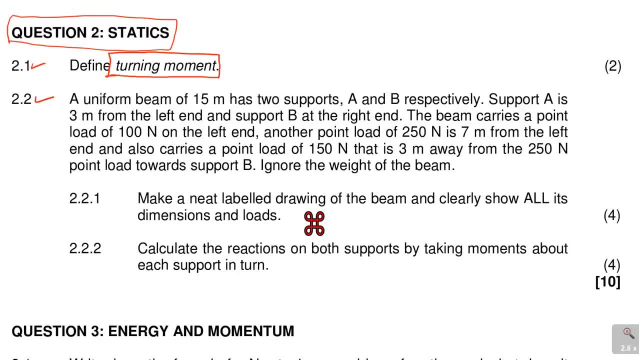 support a is three meters from the left end and support b and support b at the right end. the beam carries a point lot of 100 newtons on the left end. another point lot of 250 newtons is seven meters from the left end and also carries a point lot of. 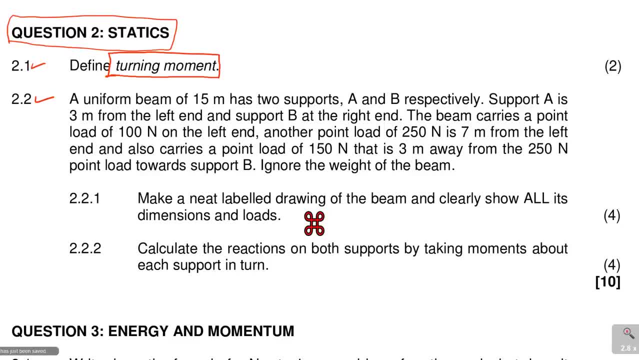 150 newtons, that is, three meters away from the 250 point load towards support b, ignore the weight of the beam. so it's quite a mouthful of um statements there, but we're going to analyze each and every statement there. then it says: make a neat labeled drawing of the beam. 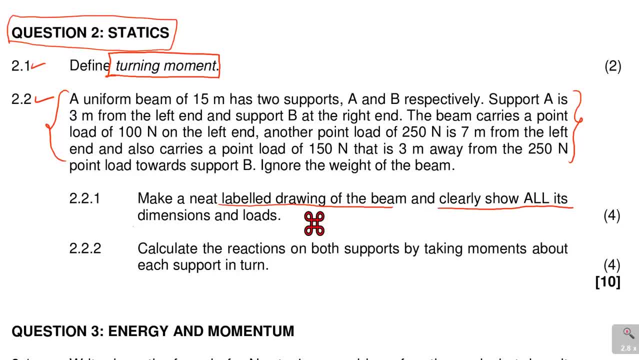 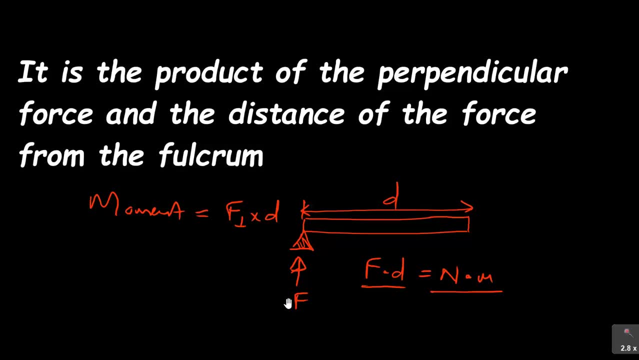 and then they're saying: clearly show all its dimensions and lots, and then they want to give to gb4 marks for that. so if you're going to make a neat level sketch of that, let's do that, um, but we need to ensure that where we get all the four marks that are given there. so let's look at what they're. 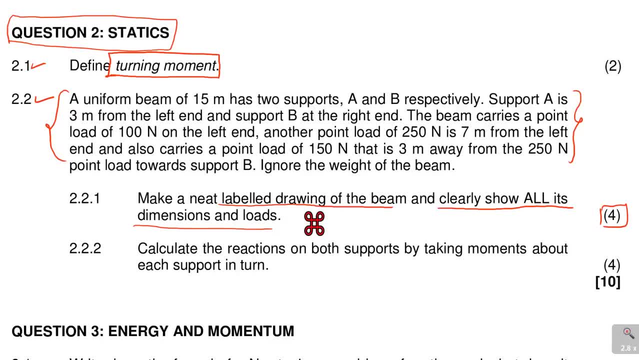 talking about one statement at a time. so you are given a uniform beam meaning: uh, your, your, the way you're drawing your beam, don't make it uneven, so it must be uniform. a uniform beam which is 15 meters. that is key. take that it's 15 meters, has supports, a and b respectively. okay, so you start. 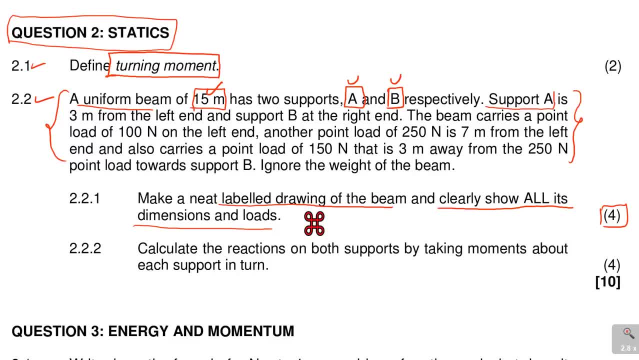 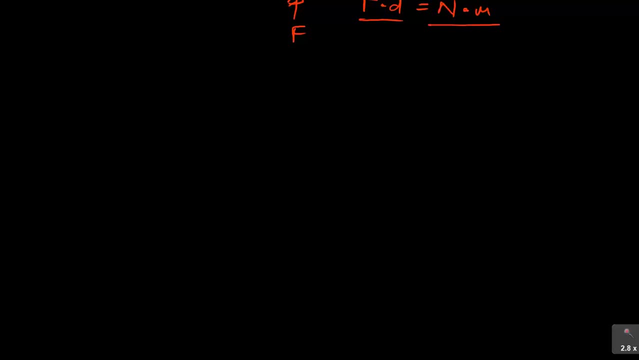 with a and then you follow by b. then they talk about support a. now say: support a is three meters from the left. so it's three meters from the left, so that is also key from the left end. so we start looking at that. i can now draw that statement. first, let's have the first. 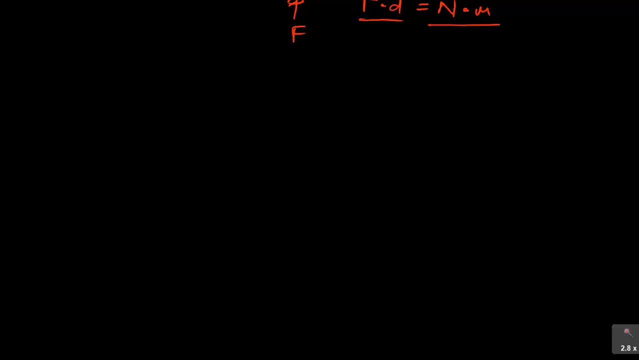 part of the statement. we are dealing with a uniform beam, so i'm going to have my uniform beam like that and so uniform. as i said, make sure that in a way it is. i made more parallel on the ends, so suppose you can do actually better than me. so this is, uh, my uniform beam and we are. 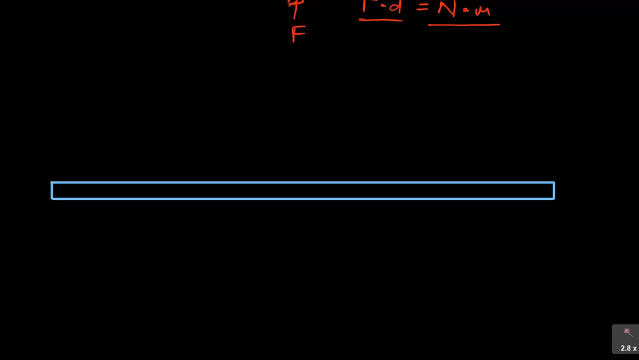 saying this uniform beam is supported at point a. i think you saw that they say there is a support at the end. so we have got two directions, the left and the right, and this is my left side. so this particular beam here there is a support here. so that is the first support and they call that support. it is support a, and then 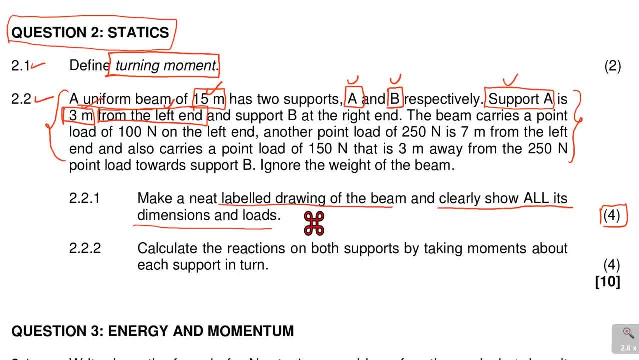 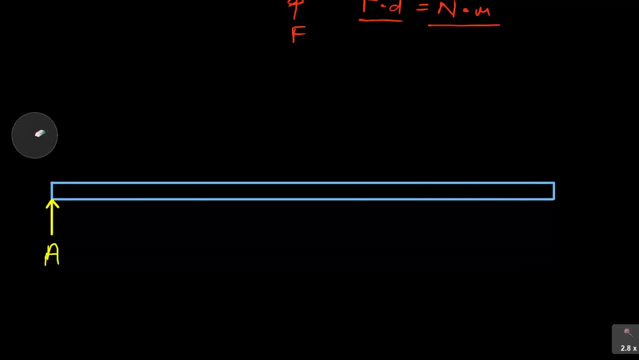 they say: let me just read again. if i'm doing right, they're saying support a is three meters from the left end. actually, this is wrong. i need to draw support a three meters from the left end. so this is the part. this is not three meters from the left end. so now what i need to do. 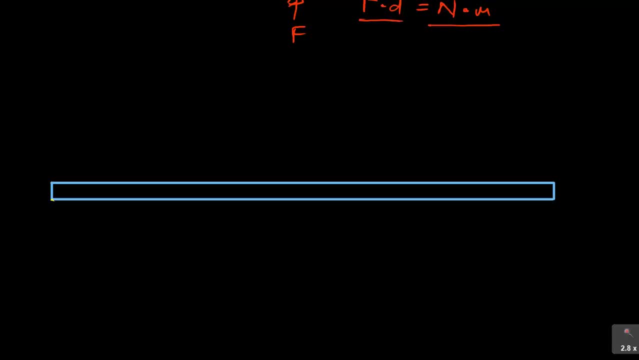 i need to start marking my beam to say the distance from this point, maybe to remember this is a sketch. you might not be very accurate, but, um, you can just have an idea. for example, from here to here. you know that i can just do it a sketch on top like that, then i'll i'll erase it just to have an idea, because the final diagram 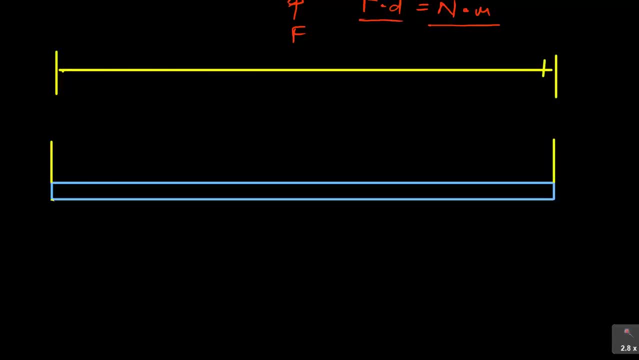 you don't want it to be clumsy, so this is um the length of the beam. they're saying this beam is 15 meters, remember. so you know i'm dealing with the 15 meter beam, so i will erase this part later, but just to have an idea, what is what? so, and also my 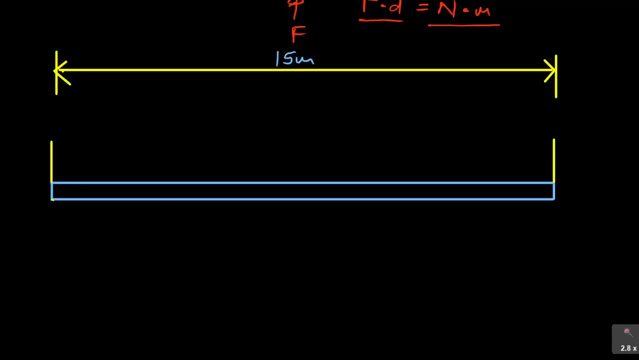 measurements, you can use your ruler, but it's not necessary. as i say it in this case, it's just a sketch, just that. you need to be a bit more accurate. so if i can now deal with that as roughly my center, so it will be in this case my 7.5 here and then the center of 7.5 is there. 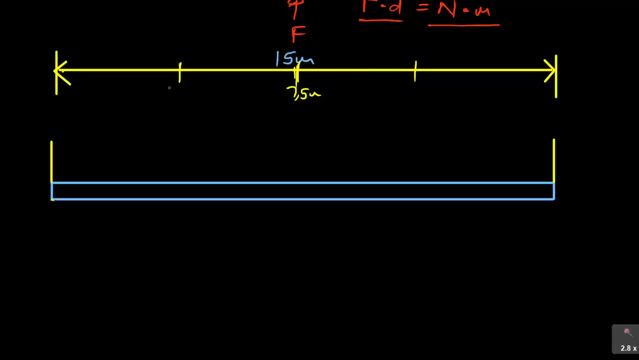 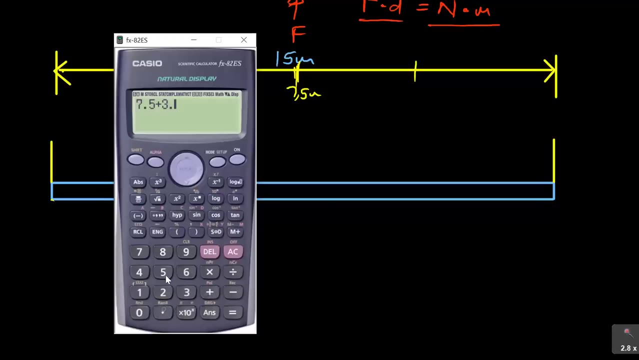 and the center of 7.5 is there. so here you expect it to be around 3.5. and then here you add 7.5 plus 3.5. um, i think it will be 7.5 plus 3.5. it gives me 11, so you expect this part to be. 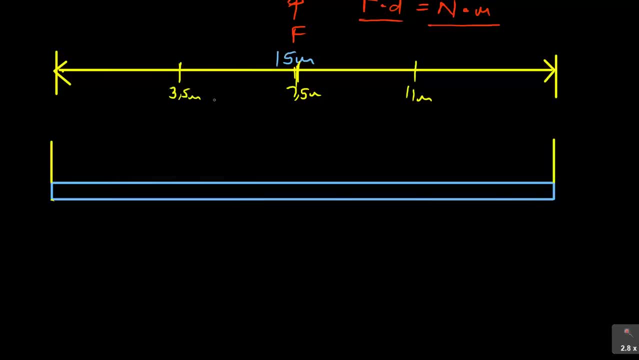 11 meters. all right, so this is just a rough kind of a thing. so they say that, um, when you start dividing it into um, what they say, it is three meters, just in a way. so you think, or you put maybe three meters somewhere there, this is three meters. so if i now come to my labeling, you can see that i can make that now be. 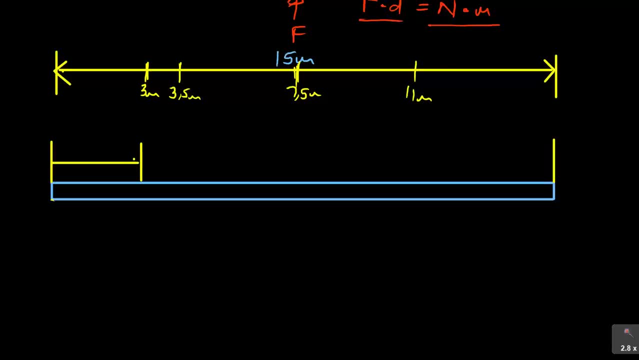 equal to three meters. so if i do that, and i do that, that's the first part that i'm given. so that is three meters. so that is three meters. so that is three meters from the left. remember, this is my left side in here. all right, this is my left and this is my right. i'm just taking it a bit slower so that you. 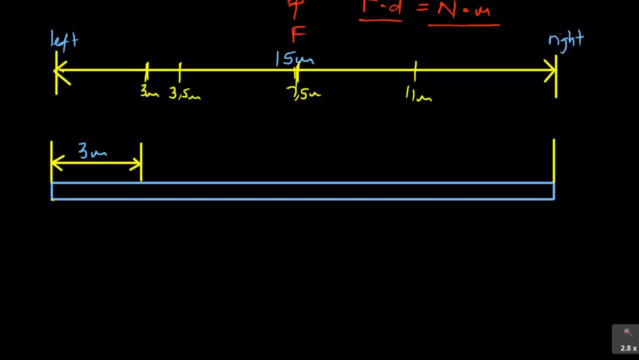 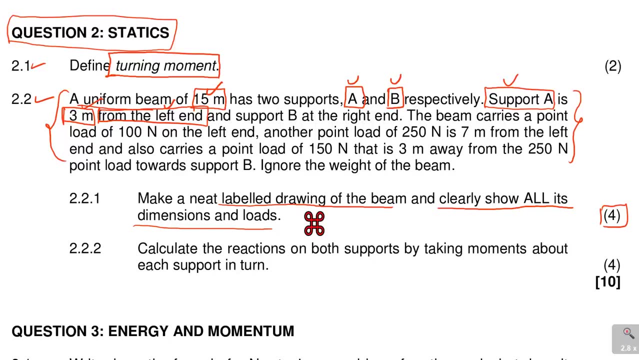 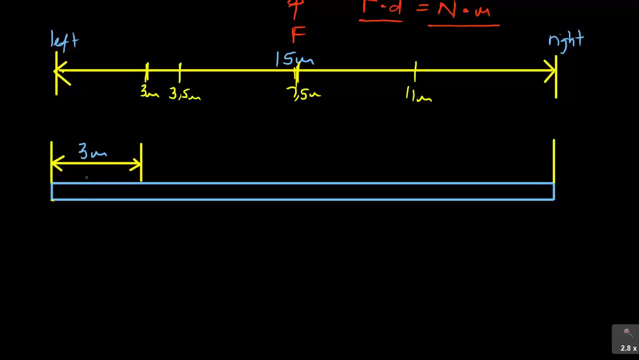 can just have an idea what we're dealing with. so they are saying here: um, a uniform beam, 15 meters, has two supports, a and b respectively. support a is three meters from the left end, so that is what they were saying here. so this is my left end. it is three meters and here 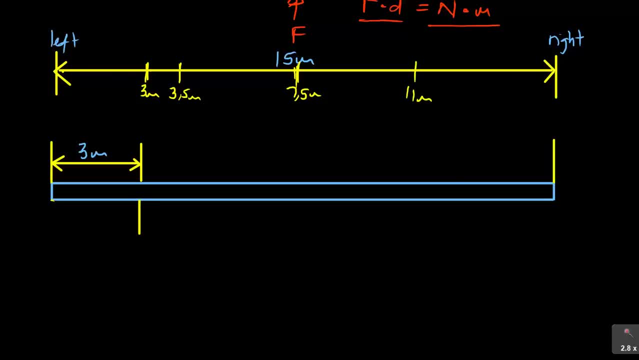 expect me to have support a just above that three meters. so that is, uh, my support a there. you see that. so that's what i'm having. and then let's find out where is support b. and then they are saying support b. and then let's find out where is the support b. here they are saying support b. 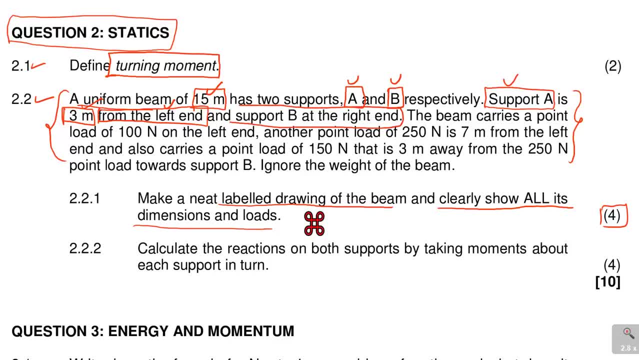 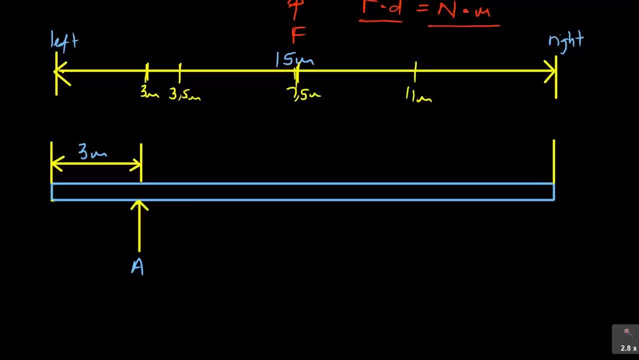 support b is at the right end, so we need that support b at the right end. so if i come to the right end also- and this is my right, and the right end is that part there- that is where i find my support b. so that's what i'm having. so this is that at the moment. then continue. then they are. 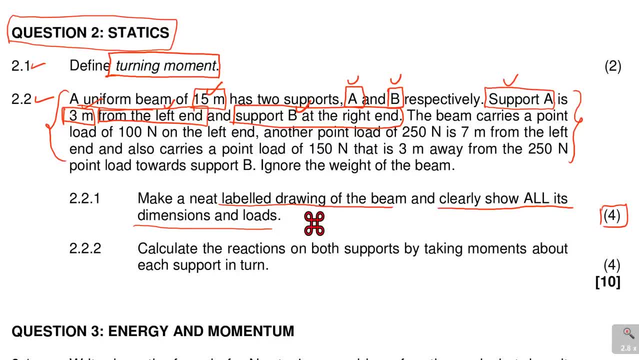 saying the beam carries a point load of 100 newtons from the left end. there is another statement: a point load of 100 newtons from the left end. so the beam carries a point load of 100 newtons on, not from on the left end. that is very important. 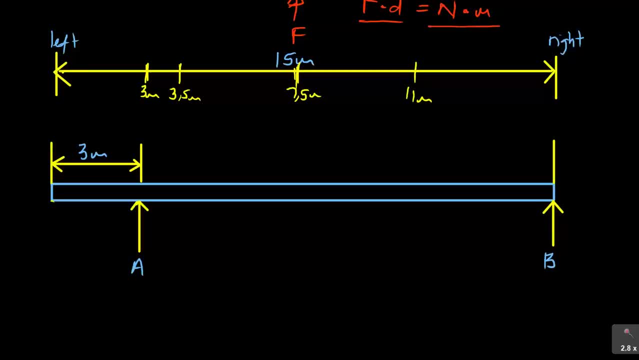 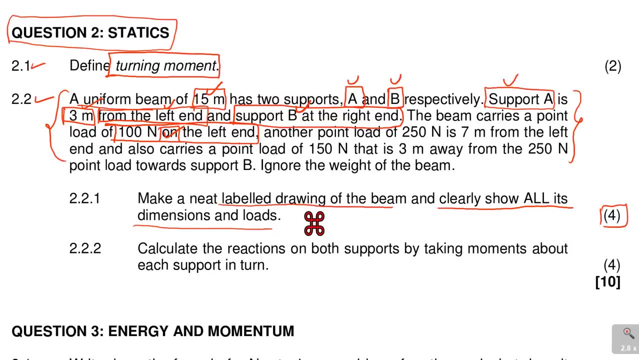 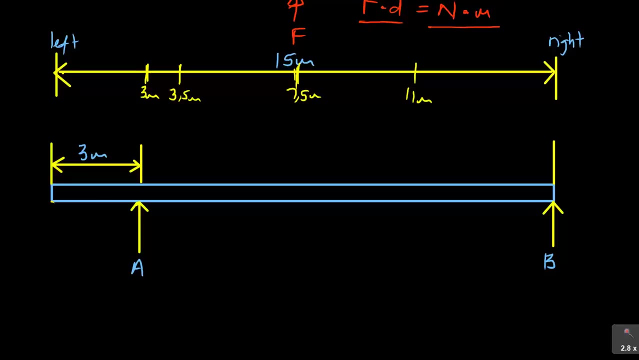 it's on the left, so which means you go to the left, just like they said here, the beam support b at the right end, so also on the left end, just like in b. so you come to your beam here on the left end. you have um, sorry about that, a point load um. 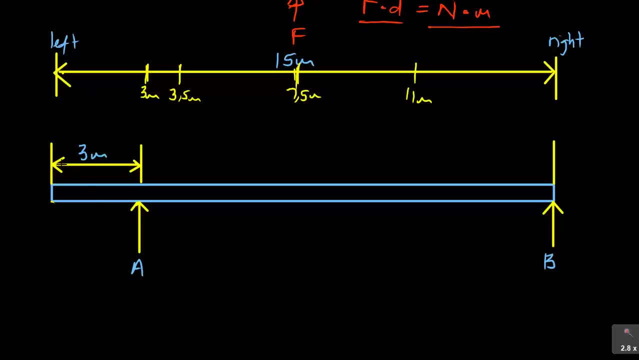 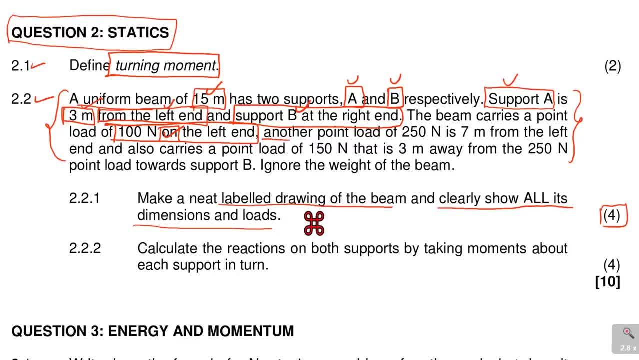 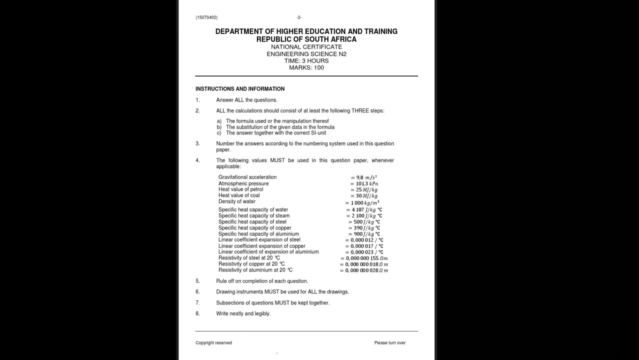 first part and they are saying another point load of 250 newtons. so there is another point load of 250 newtons is 7 meters from the left end. so there is another point load of 250 which is 7 meters from the left end. so we come from remember our reference point here is from the left end. 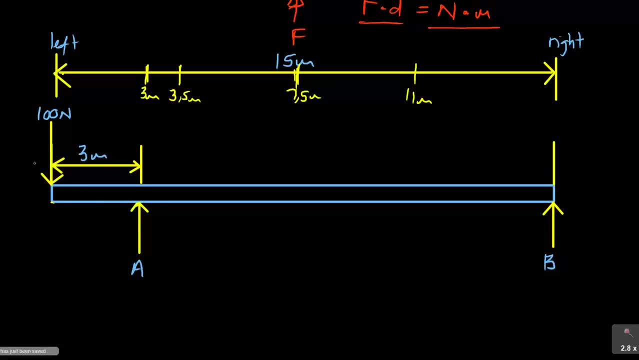 so we come from. remember our reference point here is from the left end. so i am from the left, which is this direction, and i need to find seven meters, which is somewhere there. so this is where i get my seven meters. so i will have my line to say at this point here. 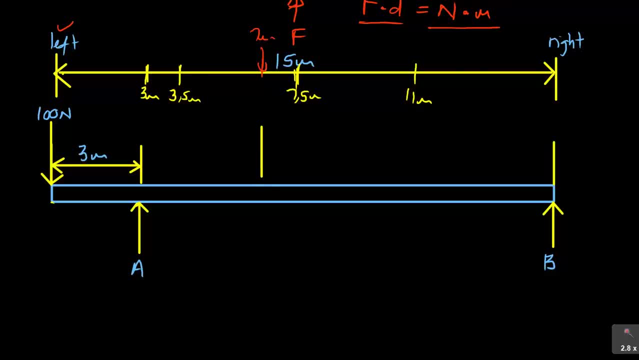 there is um a point lot somewhere there. there is my point lot, and they say: that was 250 newtons. you see that. and then in 250 newton, newtons. now, if this is now seven meters, now you don't write seven meters, what you do, you come here and say: already i have my three meters here. so for me to move from that. 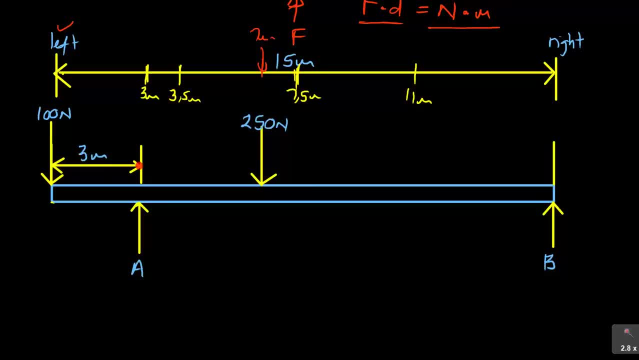 point to that point when i already have my three meters. so what is the distance from here to here? it will be four, so that you say four plus three, it will give us that distance of seven. you see that? so i need this distance here to be seven, like this. i need, uh, this part. it must be seven meters here. 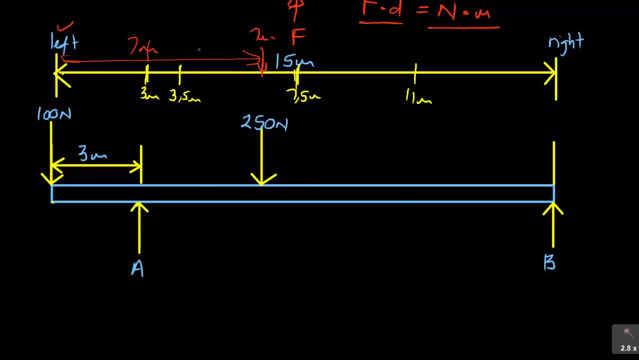 so for it to be seven meters, it means from here to here it has to be four meters, and from there to there it has to be three meters. so when i use that, i'm going then to have that, say that and then, as i said, you write that as your three meters, i mean your four meters. 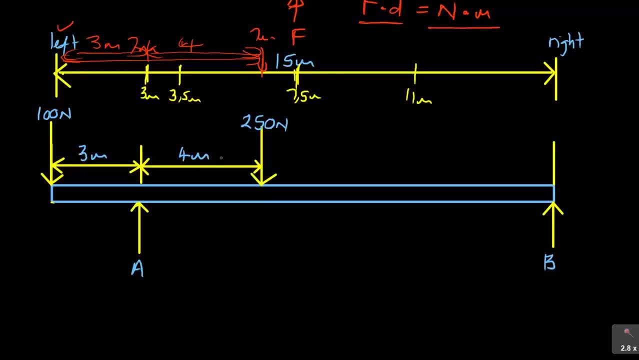 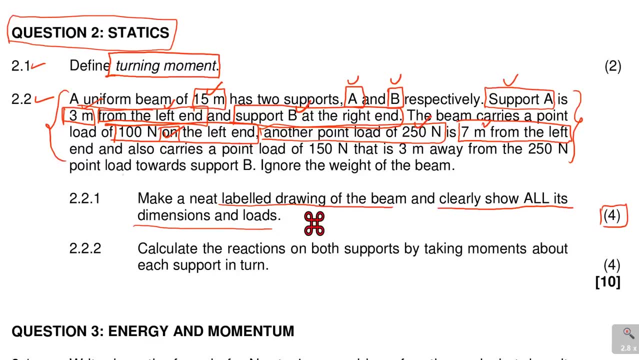 so that is how this thing or this beam- slowly you're creating that beam. then the next one says um, the statement continues. it says uh, from the left end and also carries a point load of 150 newtons, three meters. okay, there is 150 newtons. there is three meters away from the 250 newtons. 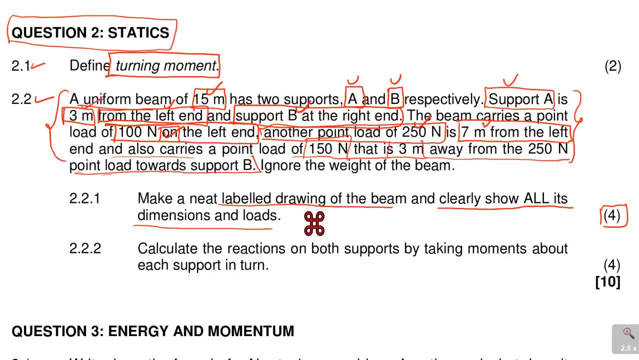 point load towards support b. so you see what they're saying. now they're saying: you have another one, which is 150 newtons. let me just clear this. so you have another load of 150 newtons. that is three meters away from 250 newtons. 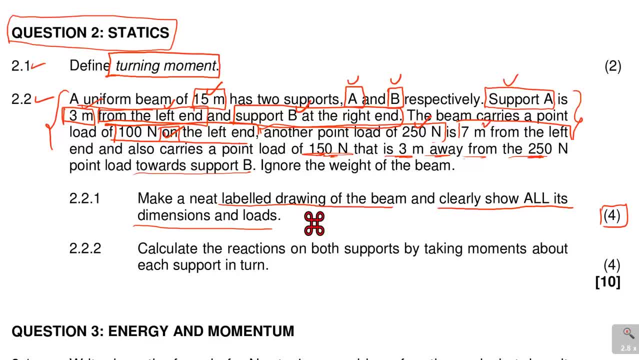 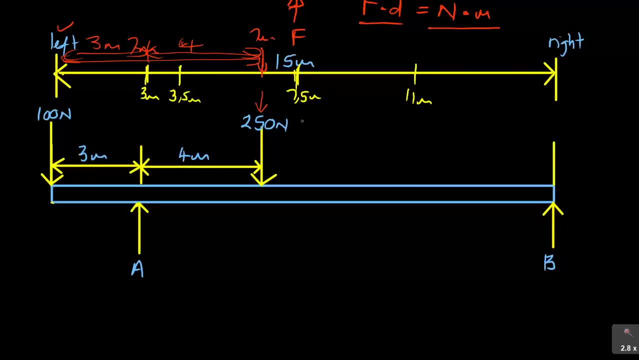 uh, point load towards support b. so you go to the 250 newtons go three meters away in the direction of support b. so what they're saying here is: we have got our 250 here now. now to what support b. this is the direction, but you must move. 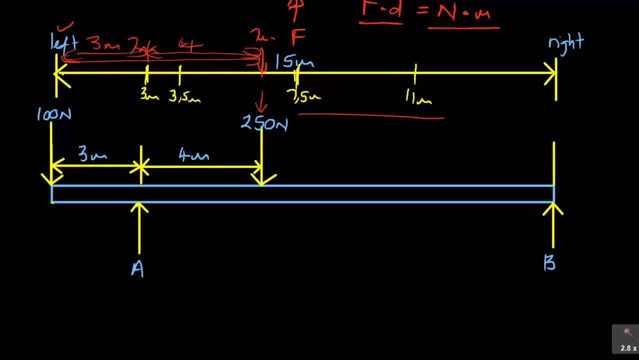 three meters. that's what they're saying. so if we can do that, we are going to have, at this stage, a distance if you are saying three meters from so i'm going to also have a distance that was similar to that size of a distance, because it is the one that 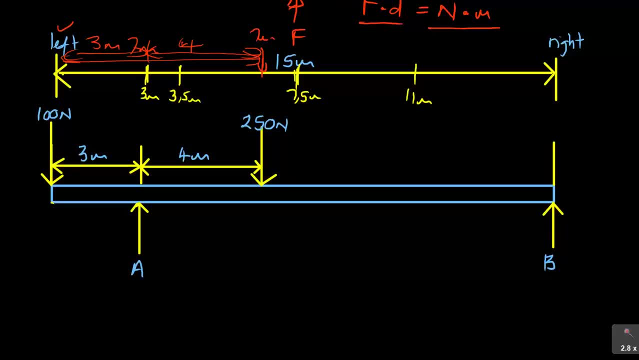 is three meters, So I'm going to now mark my beam with almost an equal kind of a force here like that, And they say that force was 150 newtons. Right, so I'm just as I said, I'm taking it slower. 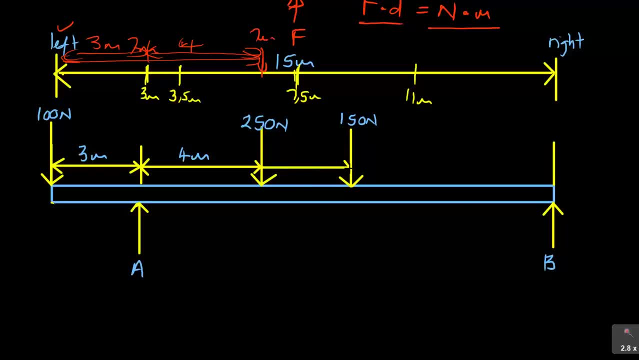 But next time I will be doing this much quicker, with the assumption that the first question was making no sense. So they're saying this is 3 meters away. So it's 3 meters away from the 250 towards support beam. I'm saying that. 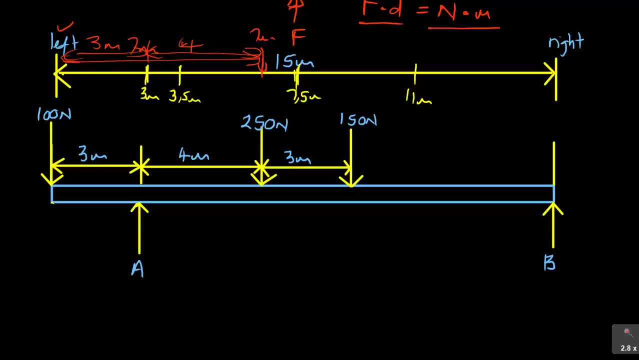 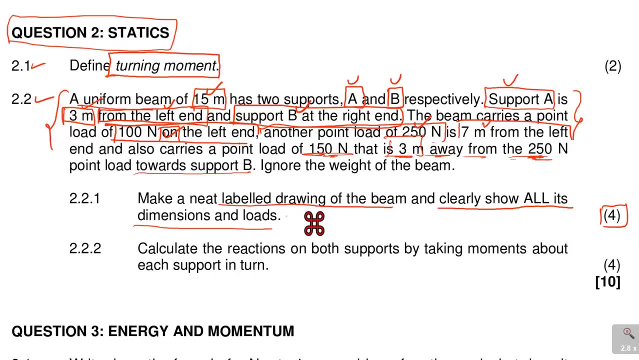 So that is why I was doing what I was doing. So now, looking at this last statement, and then says: ignore the weight of the beam, Make a knit label sketch clearly showing all the dimensions. Now, they wanted to show all the dimensions and we have managed to show part of the dimensions. 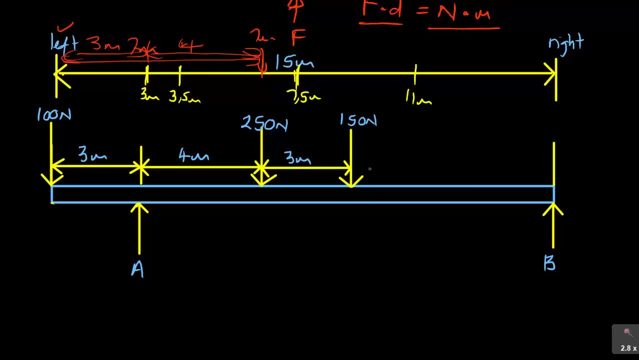 But this dimension left between the 150 newtons, this distance is still missing there. So you need to tell us or you need to calculate and write that distance there. So if I start from here to that distance, we need to find out what is that distance then. that is what they mean when they say it's a fully. 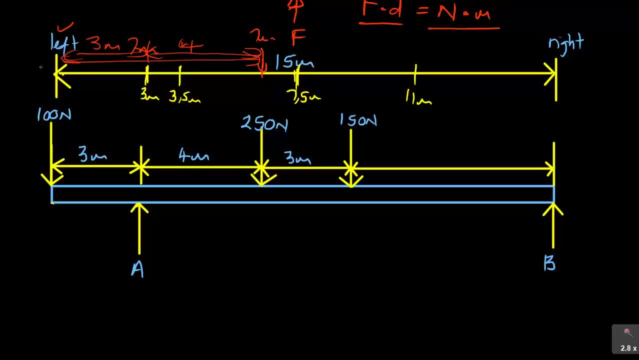 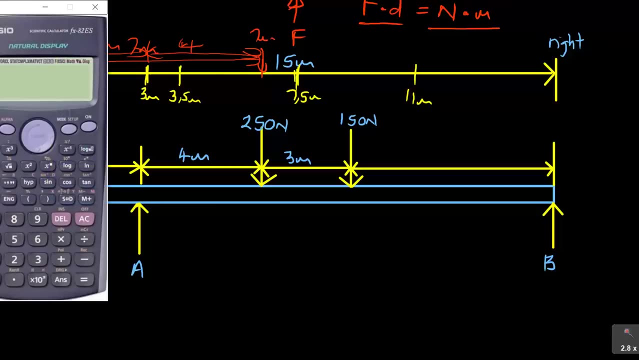 labeled diagram. Now, remember, this beam is 15 meters, So now you have the 3, you have the 4,, you have the 3.. So if you add this 3 plus 4 plus 3 minus 15, it must give you definitely the outstanding size which you're going to write. 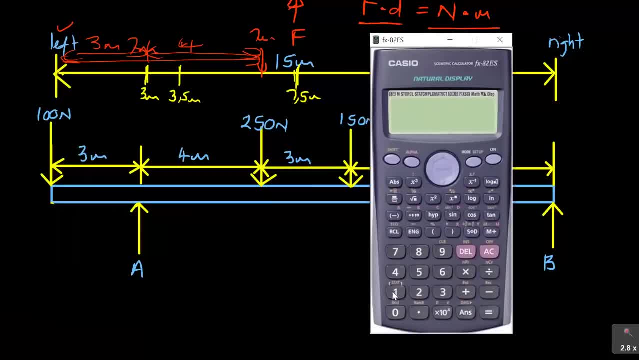 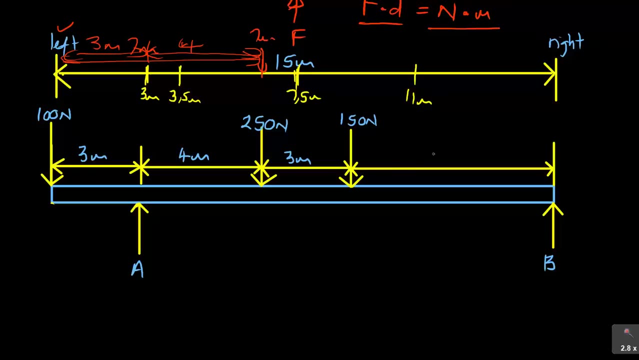 So if I say 3, 3 plus 4 plus 3 minus 15, I'm getting 4.. So which means it says minus 5, but obviously I need the positive answer, So I'm getting this to be 5 meters. 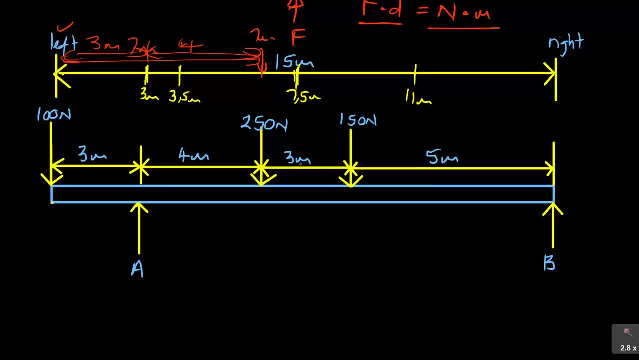 So this is 5 meters, But you say: 5 meters plus 3 meters is 8 meters. 8 plus 4 is 12.. 12 plus 3 is 15.. So this is what they mean when they say this is a 15 meter beam divided into that. 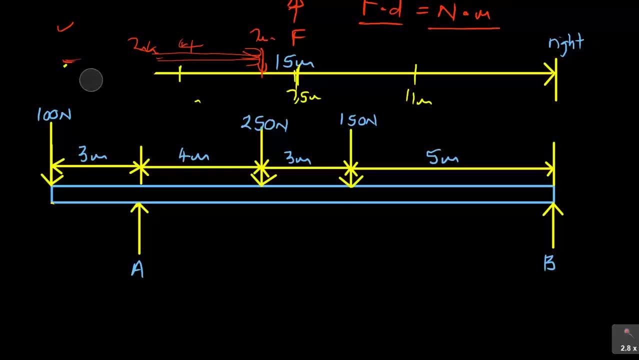 So what you do, you can now take off that just so that Your work- Remember, as I said, this was just to show or to have a way of dividing your answer, your beam, into very neat sketch which even on the beam you can just do that to show that this was your beam, just to make it neat. 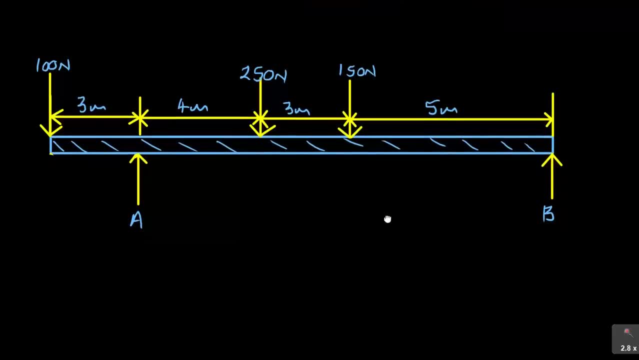 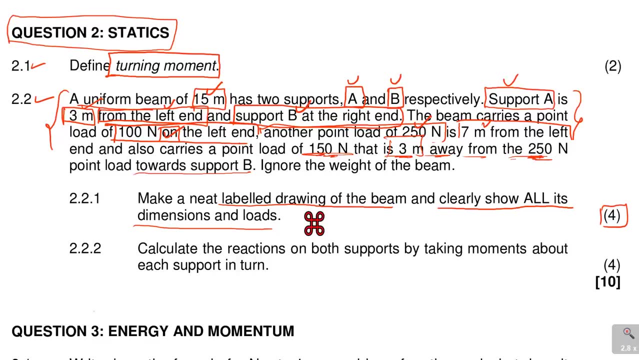 So that's what we're having. So if in this, your question That follows is based on that, It says 3.2.1.. So let's move that. So we are done with this. Let's look at the next question. 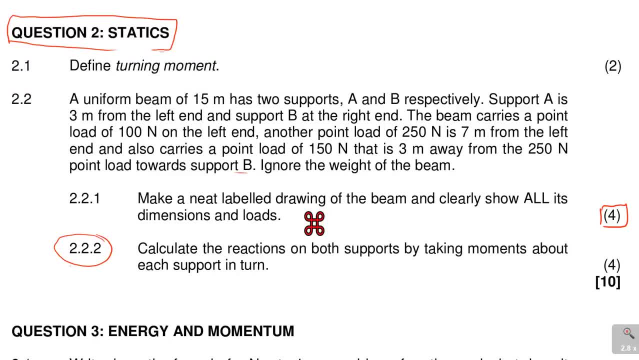 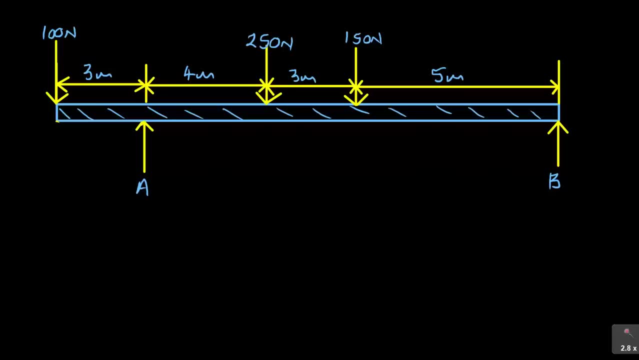 3.2.1.. The question says: I mean 2.2.2.. The question says: calculate The reactions on both supports by taking moments about each Supporting 10.. So this is no format. So now that is what we are looking at. 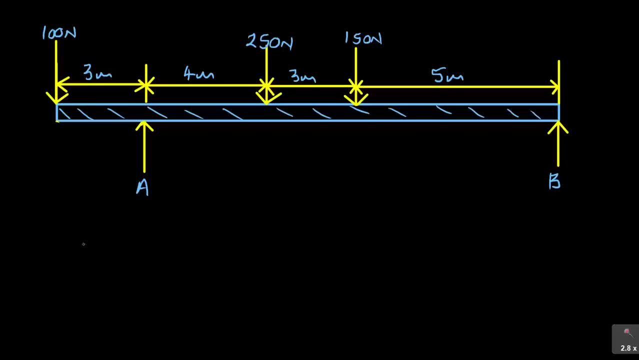 The main thing now is the calculations of that. So how do you go about calculation? All right, Now let's use. you have to state, now say when you're doing your calculations, tech moments. they said above about its support. 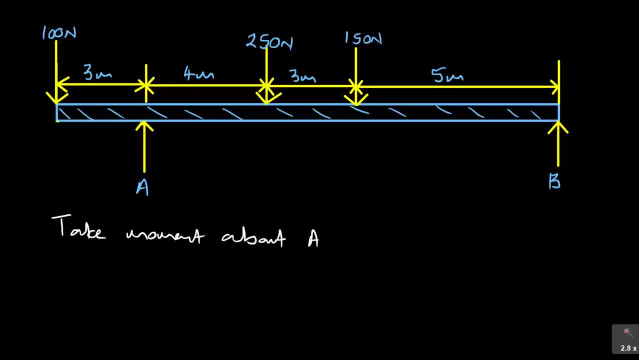 Let's start with moments about a. So if I say, Take moments about a, You are saying: if a is my line of action and everything is resting on a, how are these forces going to behave? if this is the line of action, It means, you see, this force will do that direction. 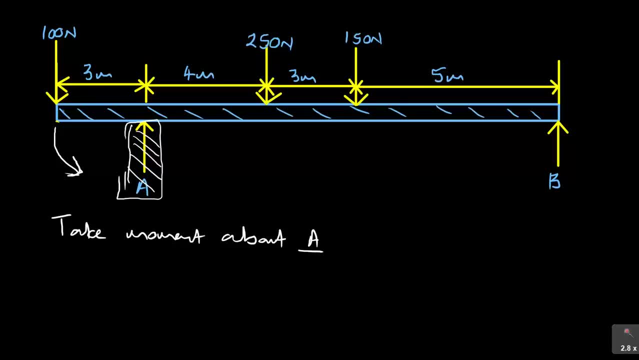 Actually, I think I needed to correct my first statement. Now, this force, you can see it is going to pull this beam or to rotate This, This beam, in an anticlockwise. You see that anti? Then what about the 250?? 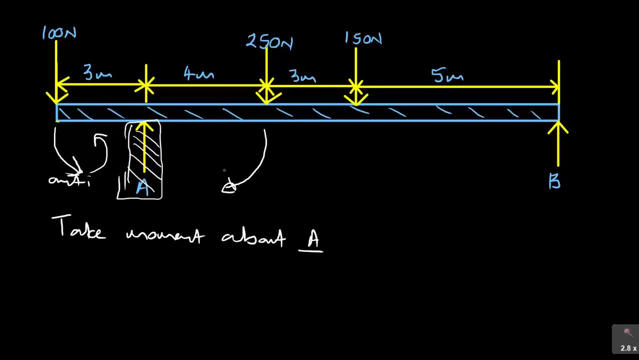 You see, it is going to do the other way around, which is clockwise. Even this other one will do the other way around, which is clockwise. See that? And what about B? B will do the other way around, which is in this case. 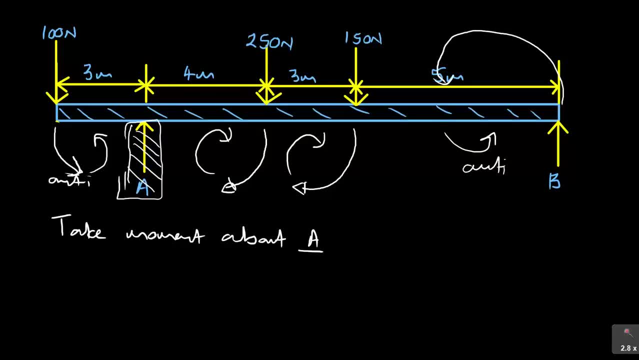 I B is anti. So that is what actually is happening there. I needed to correct the first statement I think that I made. So whenever we are now going to be calculating, to say tech moments about a, we are looking at the 100 newtons. 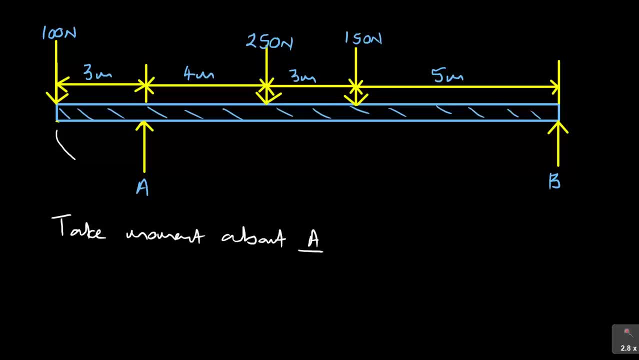 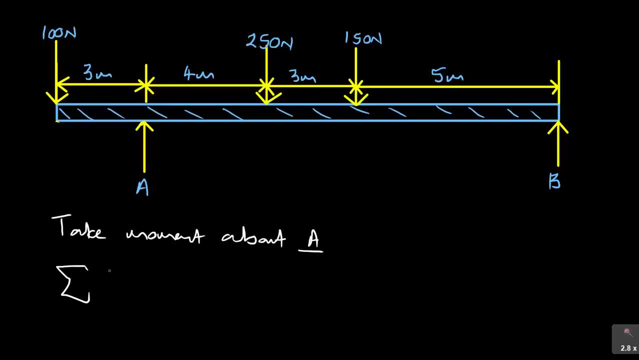 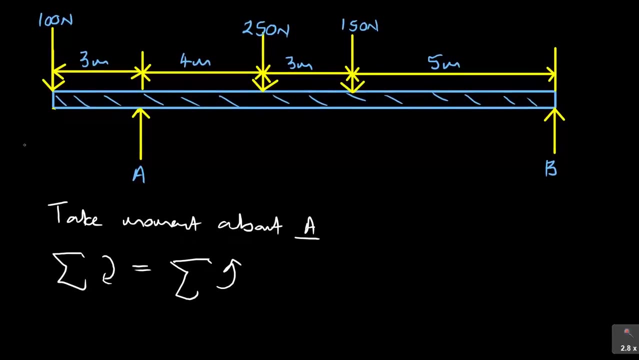 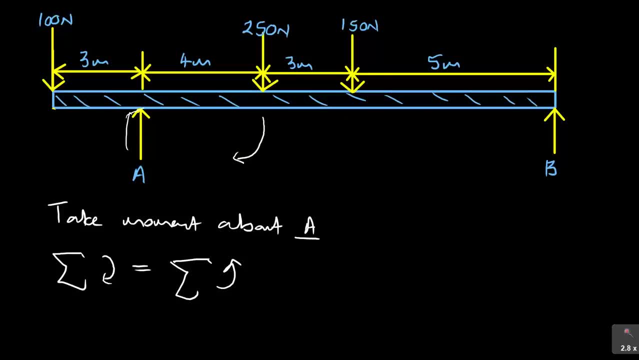 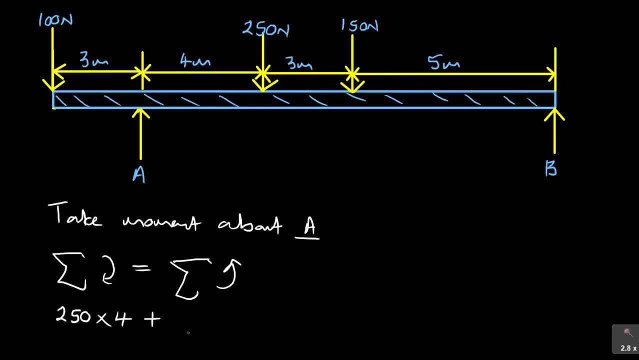 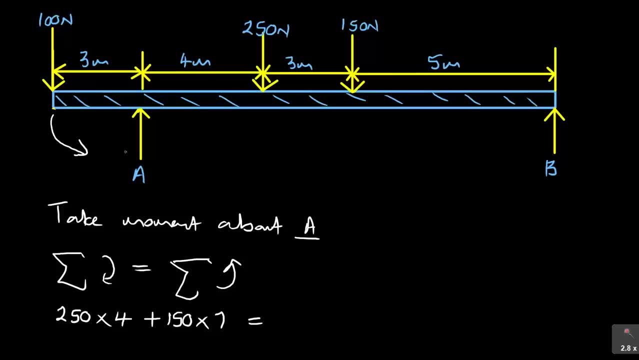 the anti-clockwise about a. there is the force hundred newtons. three meters away, that is, the is producing an anti-clockwise movement, so it's hundred times three and then plus you look at b, b as we say it from a, it will also do an anti-clockwise movement and that will be. 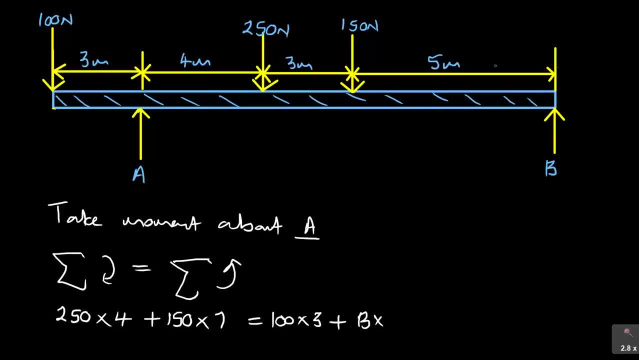 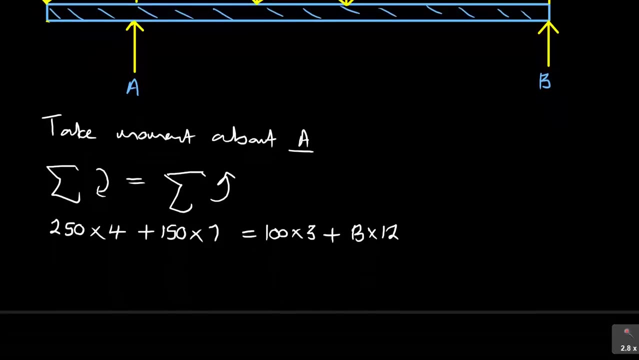 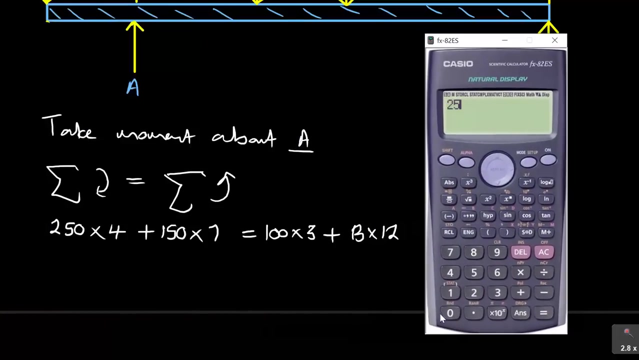 b times. now, if you look at the distance of b from a, it's 5 plus 3, which is 8, plus 4, which is 12. so that is b times 12, and then after that you need to add the left and the right and then find the final answer. so you are going to say 250. 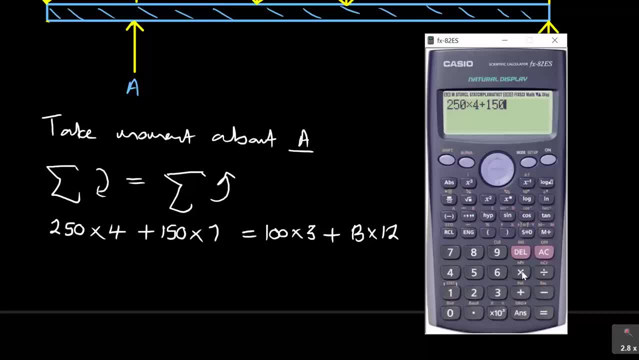 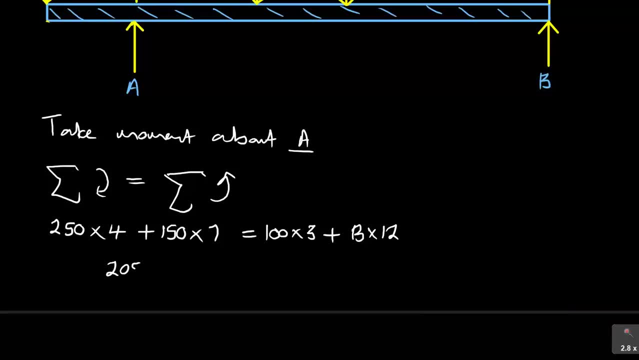 times 4 plus 150 times 7, and our answer is: 2050 is equal to 100 times 3, which is 300 plus b times 12.. and then what we need to do? we need to take 300 to the other side, which is 200- 2050.. now, when it jumps, it changes from. 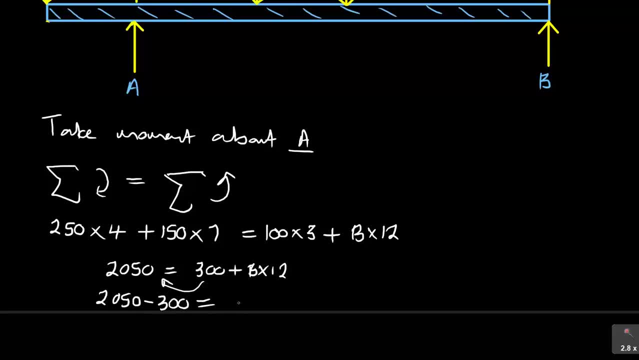 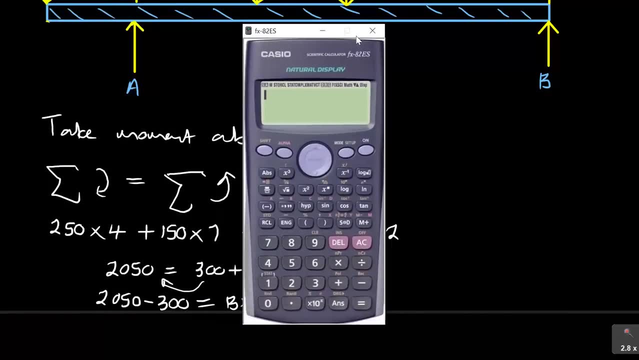 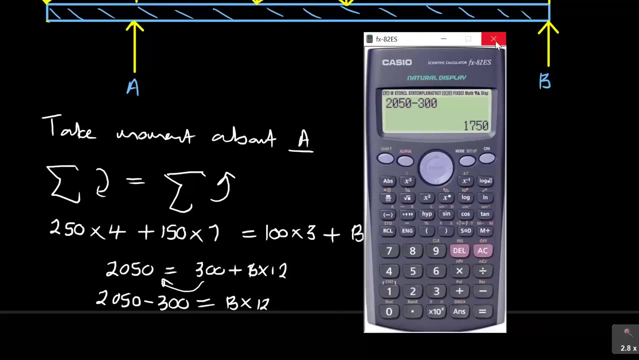 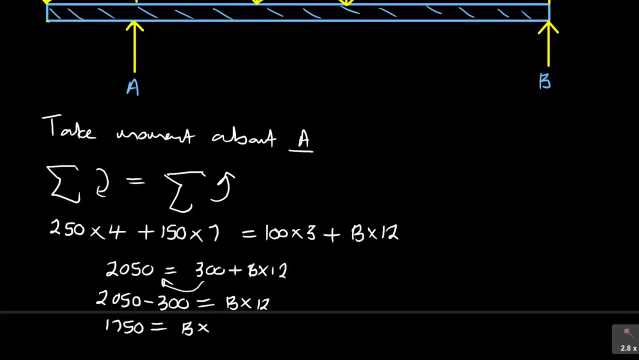 positive to minus 300 is equal to b times 12. and then when you separate 250- i mean 2050- minus 300, you get 1: 750, i mean 1750, is equal to b times 12. you divide in this case by 12 so that you can get your answer. you can see that. 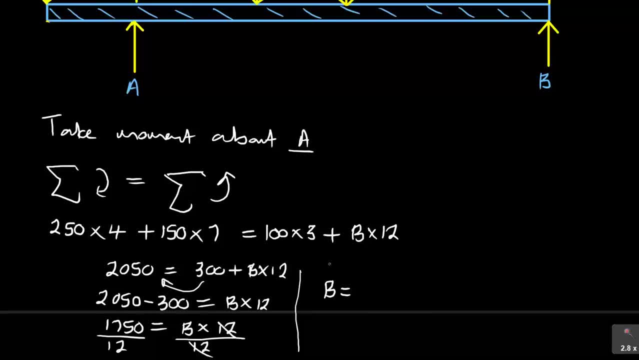 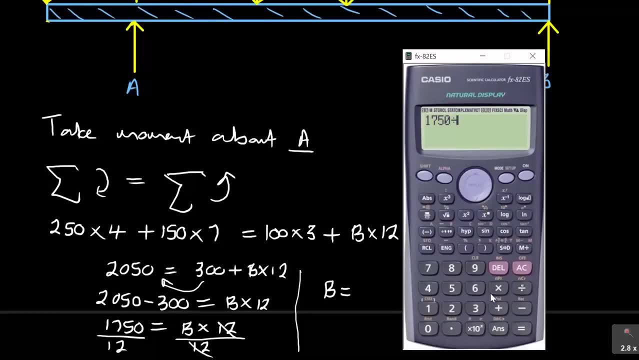 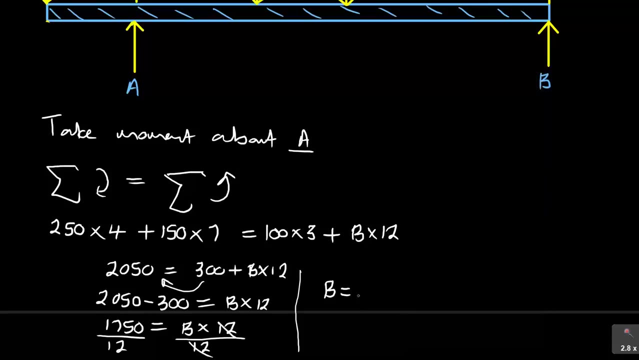 now our b is equal to 1750 divided by 12.. it will give us one 145 comma, eight, three. so i've got one 145, two decimal places, common, 8, 3 neutrons. so that is the first answer that we have for p there. so that is when we're taking moments about a. 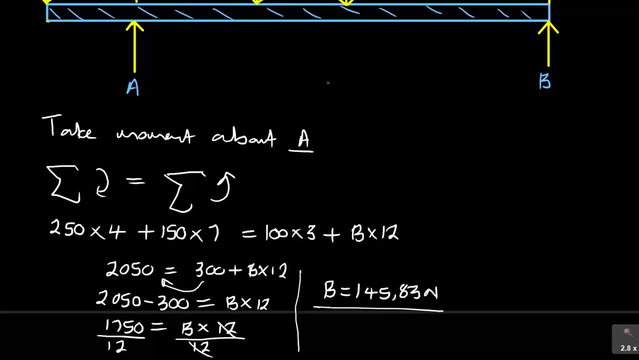 now, what about if we now just have to work everything in this space so that i can see my beam- 2017.07.18. žd season- and now i have to wait in myzinabad 16 hours as an amount to the, though, so in this space, so that i can see my beam? the�umny number 8, 10.iques. so now let me show you. now i have changed anywhere in the result, even though there is, and also now i want to give my ontography. now let me take products 14. 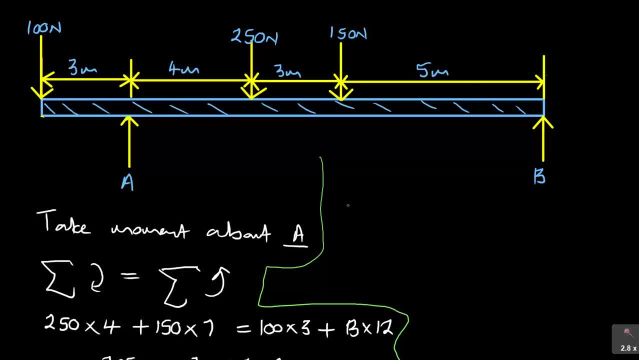 us take moments about b. so i'm going to write here, take moments about b meaning. now my b is my focus. so if b is my focus, i ask myself how will these forces behave if the support is now at b? now you can see that this force, if the support is at b, the hundred newton. 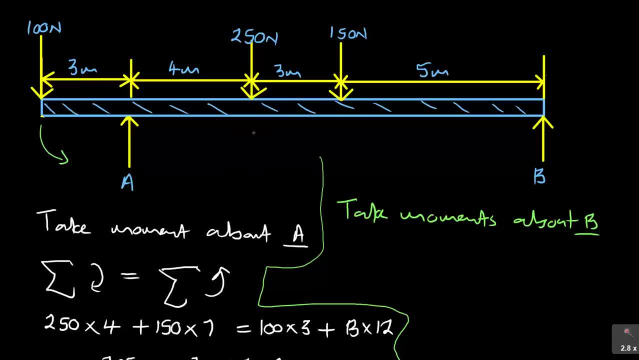 will do that, which is, uh, anti-clockwise. the 250 will do the same, which is anti-clockwise. 150 will do the same, which is clockwise. the only force that will oppose, you see, it, is the a, which will be um clockwise. the rest forces are anti-clockwise and only a will produce. 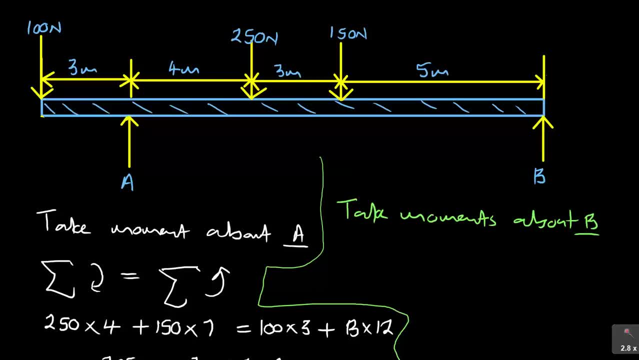 a clockwise movement. so now, if i start doing the calculations, it will be 100. the hundred newton force times b, remember, is you are adding the whole thing a from this point to that point. it was um to b. it is 15 meters, because that's the length. 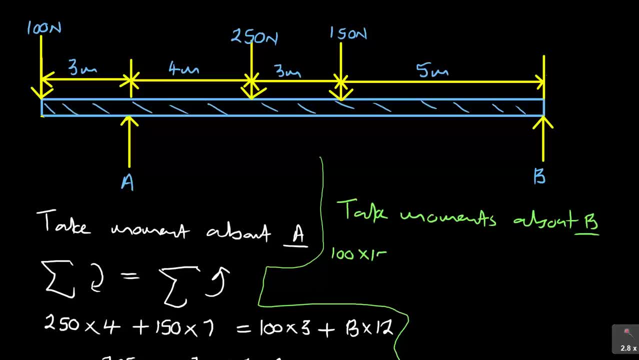 remember, the 100 newtons is at the far end, so it's 100 times 15, plus you look at the 250. what is the 250 from b? so you see 250 is three plus five, which is eight meters from b. so we're going to say 250 times eight and then plus the 150 is five meters away. 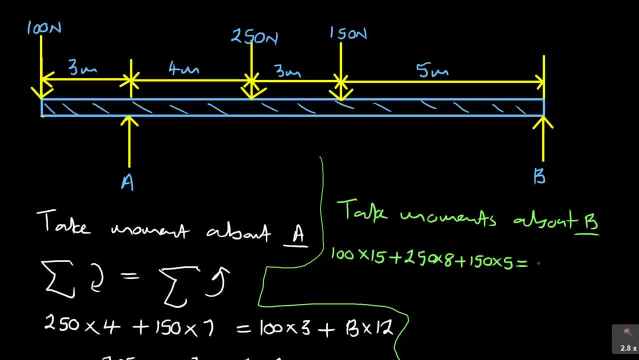 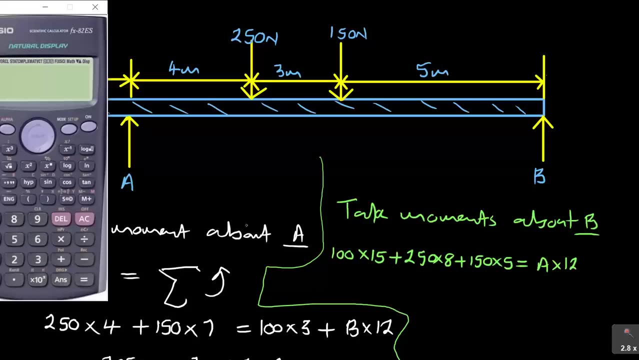 this is equal to what? about a from b? it will be a times the distance of 8 from B is 4 plus 3, which is 7, 7 plus 3, which is 12. so it's 8 times 12, and when we use the calculator again, we have 100 times 15. 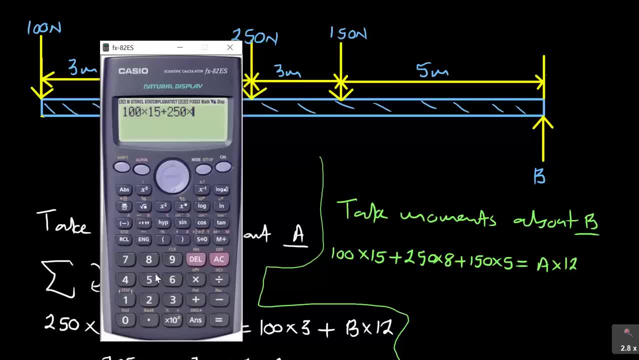 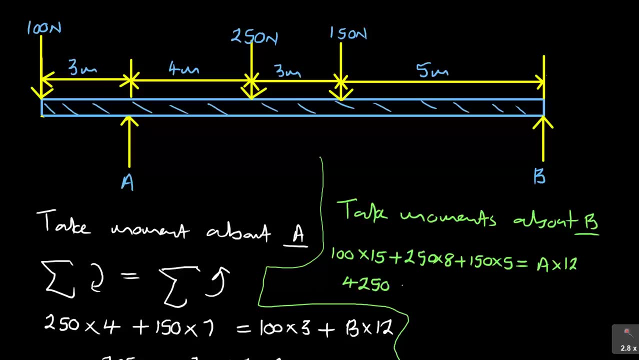 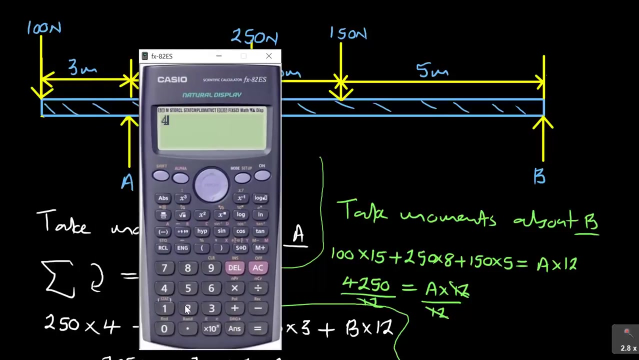 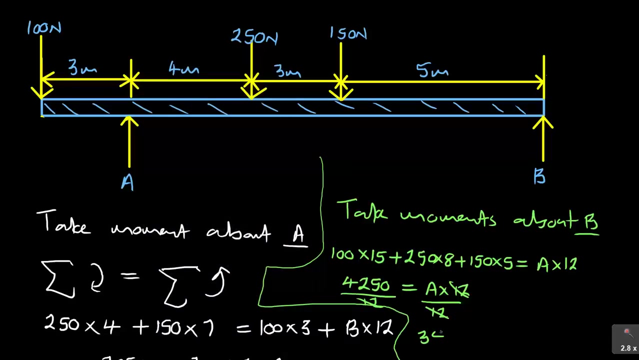 plus 250 times 8, plus 150 times 5, and then this is 4250 is equal to a times 12. then I divide by 12 on both sides so that I can get my a. so you divide 40 to 50, divided by 12, it gives me 354 comma 16, which is 354 comma 17. so I've got three, five, four comma. 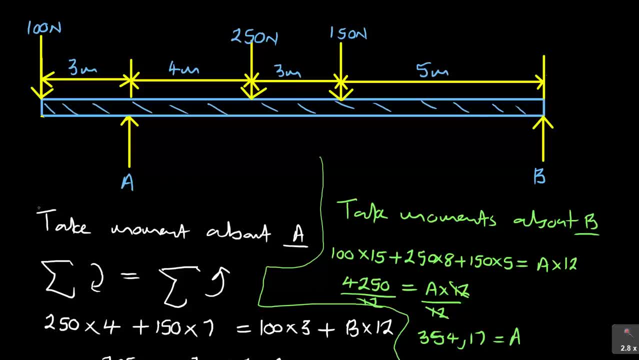 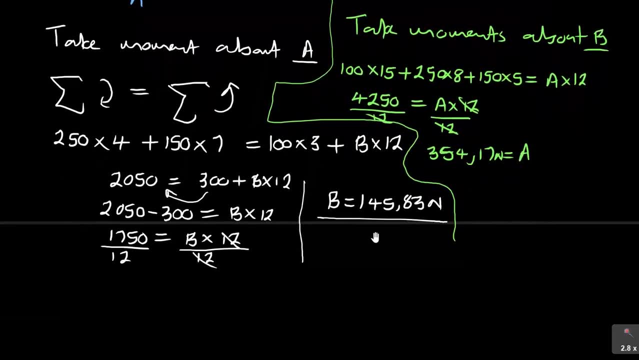 one seven is equal to my a. remember it is in new tones, we mustn't forget the units. so this is what I'm having in this case. so in other ways, my, my, my a, or I write it properly: a is three, five, four comma one seven neutrons. so this is the answer to the question. and they calculate the region at what? 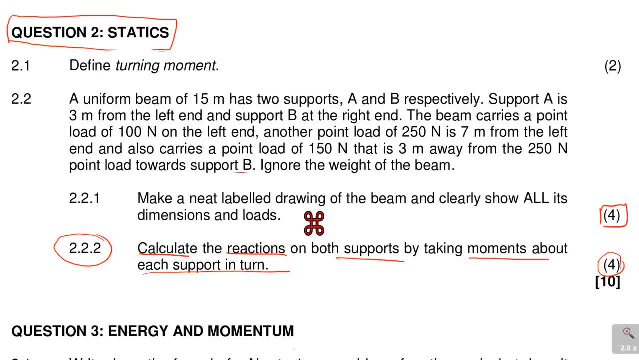 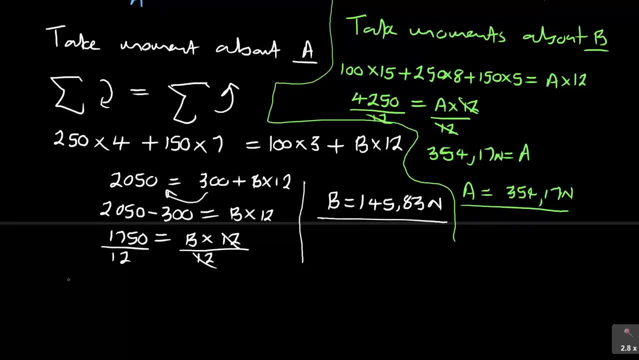 end by taking moments about the support in the 10, but now I need to test my answers here. remember, you can test here your answers. so how do you test your answers? some questions they'll actually say: test your answers now how do you test what you're doing? is you're going to look at all the sum of? 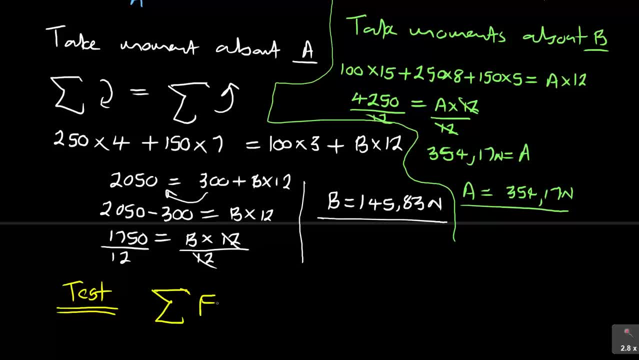 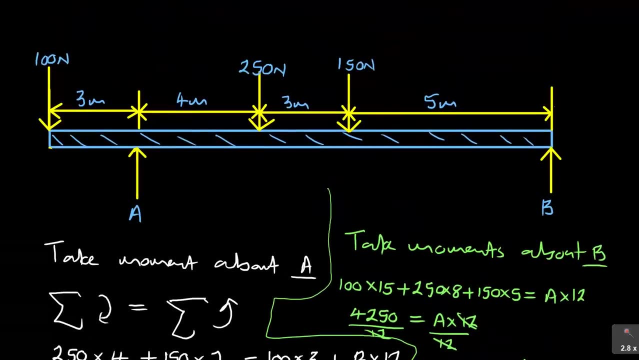 forces that are facing, for example, up must be equal to the sum of forces that are facing down. so let us look at our analysis. we have got all the points. this: this is facing down, that is facing down, that is facing down. so you look at all the forces that are going down, which is 150 plus 250 plus 150. so those are. 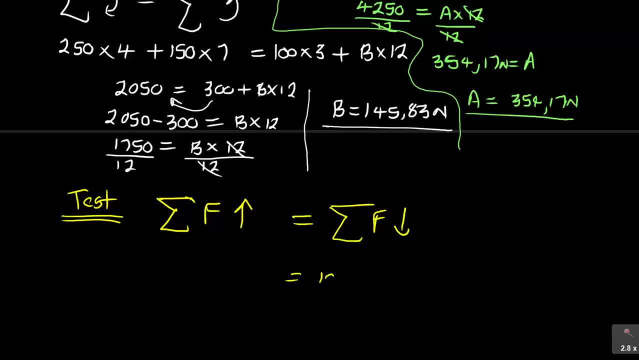 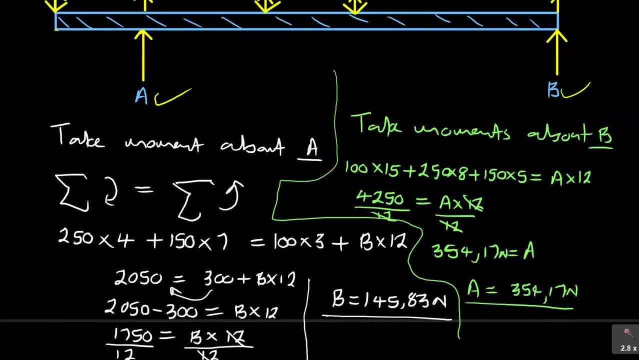 facing down here, which is the hundred plus the 250 plus the 150, and then you look again at the forces that are facing up, which in this case was our a and b. they are the ones that are facing up. these forces must balance. and then we did. 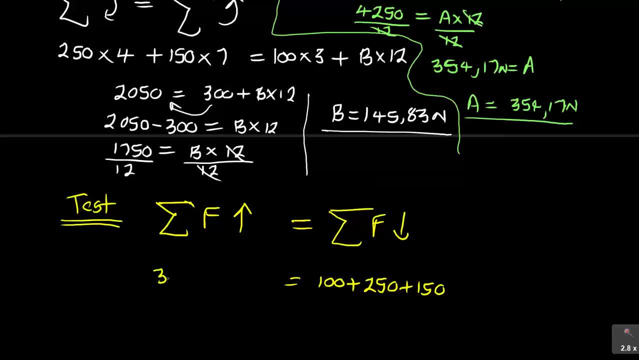 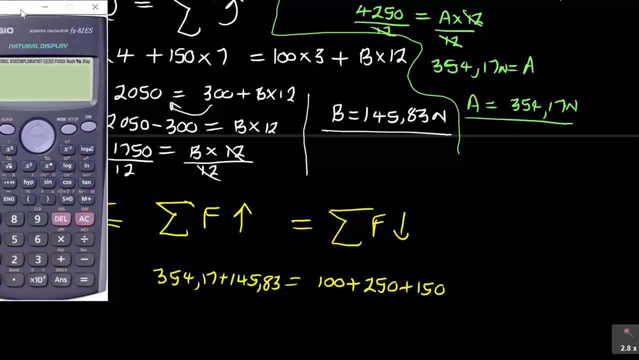 calculate a and b. we said a was 354 comma 17 and b was um 145 comma 83. if this balances, it means your calculation is correct. if they don't balance, go back to your calculation and correct it. so if I say three, five, four, 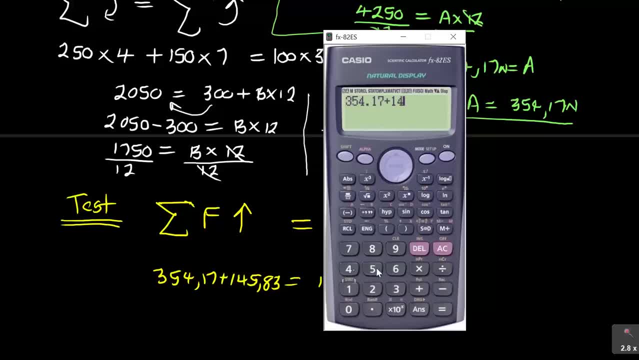 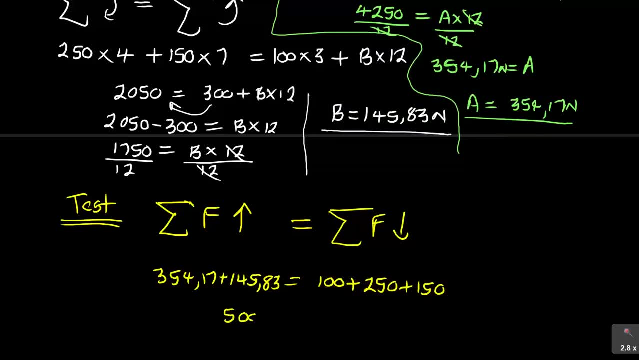 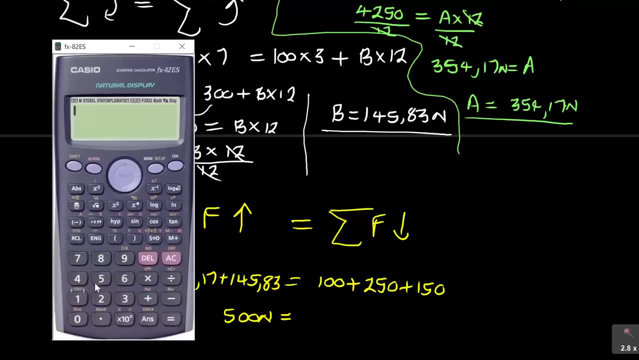 comma one, seven plus one four. five comma eight, three. it gives me 500. so I've got 500. Newtons on the other end is equal to. then I also add the other side, which is 100 plus 250 plus 150, and again it is 500. so you can see now that 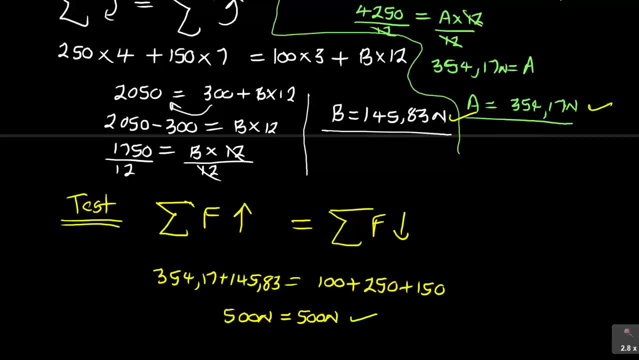 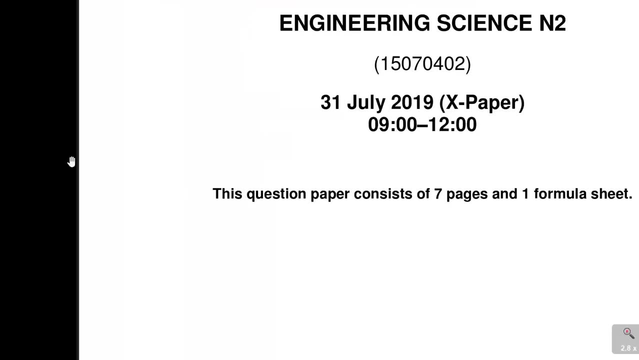 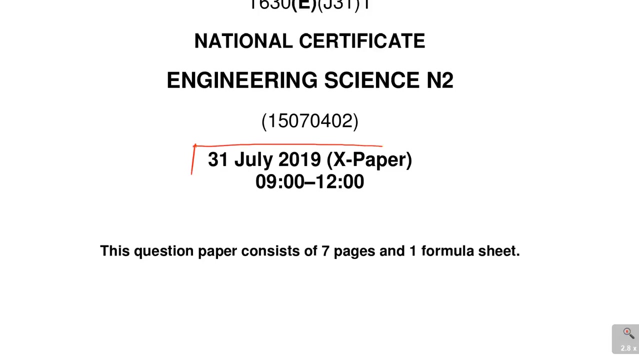 this balances, which means my b and my a. they are correct as far as this is concerned. so that is how we work on this question. as I said, I took quite some time focusing on this question, but now let us try to be a little bit faster with this one. this is a July 2019 question, as you can see, and 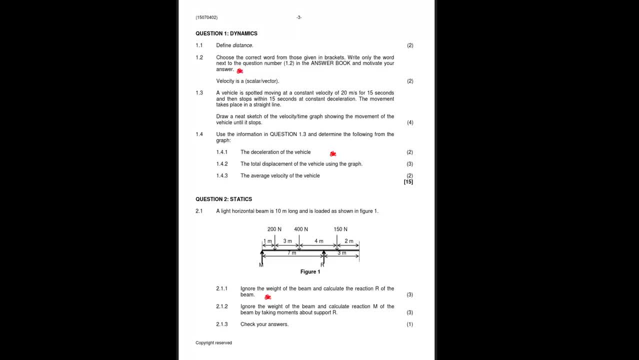 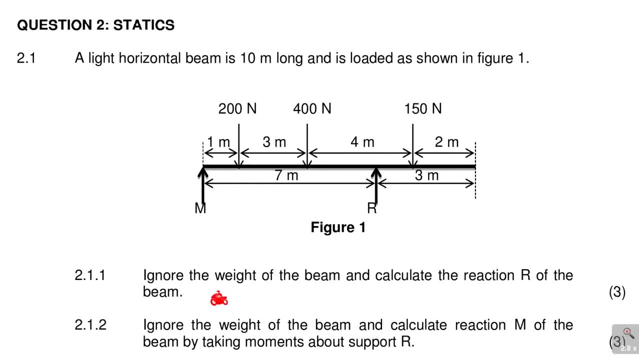 I'm looking, or the focus here is on moments. as I said, I'm not going to be focusing on other parts, but it's on statics, question number two- you see that one again, and question number two deals with moments. so look at 2.1, it says a light. 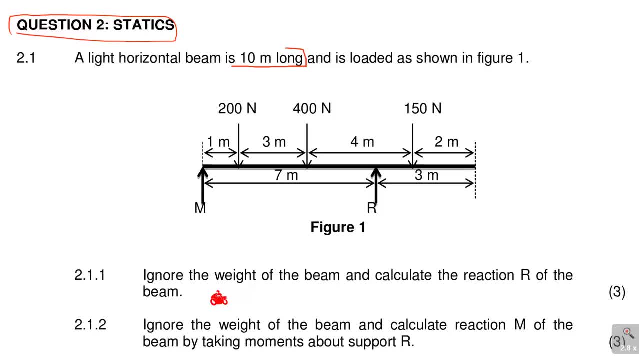 horizontal beam is 10 meters long. so we have a horizontal beam that is 10 meters long, that is shown here and is loaded as shown in figure one. so let's look at this beam and study it. you have got supports m and r, and the first support is one meters from the end. then the 400 Newtons. the 400 Newton's support is 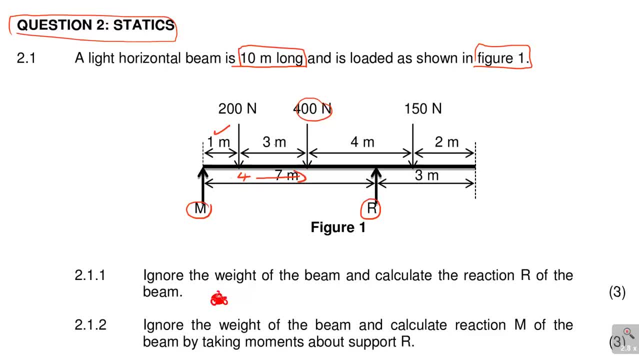 one plus three, which is more like four meters. you see that we have got a four meters distance there. and then that's where they wanna confuse you here to say from R. you see, they mixed up and they mixed up these distances and we have to be careful how we analyze that. now the 150 is not difficult from M. you get that we. 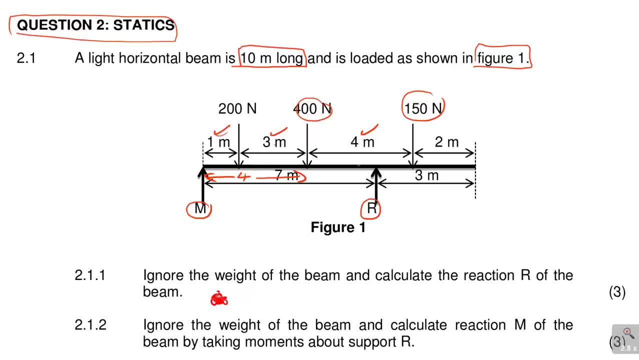 get that, you get that. that's not a problem. now the challenge comes when you want to find the distance of the 400. if we look at the distance of the 400- or let's start with the 200- the distance of the 200 from that end and the 400 from, 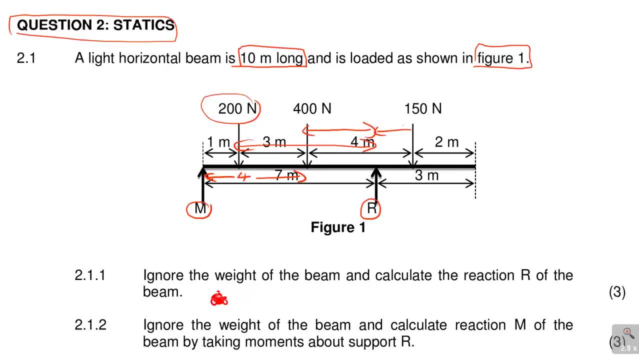 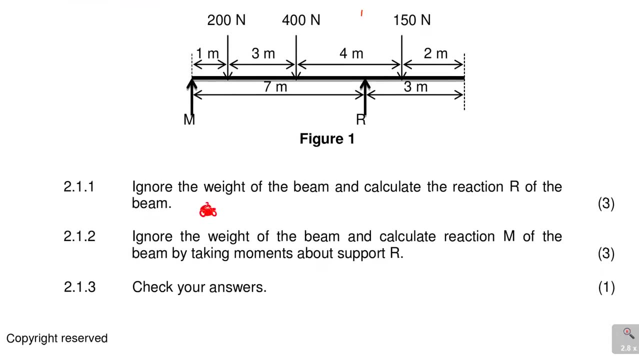 that end and the 50 from and the reaction are. so if this is to be divided, we need to find that particular distance in a way. but let us- let me not get hell ahead of myself- let's look at the questions it says. ignore the weight of. 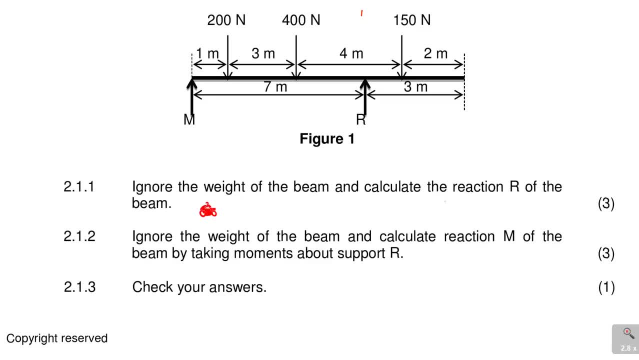 the beam and calculate the distance of the beam reaction. the reaction are of the beam, so they want us to calculate the reaction. are of the beam, to say what is the reaction are from the given measurements. so now, in other ways they are saying: take moments about, are. so if 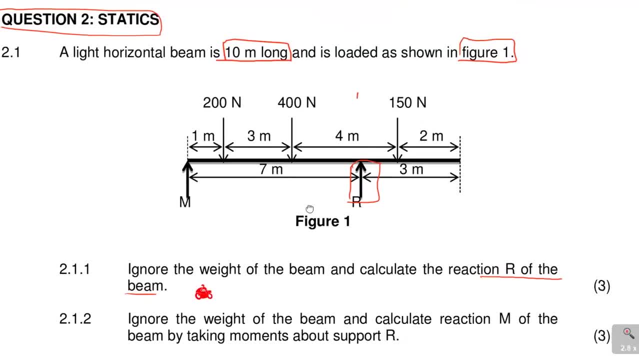 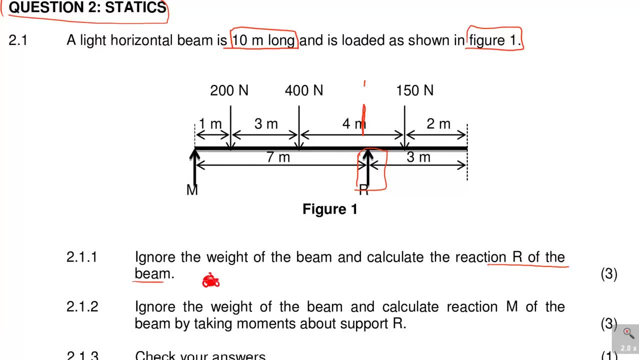 we're going to take moments about are we need to be also sensitive to the distance. as you said, we need to know what is the distance of the beam and what we need to know, what is this particular distance? because this distance, these doses, will determine the Gaussian. 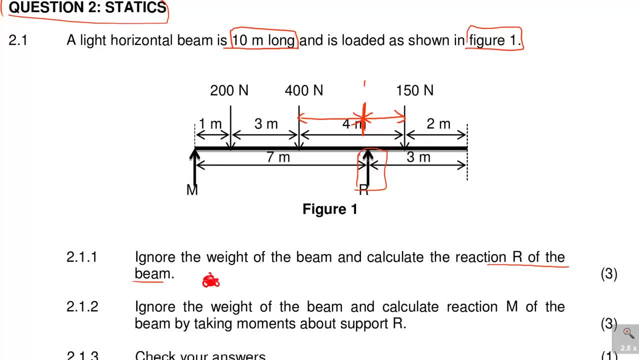 descent solid level, because these dosage will determine our distances from this part of are. so now, remember you are, given that a was one. we will determine the distance. as you said, we need to be are, so we need to be also strict to time, but is the distance is determined silent, so it's slightly αυτό. 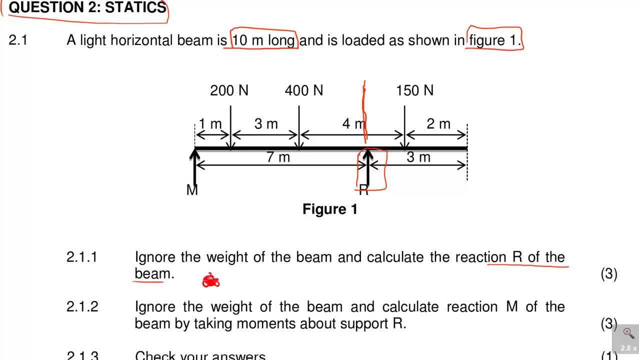 so that I don't close that for so. we- so that I don't close that for so S- know that the whole distance in the distance is a special criterion for the That we're given there is 4 meters, but look at the bottom. The key is in this part that you're given there. 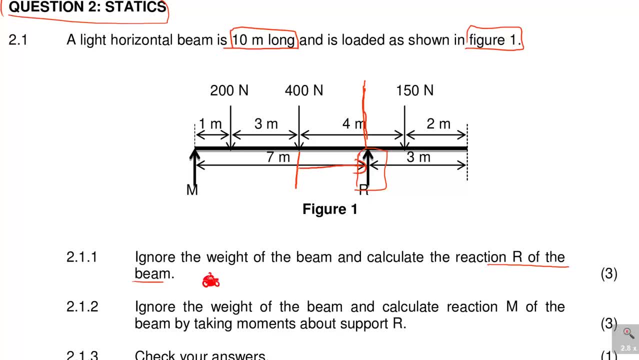 Let me not make an error. Look at that Now, and then again, look at that. We are told that this beam is 10 meters long. so we know, at the bottom, 1 plus 3 gives me 4 meters here, and then from This point to this point it has to be 3 meters so that it will add up to become 7 meters. 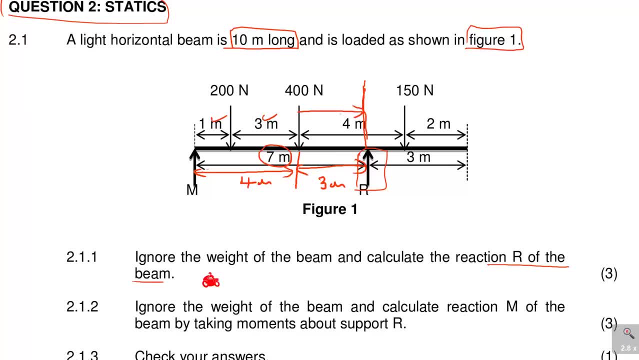 So you can see that from here to here It is 3 meters. now, from here To here it has to be 1 meter, so that 3 plus 1 will give me the 4, so that now we managed to crack this distance. we know that it is 3 meters and 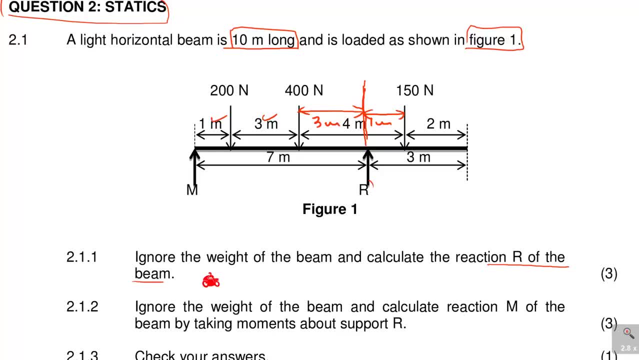 1 meter. so now we have to take moments about R. Now, if you take moments about R, you have to ask yourself: What are the effect of these forces about R? now look at the 200 Newton. It will rotate. you can see how the rotation is anti. 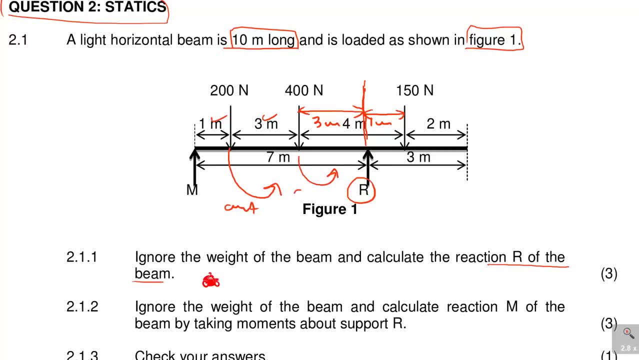 You look at the 400 about R, It's anti. Remember, this is our main part, We're focusing. it will cause this thing to go down and in this point It's going down, it's going down. but now look at the 250 about the hundred and fifth about R. this force will cause it actually to go in the other direction, which is clockwise. I 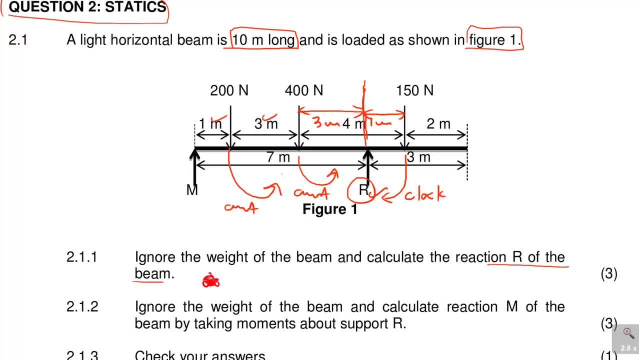 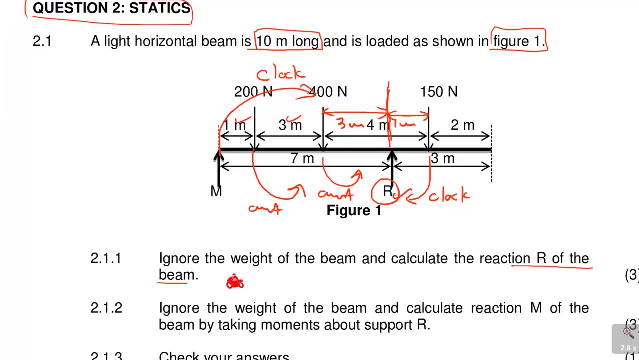 think that now, what about the M with respect to R? you can see that the M is going to push it up and also do a clockwise. You see that. so now we can now come up with our Formula. remember what it says. it says sum of. Let me just do it just here. I think I can just be something. remember. it says some of. 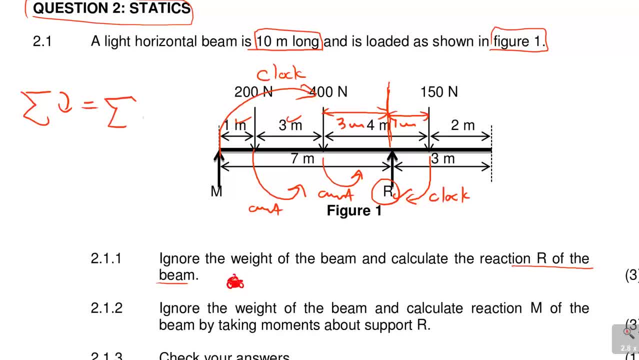 Clockwise moments is equal to sum of under clockwise moment. so we're going to look now at the clockwise moment that we're having and the first one is this force. it is clockwise so, which is 150 Times the distance of the 150 from R. We say it was 1 meter. 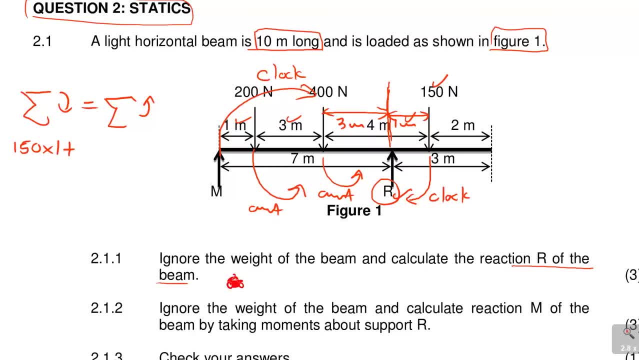 Plus the next one that is clockwise is the M here, which is M Times the distance of M from R. You can see that what they gave us, they is 7 meters because it's 1 plus 3 plus 3, but at the bottom It's clear there. 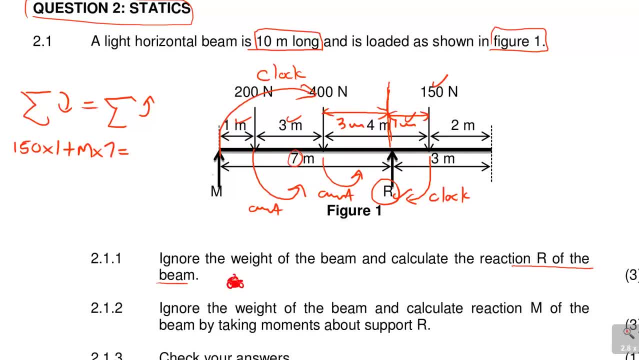 You see that this is equal to The 200 Newtons. You can see that's the one that is anti clockwise, 200 Newtons, but the distance of That it's 200 times. so we have got the 3 meters, and Then we also have the 3 meters, so it's 3 plus. 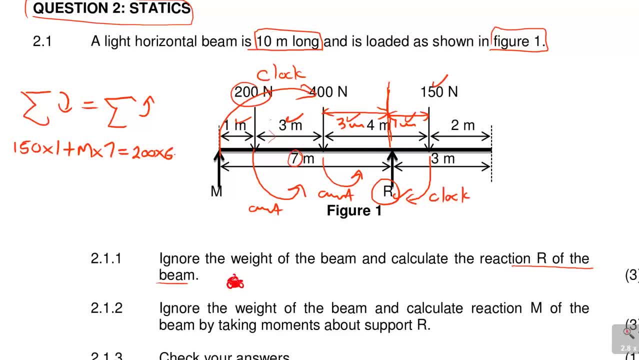 is 3 plus 3, which is 6, and then plus the 400 Newtons, which is 400 from R is 400 times 3, so we've got 400 times 3, so let me just Have that. so it's 400 times 3. 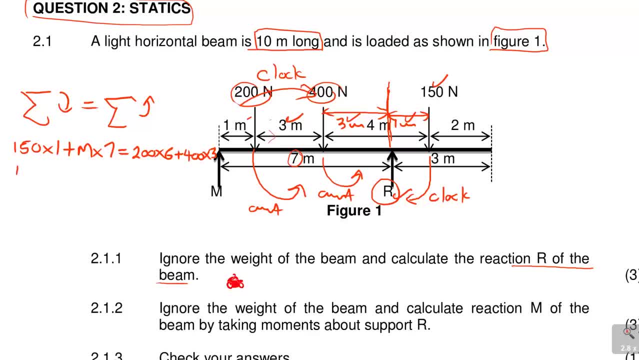 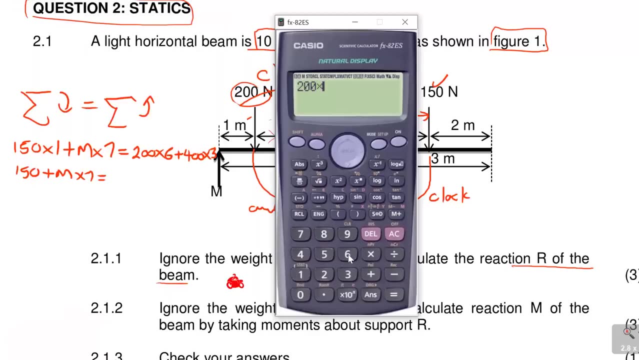 So these are the way you're going to calculations. so what you have is plus M times 7. This must give me, If I use now My calculator here, must give me 200 times 6 plus 400 Times 3, which gives me 2400. 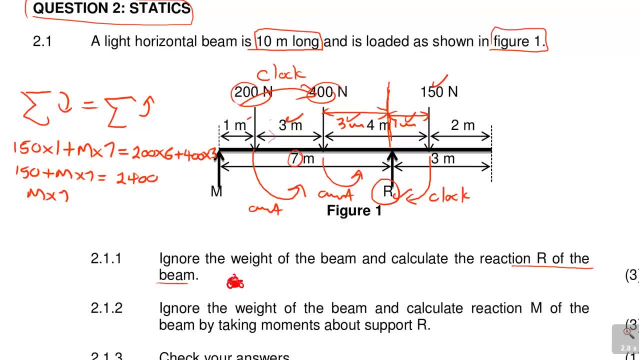 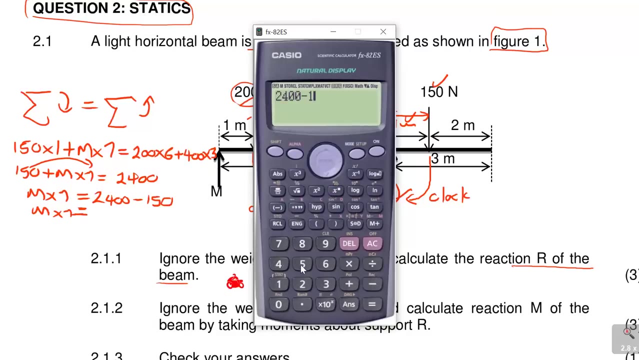 So now M times 7, you take 150 to join that, it will become negative, which is 2400 minus 150. remember it's jumping the equal sign. so M times 7 is equal to Says to 400 minus 150, which is 20 to 50. 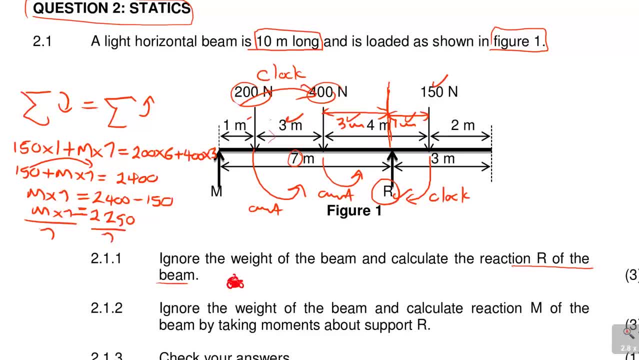 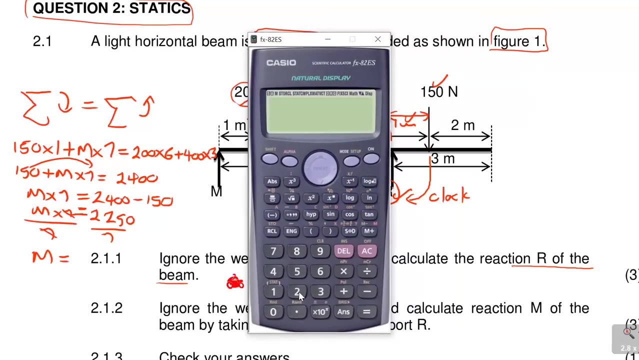 So what you need to do? divide by 7 so that you get your M. So what is M? That is the reaction 8, in this case The reaction at M So away, that is 2250 divided by 7, which becomes 321, comma 4, 3 if round up the two decimal places three to one comma or three. 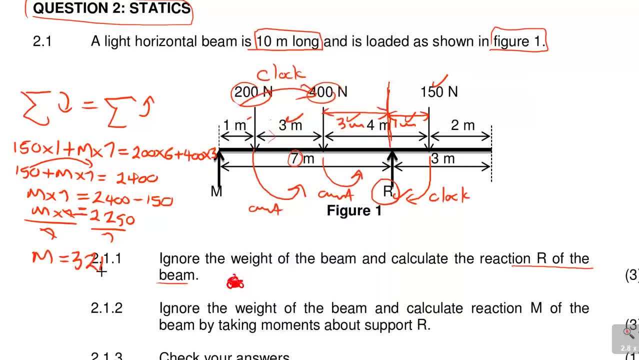 three. so that's three hundred and twenty one comma four, three. that is in Newton's, so I'm gonna keep that one to say: they say direction, M says okay, the first one does. the reaction are- so I'm gonna write it here- is three hundred and twenty one. 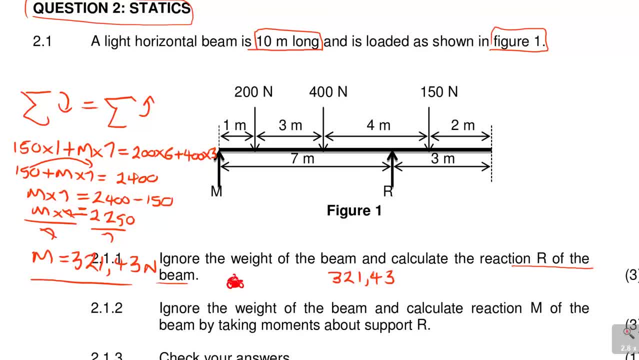 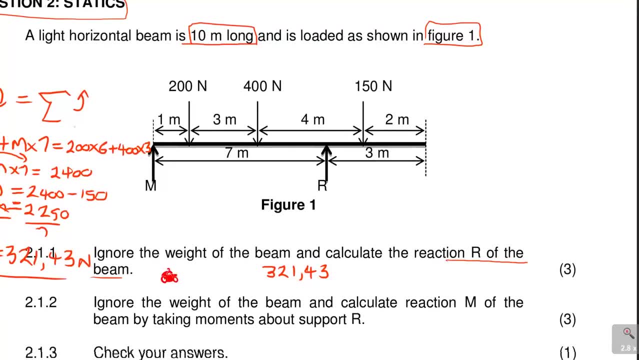 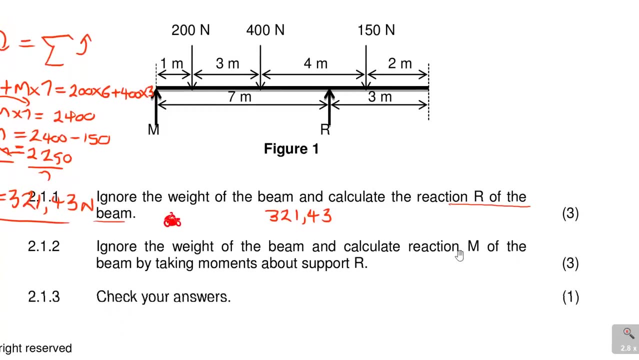 comma four, three, all right, so now let us look at the other one. I'm not gonna erase that, just to keep my working question, in this case two point one. point two: ignore the weight of the beam and calculate the reaction M by the beam. taking moments about support R. 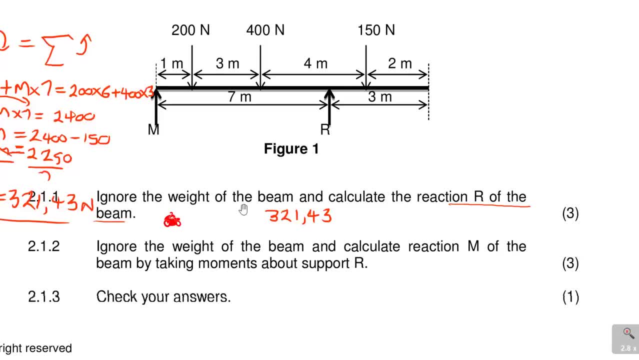 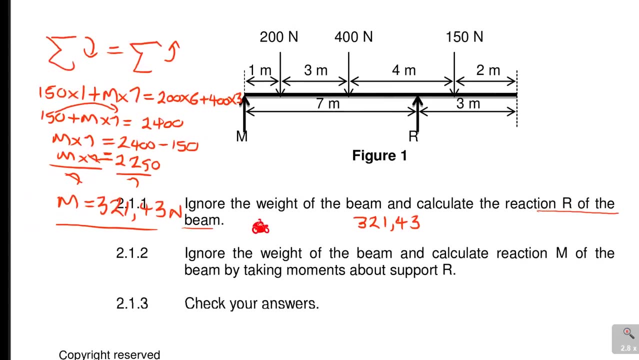 and the first one was ignore the weight of the beam and calculate the reaction R of the beam. so we've calculated, actually, the question. I did the question other way around. I was supposed to take moments, this question, this particular question. I didn't read it right. I was supposed to take moments about and this 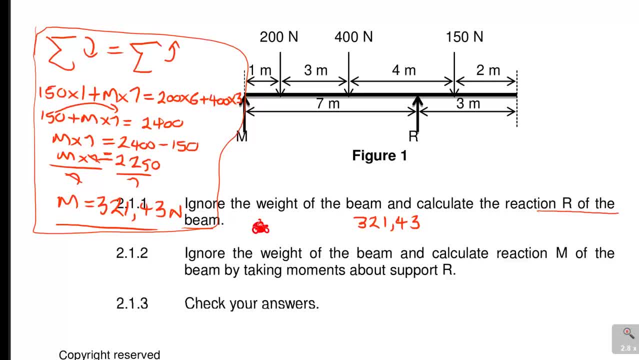 is taking moments about M. that's why I says: ignore the weight of the beam and calculate the reaction you M of the beam by taking moments about support R. so this is actually the question for two: point one, point two. now I'm looking now for question for two. 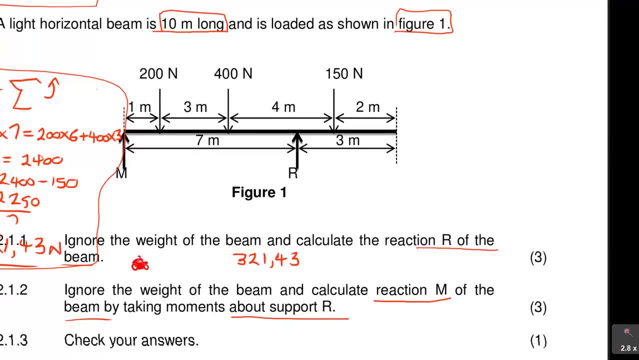 point one. point one is the first question that I was supposed to do. he says: ignore the weight of the beam and calculate the reaction R. if I'm to calculate reaction R, I must take moments about M. I think that. so now, if I'm taking moments about M, 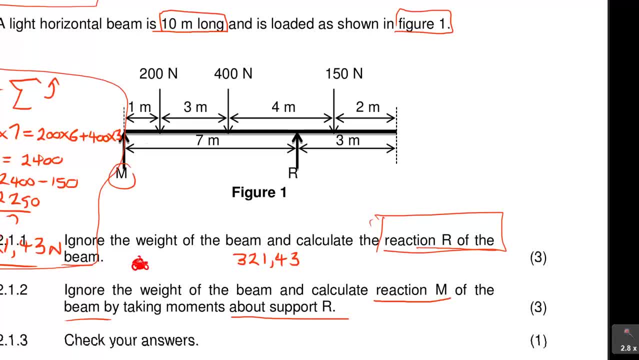 what I'm going to have is that with to say, if this is my focus here now, you see, this force will turn like that, it will turn like that, it would turn like that. so all these are clockwise. so sum of clockwise is equal to sum of anticlockwise. so let's look at the clockwise at first. we have got the 200 M. 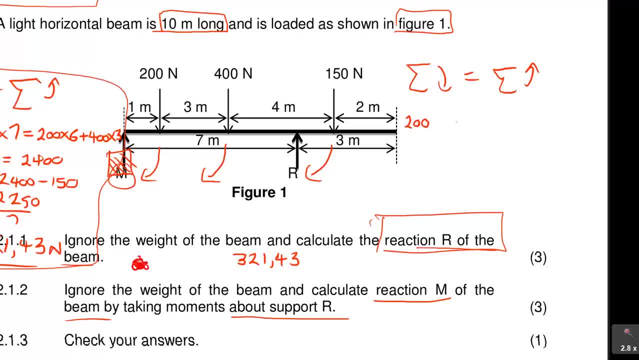 we have got the 200 M From M is times 1, plus we've got the 400.. Now again, 400 is 3 plus 1, which is 4, plus we've got the 150. there times now it's 150, it's 4 plus 3, which is 7 plus 1, which is 8.. 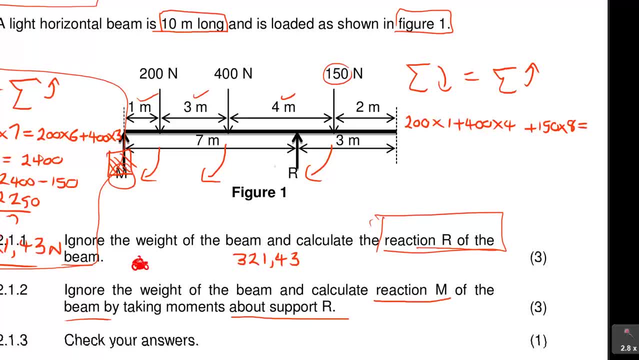 And this must be equal to look at the one that is going to produce an opposite effect, which is R. see, R will produce an anticlockwise. So what is the distance of R from M, which is equal to R times 7 in that case? 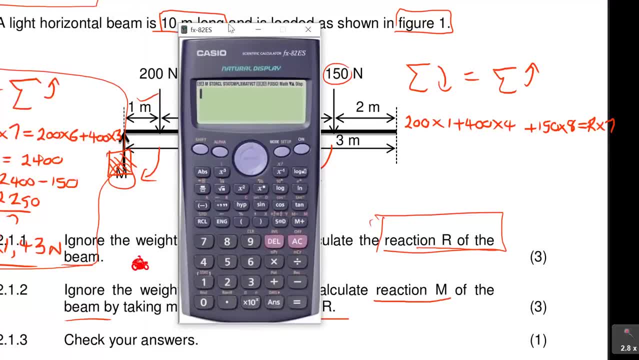 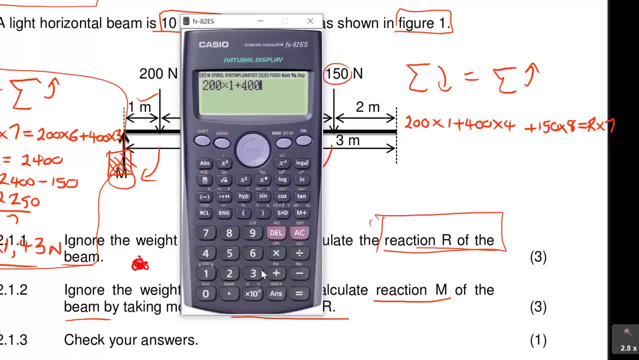 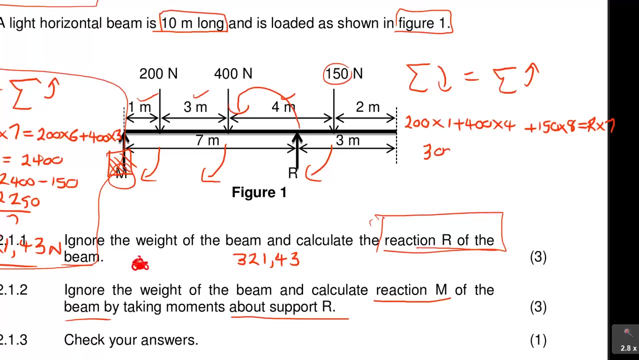 So you can use the calculator then to find that, which is 200 times 1 plus 400 times, So that means 4 plus 150 times 8, see that it will give me 3,000.. So I've got: 3,000 is equal to R times 7, divided by 7 on both sides, so that it will give me my R. 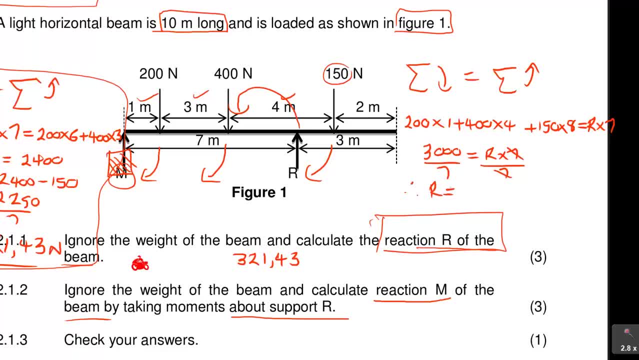 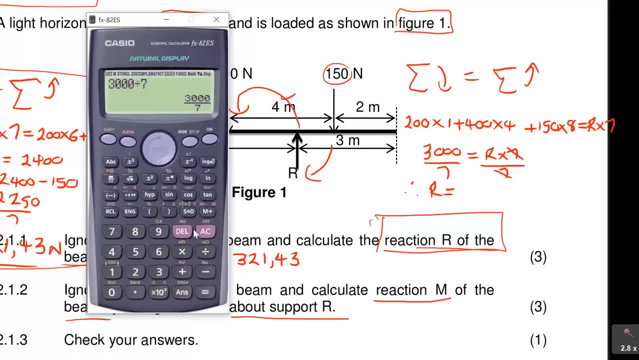 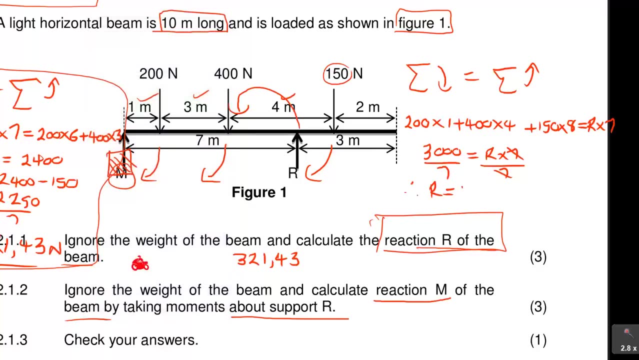 Therefore, my R is equal to, in this case, 3,000.. Divided by 7. And if I do that, it's 428,57.. So it's 428,57 newtons. So that's what I'm having in here. 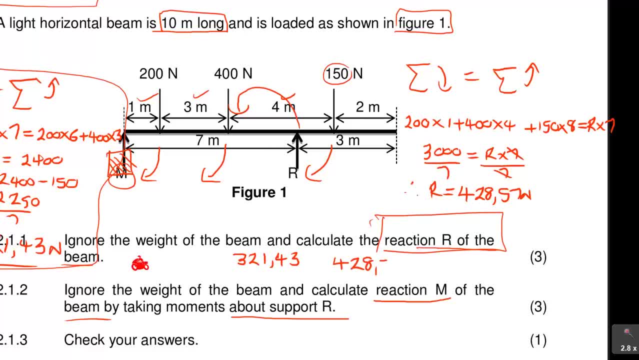 It's supposed to be 428,57 newtons, And this one is down there which is 321.. So it's 428,57 newtons. So that's what I'm having in here. So that's what I'm having in here. 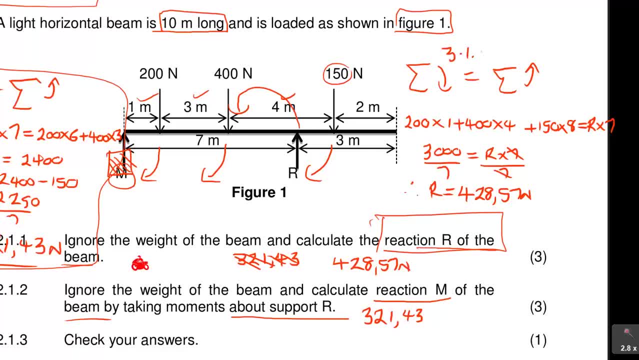 Remember we said this is question 3.1.1.. This was 3.1.2.. I just didn't read the question properly. It was supposed to be. when they say calculate the reaction R, meaning take moments about M and the vice versa. 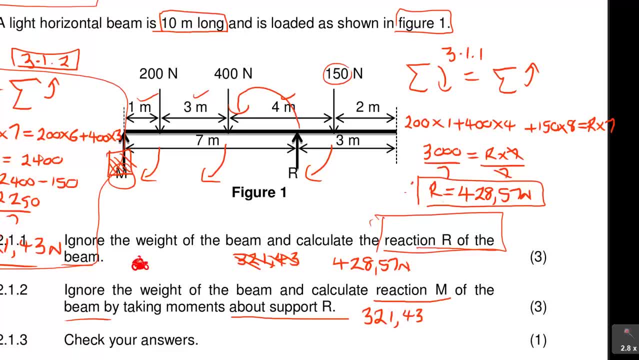 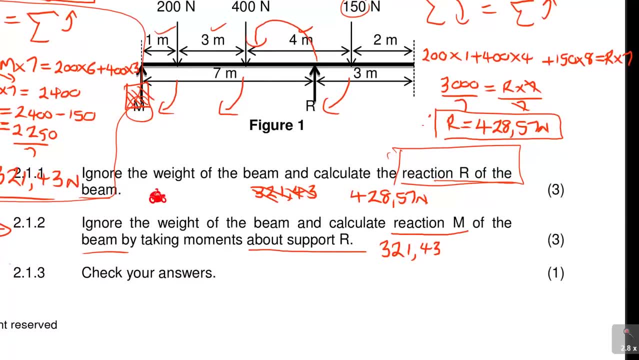 So this is: see, now it's giving me R in that case. And then look at the last question. there It says: I need to check my answers. See, now, That is where It's saying some questions. They say: check your answers. 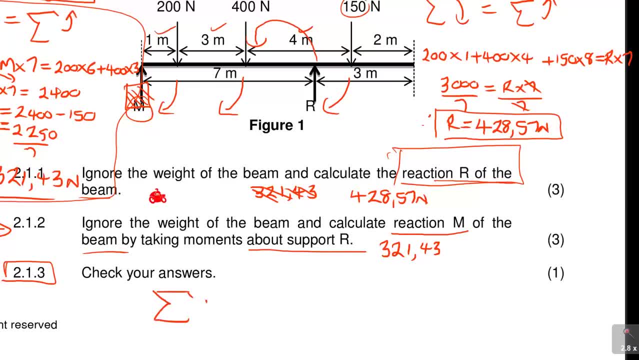 When you check your answers, you are saying the sum of upward forces is equal to the sum of the downward forces. That's what we're saying. So all forces that are facing up it's M and R. So you say M plus R. 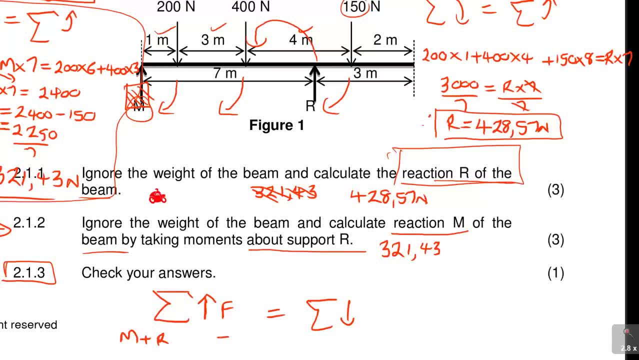 These are the forces that are facing up- is equal to the forces that are facing down, which is 200.. Plus the 400, plus the 150.. All these forces, as you can see, they are facing down. So now, what is M plus R, though? 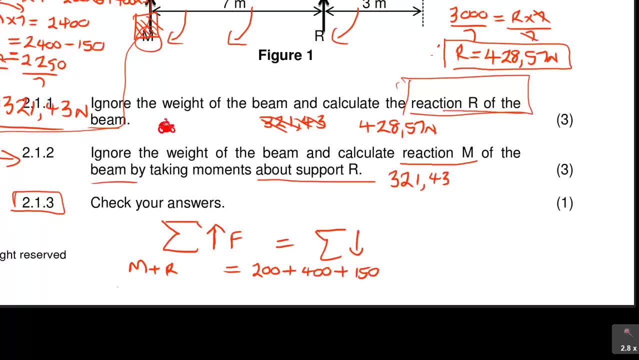 M plus R. we said M was in this case. this is my M, This is my R. So M is 321,43 plus my R is 428.. Comma 5, 7 is equal to the 200 plus the 400 plus the 150.. 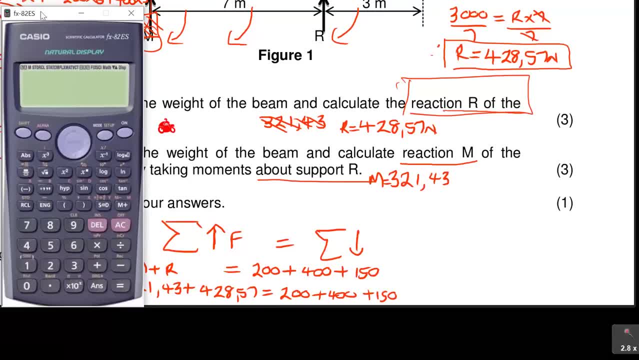 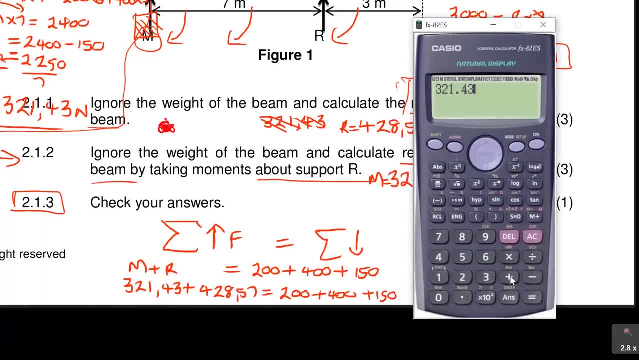 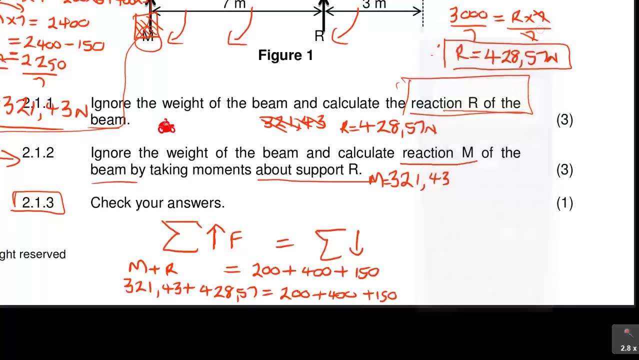 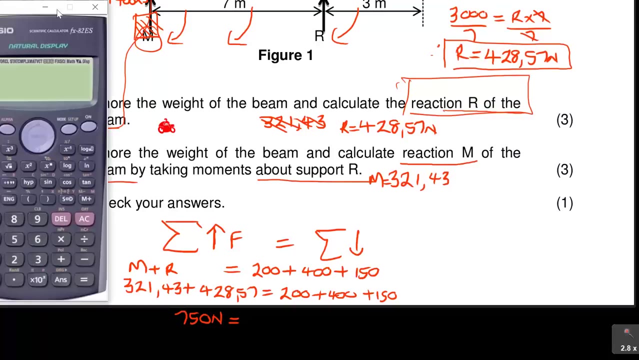 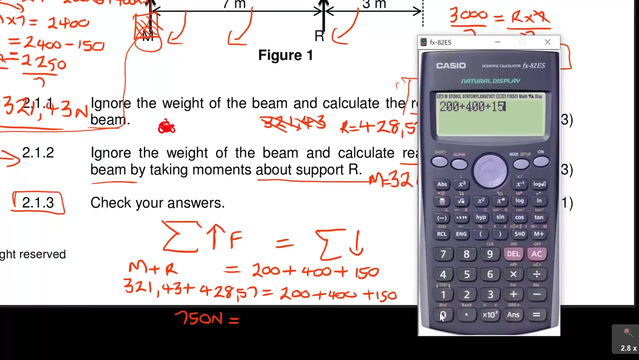 So now let's test that. In the first one we have got the 321,43 plus 428,, 57.. It gives me the 750.. So I've got 750 here. Newtons is equal to. so I test the other one, which is 200 plus 400 plus 150, and it gives me also 750.. 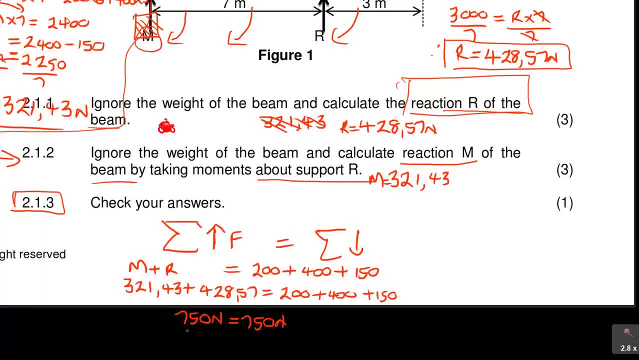 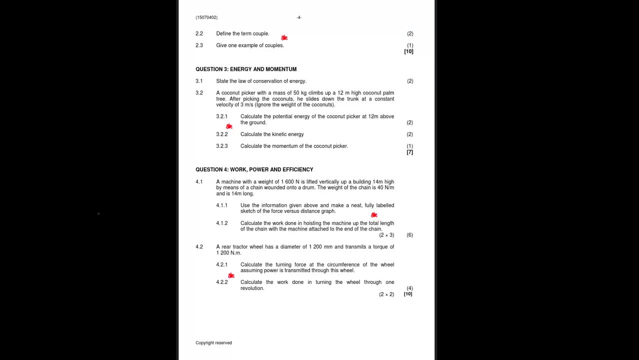 So you can see that my forces are balancing. It means my answers. in this case they're correct, So you can use that as a test. also When, even if you're not told to do that, you can use that As a way of testing your answers. 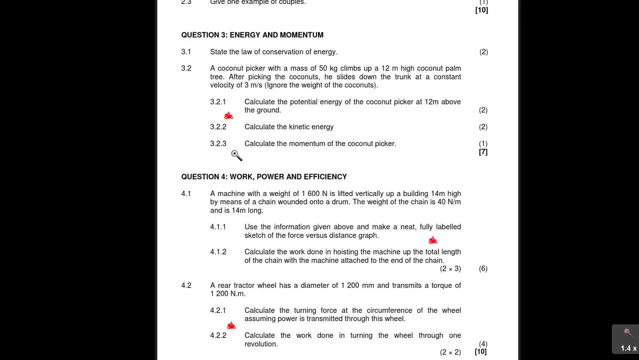 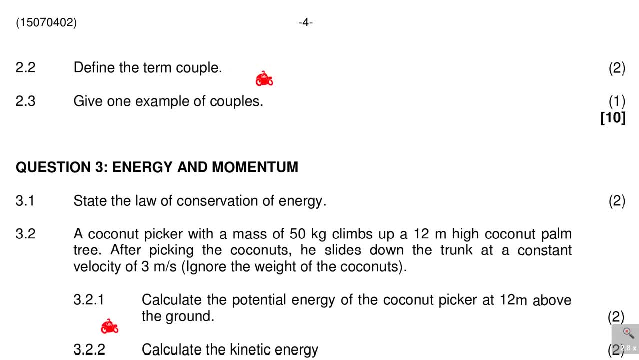 Now the next questions. that's question 2.2.. Still continuing on that question 2.2, these are common questions that I wanted to master so that you just ensure that you don't lose marks on this part. They like this question to say: define the term couple and also give one examples of couples. 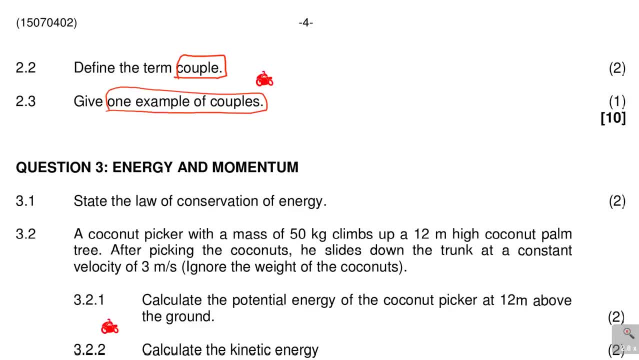 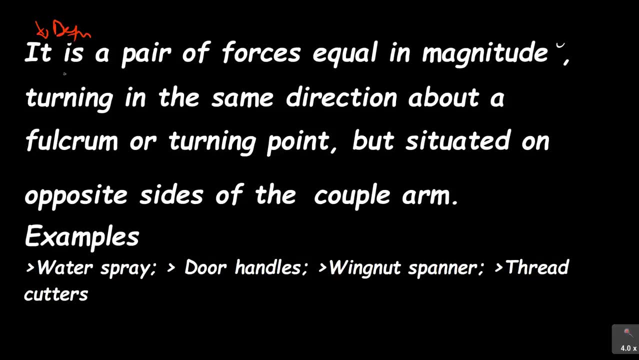 Please remember that These questions, you need to know them. It's two marks, and one mark First is about a couple. So this is the definition here: It is a pair of forces equally in magnitude. They will give you a mark there. 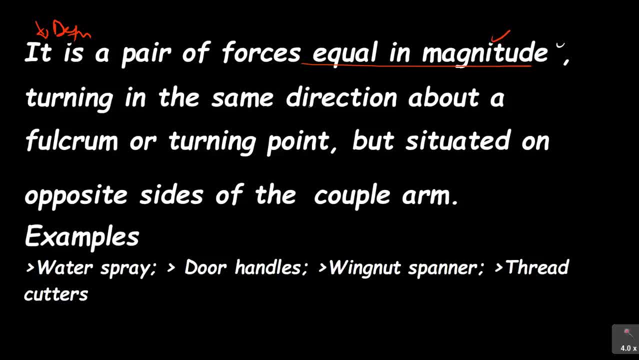 So it is a pair of forces equal in magnitude, turning in the same direction, about the fulcrum or turning point, but situated on the opposite sides of a couple arm. They'll give you that. So it is a pair of forces equally in magnitude, turning in the same direction, about the fulcrum or turning point. 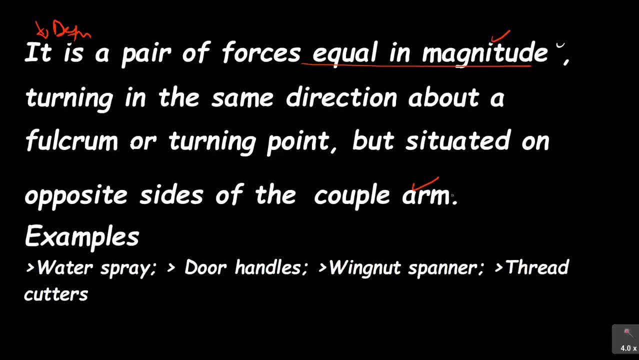 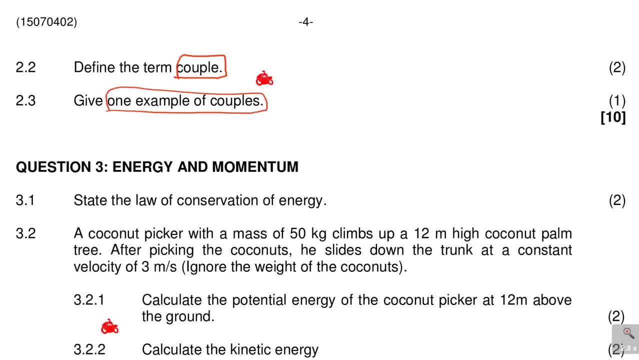 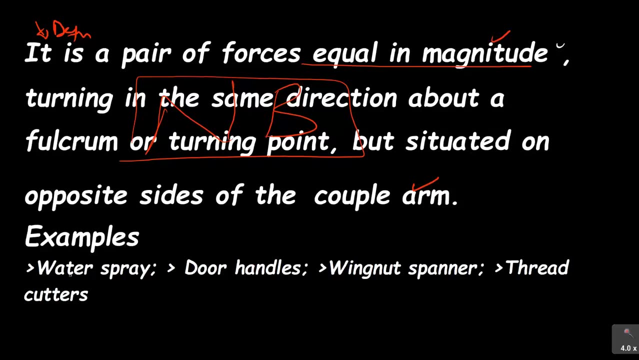 but situated on the opposite side of the couple arm. please remember, this is- and i'll say nb. you need to know this definition. they like to ask that and the next thing that they like asking is give one example of couples, and the common answer that you can bring here is: you can use a water. 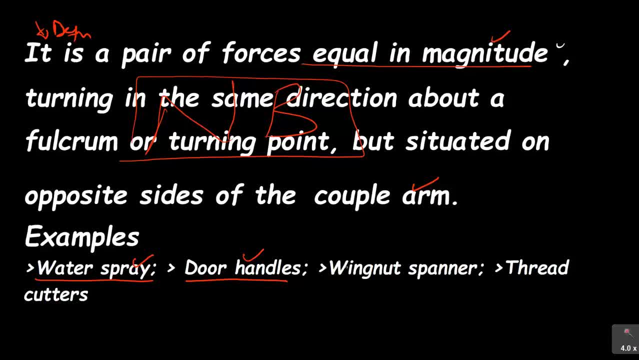 spray. that's where you use couples door handles. that's where you use couples wing nut spanner and then a thread cutter. now, don't forget, you can just master all these three must. at least make sure you must have three of these, because they usually sometimes says give. 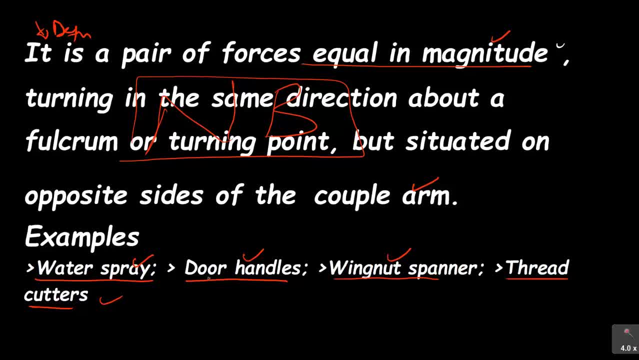 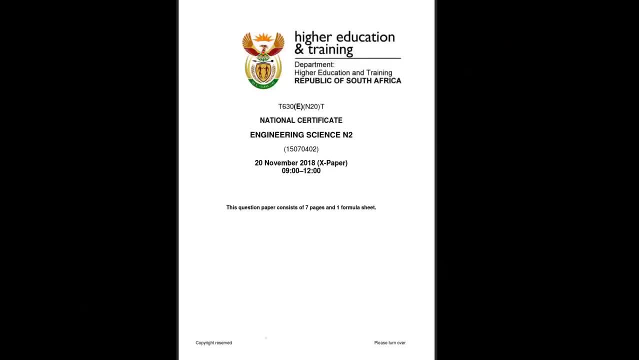 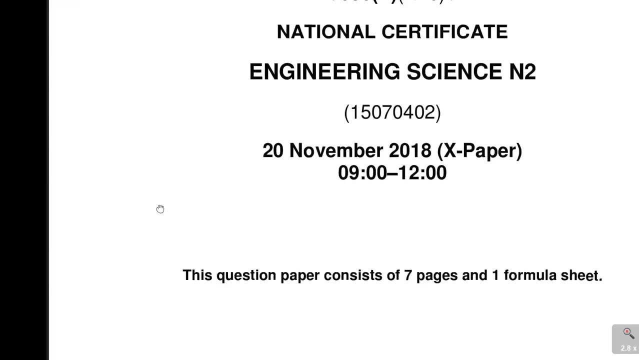 three examples, give two examples or give one example. the definition is a must, the examples: it's a must. don't forget this. i hope you are benefiting from this, guys. now let us move on to the next question. again, i'm bringing more, more questions to you, guys. 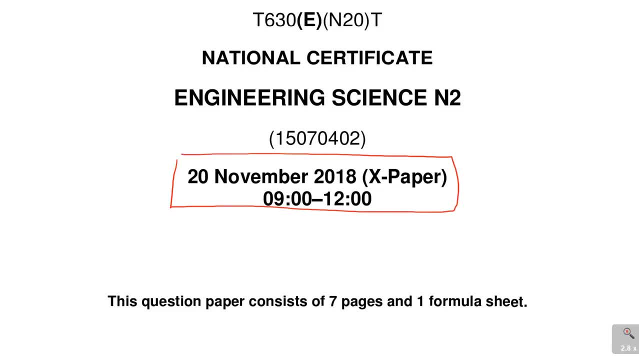 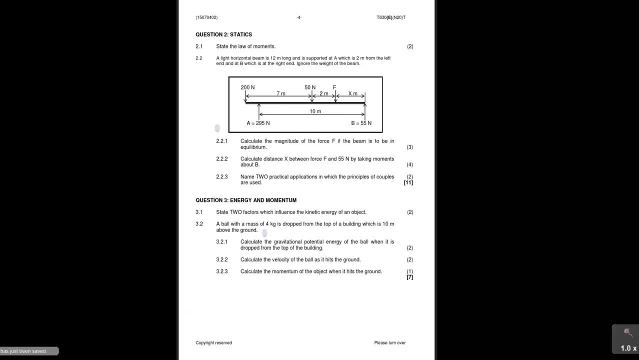 i'm bringing more questions to you, but, um, it is good this is a complete guide to uh, looking at moments. so that's why i'm looking at all these questions. so you see, this question it was in november 2018 and in this question i just took different questions. they've got different. 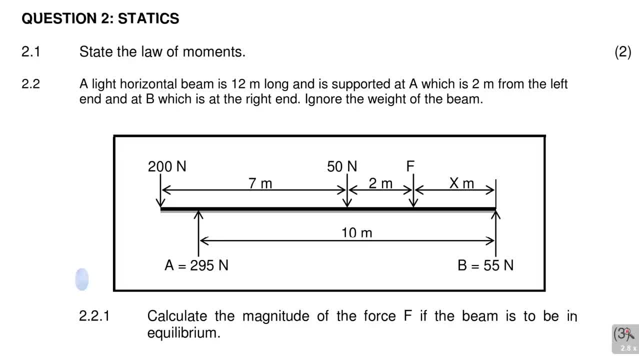 approaches, so that i try to cover almost everything now. question 2.1 here say: state: the law of moments. it's a very common question, also very important, uh, to master. now what does the law of moments say? the law of moments say the sum of that is the definition of the law of moments. 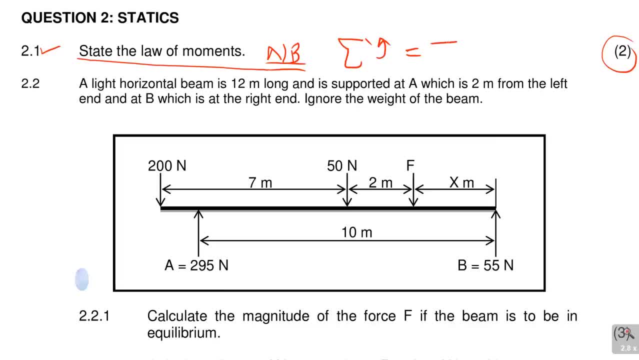 this is what you'll be defining. remember that we are defining this. what we've been talking about, what i say, it is: the law of moments says the sum of clockwise forces about a fulcrum is equal to the sum of clockwise anti-clockwise forces about a fulcrum. so i repeat, 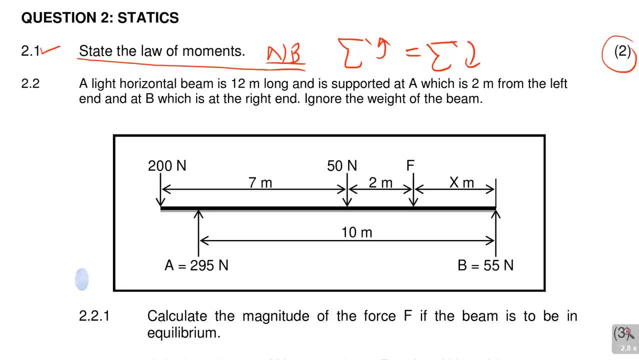 again. it says the sum of clockwise forces- this is the clockwise forces about the fulcrum- is equal to the sum of anti-clockwise moments about a fulcrum. i said forces, but i'm supposed to use moments. the sum of clockwise moments about the fulcrum is equal to the sum of anti-clockwise. 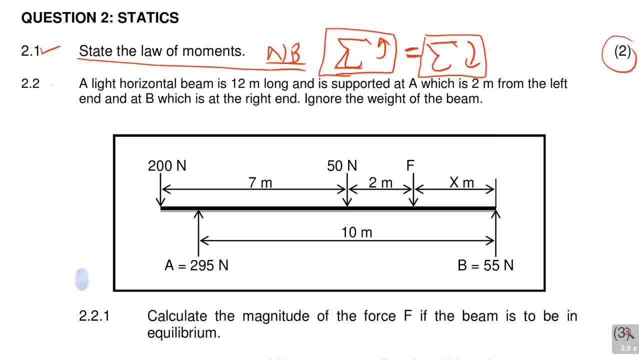 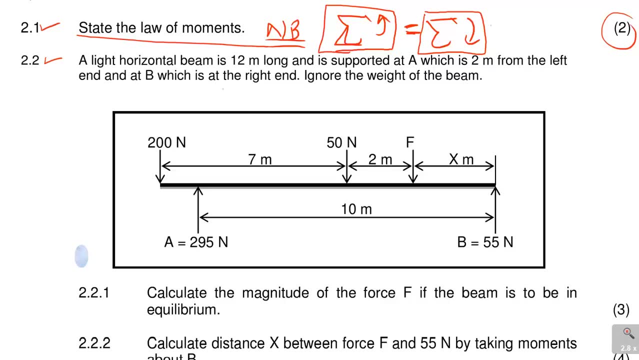 moments, about the fulcrum that is the definition of the law of moments. so remember that one is very important. all right, so let us look at the question, in this case question two. point two says a light horizontal beam is 12 meters long and is supported at a. 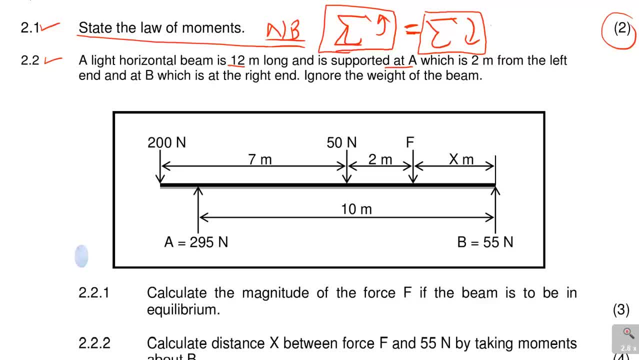 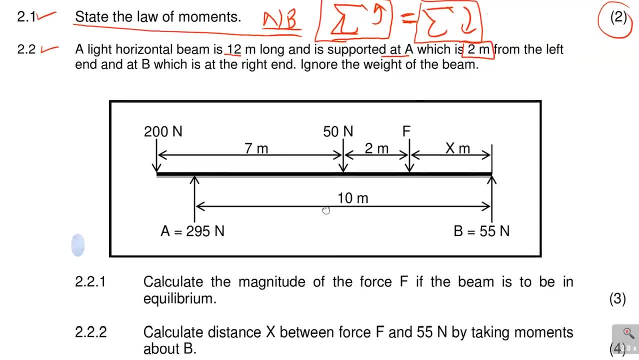 which is two meters from the left end. they didn't indicate, though, but they're saying, they're telling us it is two meters from the left end- and b, which is at the right end. you can see that. ignore the weight of the beam, so let's look at the information now. the first question says: calculate the magnitude. 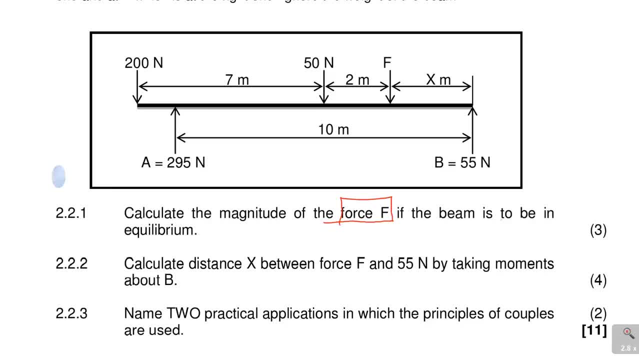 the force f if the beam is to be in equilibrium. so this beam is in equilibrium. they want the magnitude of that force f. now there's something interesting though they did here. they gave us a force there facing down. a force there facing down. f is facing down. look at the arrows, it is. 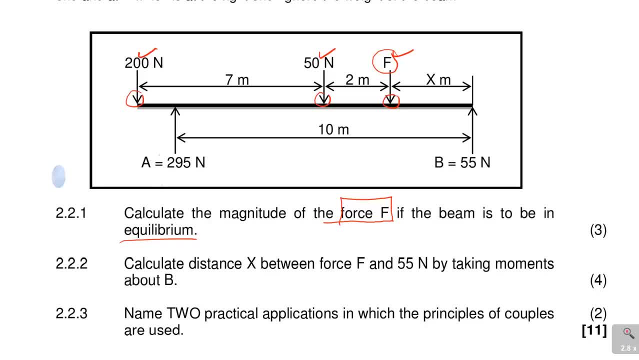 going down, it's going down, it's going down. and they also gave us a that is facing up and b that is facing up. so in other ways they calculated all these forces. what they usually wanted to calculate is calculate the forces or reactions at a and at b, and then after that they say test. 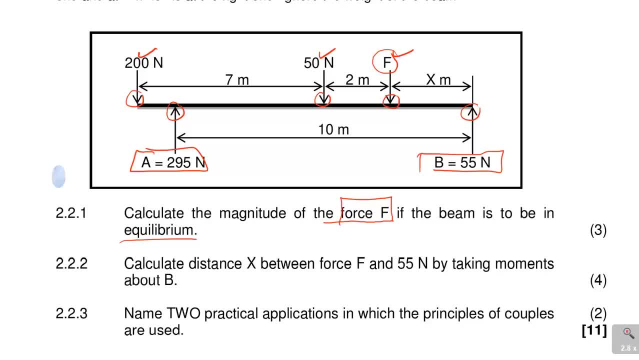 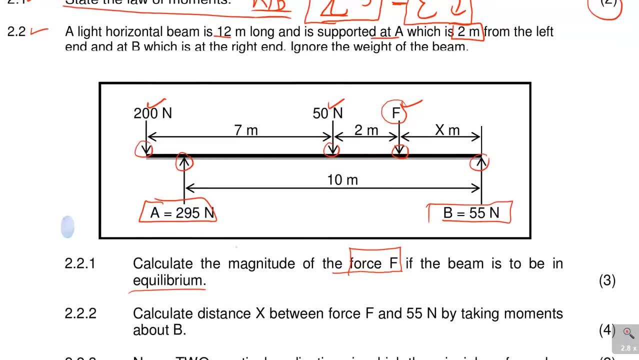 so here they've given you the forces. so now what you just need to do is to do the last part that you do for testing, and it will give you now that f. so how to usually test, remember we said when we're testing: sum of upward forces. 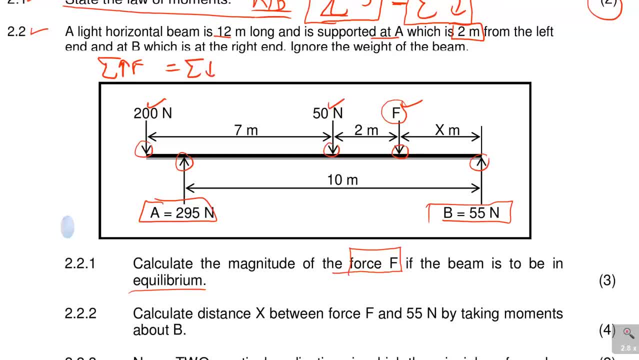 is equal to sum of downward forces. so now let us look at the all the upward forces. they are at a and b, which is 295. they're going up plus 55 is going up, is equal to look at all those that are going down, which is 200 plus 50 plus f. you see, that's what they needed there to calculate f. so 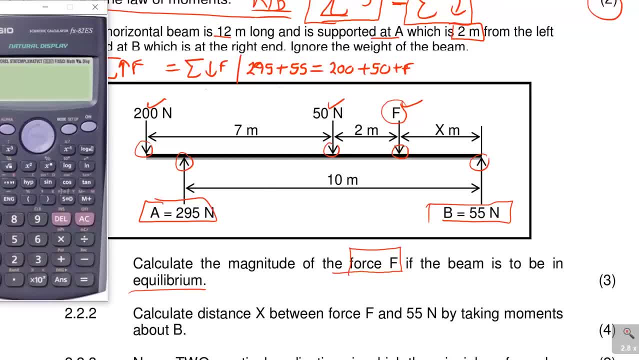 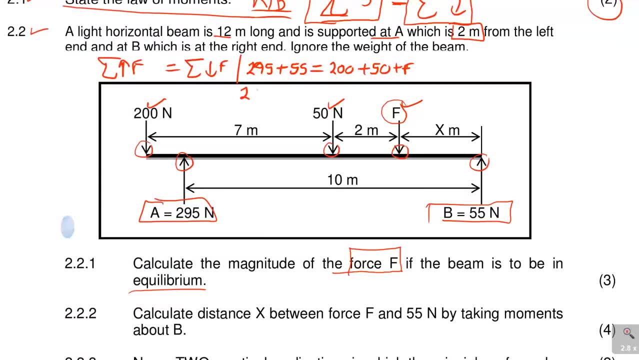 when you do that, you add 295 plus 55. actually you can do that once to say: 295 plus 55, take 200, this side, which is negative 200, take 50, that side, which is negative 50. remember, when you cross the equal sign, you change the sign that is now giving us f. now you can see, we can do this once. 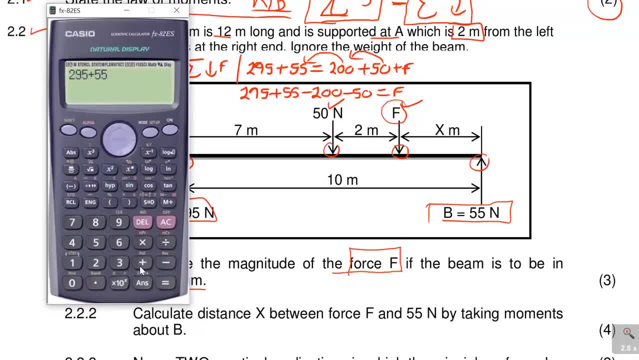 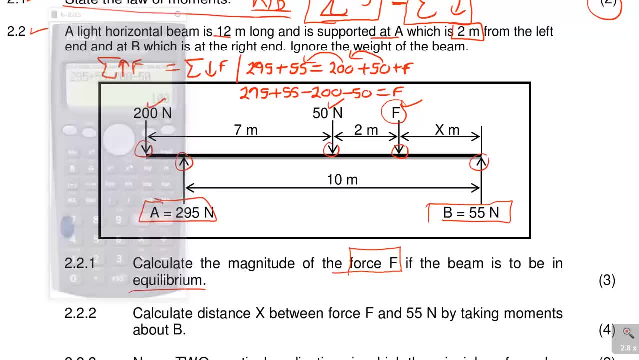 we make it to 295 plus 55 minus 200 minus 50, then that gives us 100 newtons, so f equal to 100 newtons. so that's what they wanted, they defined. so f is equal to 100 newtons. it's just just a good three max for you there. all right. and then the next one. i think you can see there's an x set, so just you can just have the x set. and then the next one, i think you can see there's an x is salt for whatever, and this one is the zero, because always half times the top is a positive three. so most of the times you tend to do the same thing. you can also do it twice. if you have the f, that's the one you need for the five, and then you can just simply give it to three or four as the number and keep doing that until the last one is. 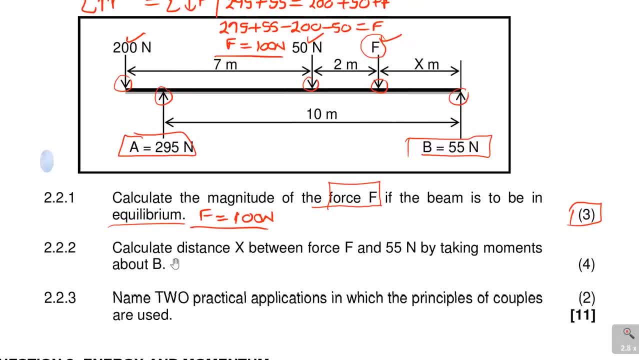 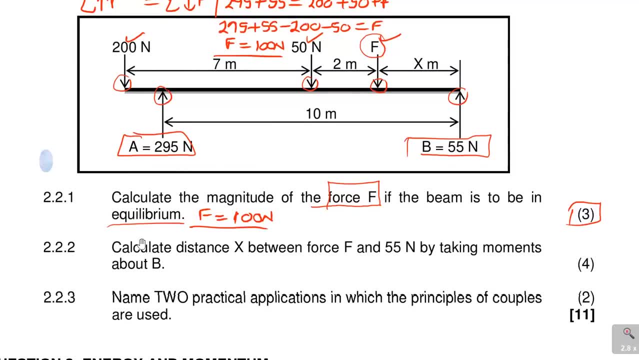 a positive three percent plus p times, so that's the other half which is the most effective. so let's give a good three to say: calculate, calculate distance X between force F and the 55 Newtons by taking moments about B. you see, now they are saying: take moments about P and when. 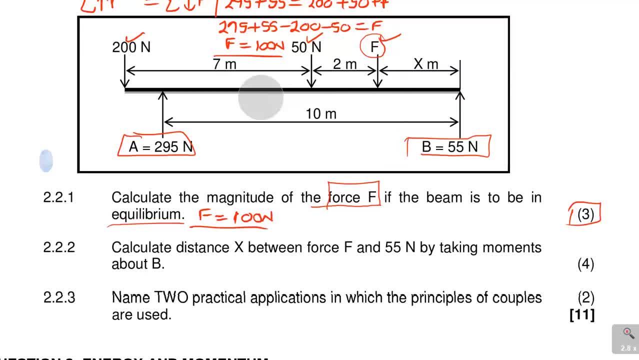 you take moments about P, it'll make you calculate that distance: X, M. so if we're going to take moments about this force, P, you ask yourself what is the effect of all the other forces, which is that, that, that and that. so let's start with the. 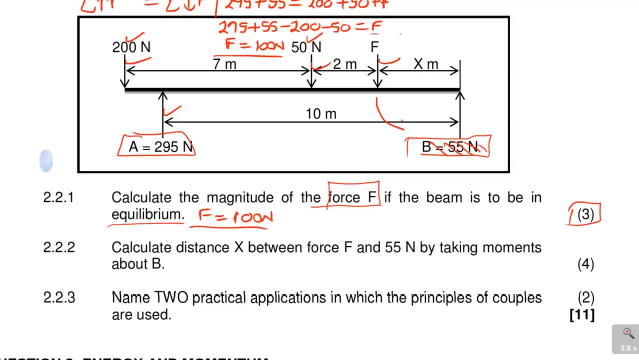 forces that are facing down. you can see about P. it will make this beam go in this direction, which is anti. even this force will do anti, anti, clockwise. by saying anti, even this other force, it will produce an anti-clockwise. but look at, a is the only force that will do. 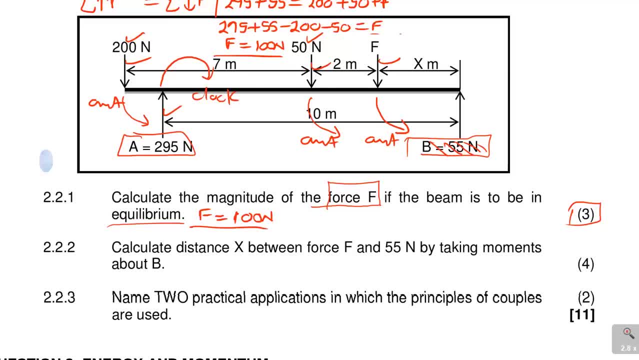 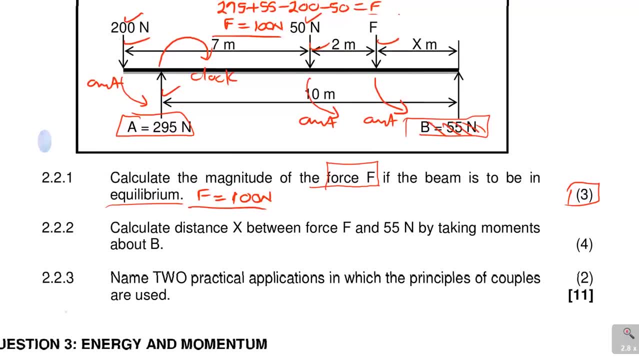 a clockwise. so now I can actually use this information then in here to calculate. I'll just use this space here. remember it says sum of clockwise moments is equal to sum of anti-clockwise moments. so let's look at them now. there which one is the clockwise moment? it's a which is 295 times. what is the? 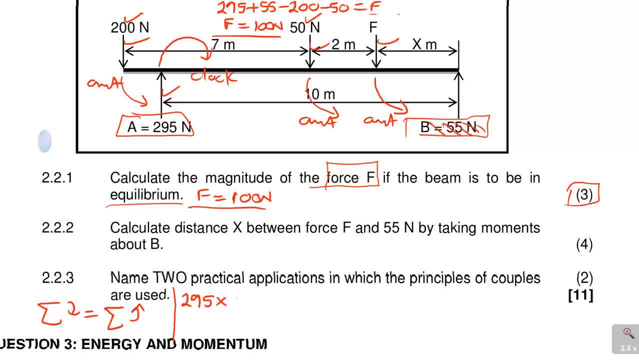 distance of a from B, which is 10 meters then they're showing us, is 10, if there is no other force of clockwise is equal to- you start with it- 200. what is the distance of the 200 from the 55? I think they say. 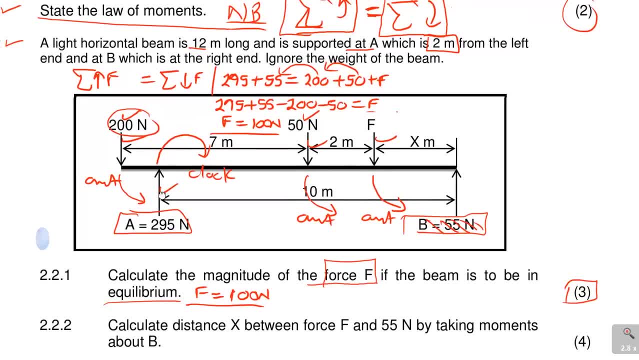 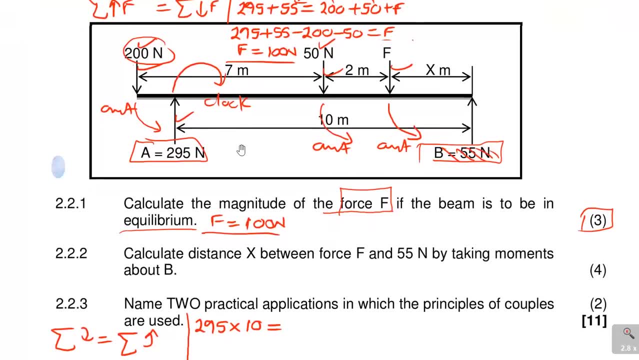 we read this beam. they say: the beam is 12 meters long. you can see a and in the 200 is far end. so that is 12 meters long. so it's 200 times 12 times 12. that's the first one plus. and then you look at the next part to say what is the 50 Newton a? 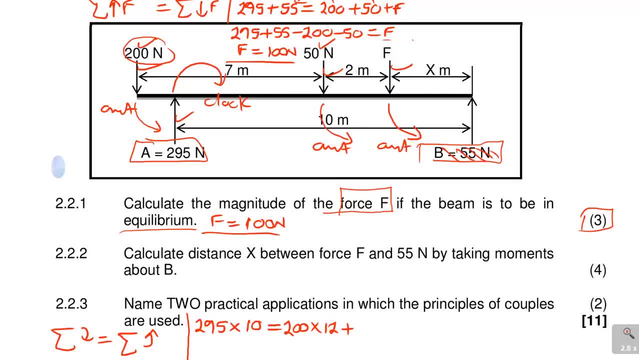 force from B. so you can see that the 50, it is this distance all together, which is you need to add 2 and X, so it is equal to 50 times 2 plus X. that is the first part, and then the last one is F. you see that F, F times X, which is equal. 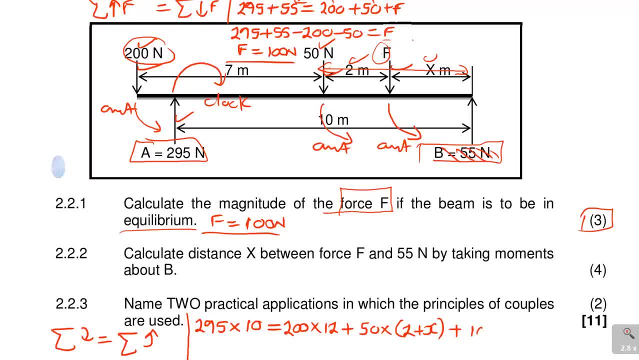 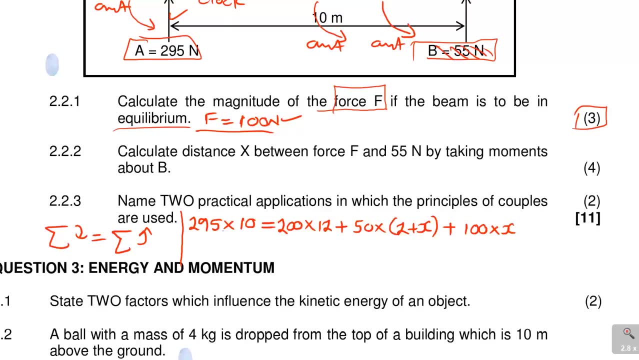 to plus the force F, which we found it was 100 Newtons, remember. we calculated it ten times X. so these are the forces that are acting, and then you just need to solve X. so what it do is 295 times 10 is 2950, is equal to 200 times 12, I think. 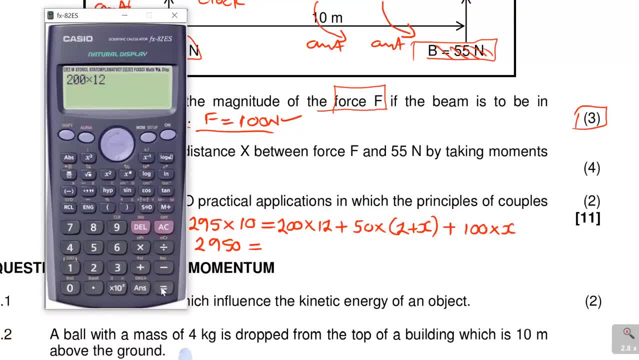 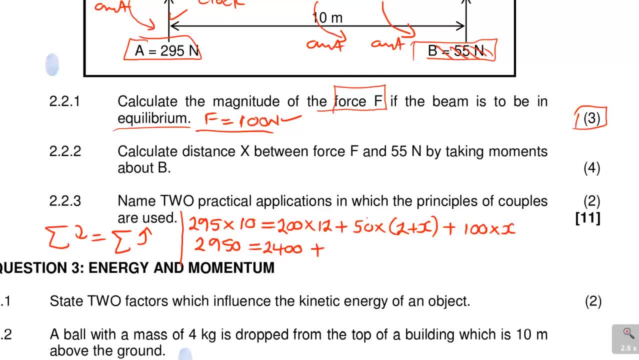 it gives me 200, 250. 250 times 12 gives me 2400 plus. you open that bracket 50 times 2 and 50 times X. 50 times 2 is 100, plus 50 times X is 50 X, and then plus 100 times X is 100 X. so 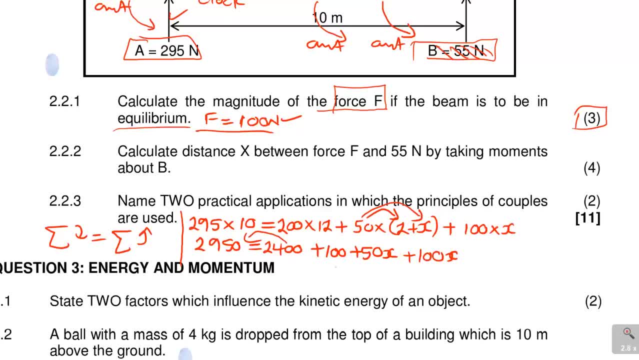 you see how you solve it. take 2400 that side, take 100 that side, you believe to decide on the other side. so you'll have to: 950 minus 2400 minus 100 is equal to 50 X plus 100 X is 150 X. so when you simplify, finally you will have: 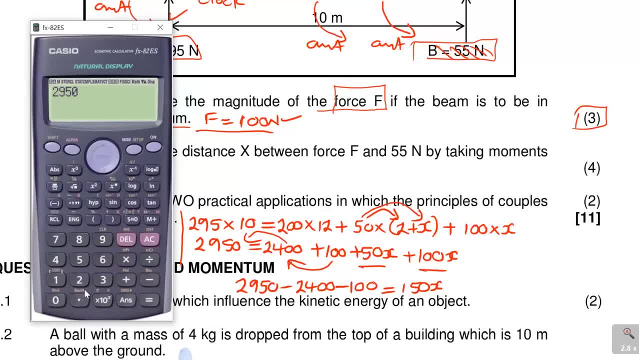 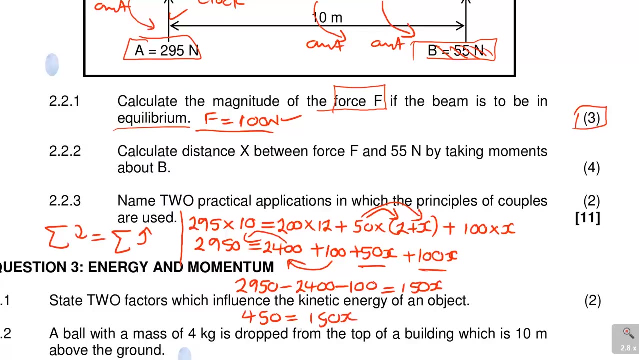 to 950, right minus 2,000, right minus 2,000, 400 and then minus 100. if I do that, it give me: 450 is equal to 150 X and divide by 150, so that will remain with X. you divide 400 by 150, so you will have. 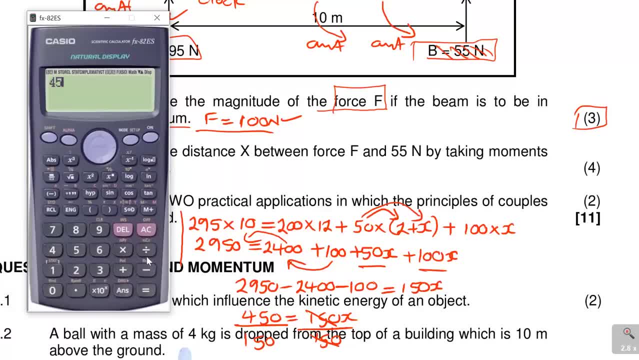 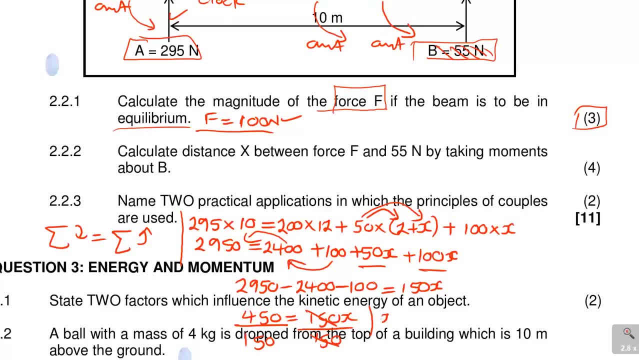 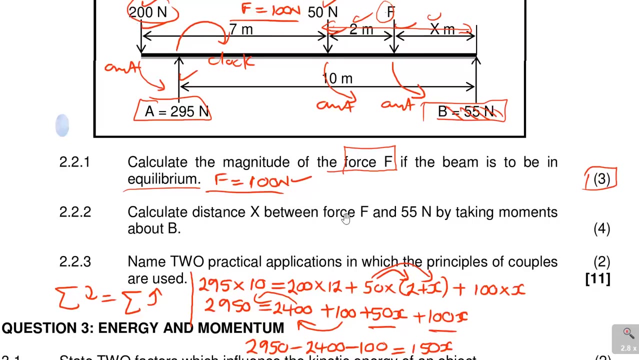 in this case 450 divided by 150, and then gives us three. so I can see that here X is equal to 3 and we're dealing with meters. so X day that distance that they wanted, a, it was three meters. so they say: calculate the distance X between force F by taking 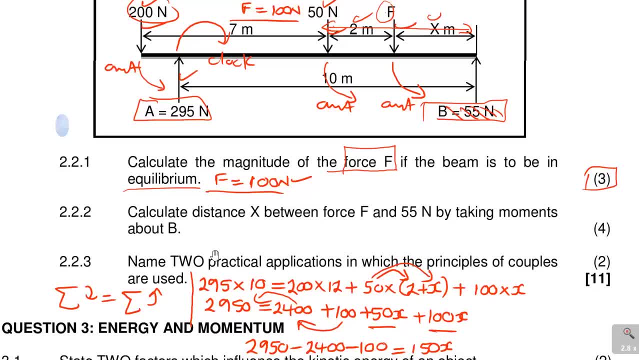 moments about P and then say the next one says: name two practical applications in which the principles of couples are used. see this question again. it is coming to practical applications by which the principles of couples are used. is the same question I said previous to say you definitely need to. 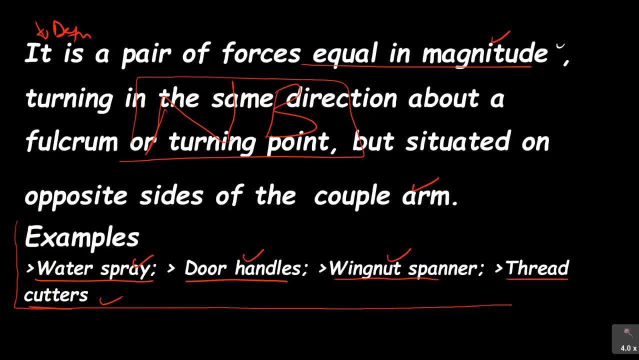 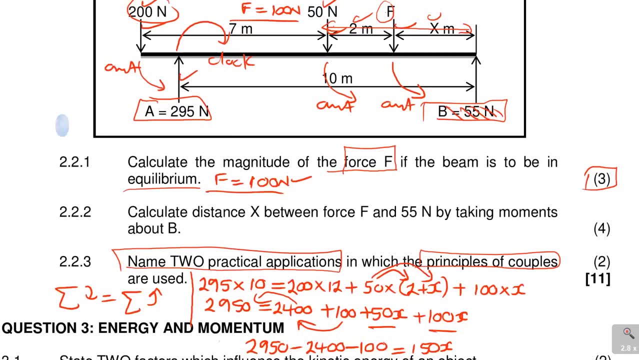 know where to use them under examples. so the practical applications here they wanted. you can say water spray, door handles, wing nut spinner and thread cutter- they like such questions. or to say define couple, as we said. so that is this particular question that they wanted. so I think I've done three more. 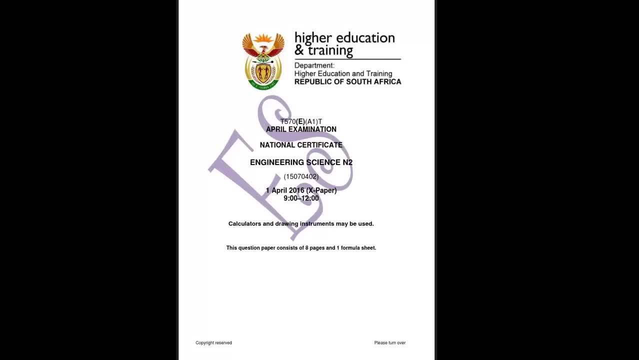 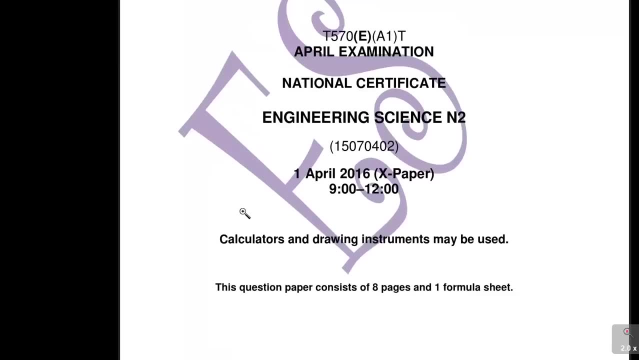 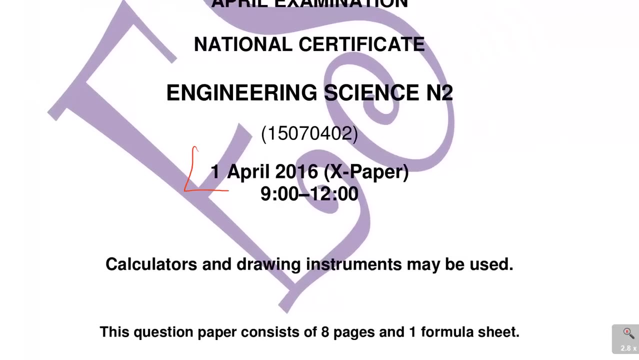 questions and I hope this is benefiting to you guys. but now look at this one. I'm not going to work on this question because of my time, but the last question I had wanted to do for you was this question on April 2016, and I wanted to 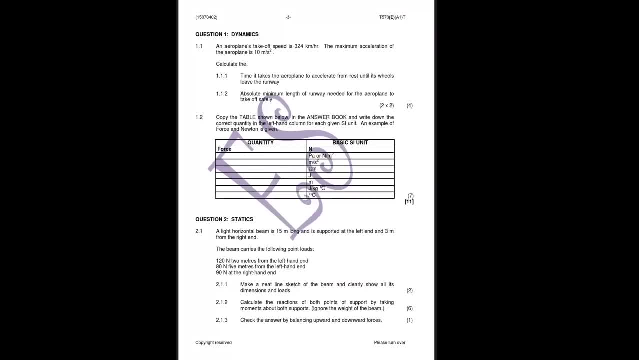 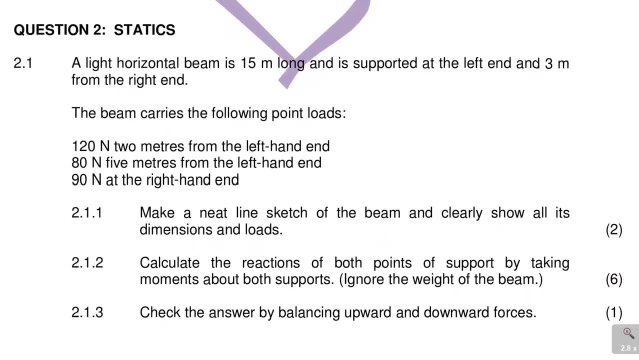 try it now, guys. you try this question. let me bring it to you. I want you to try this question and there is question two. just look at this question. it says a light horizontal beam is 15 meters long and is supported at the end and its ability is supported at the end and three meters from the right end. the 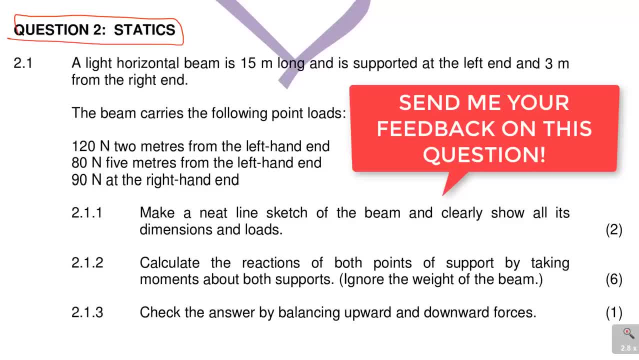 team carries the following loads: 120 neutral 2 meters from the left end and 20 new tons five meters from the left end, and 120ö and end 90 newtons at the right hand end. so they give you those forces that are facing down and 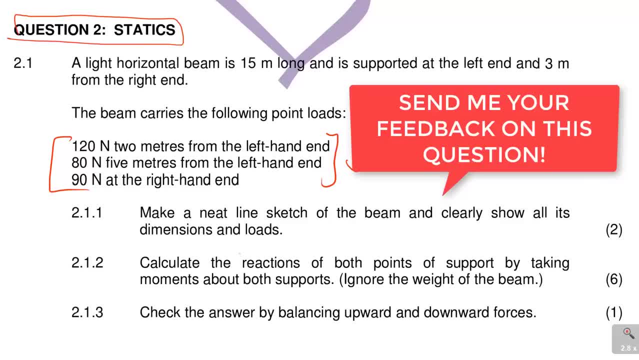 then says: make a neat line sketch of the beam and clearly show all these dimensions and loads to max. calculate the reactions of both points of support by taking moments about both supports. ignore the weight of the beam a good six months. then says: check the answer by balancing upward. 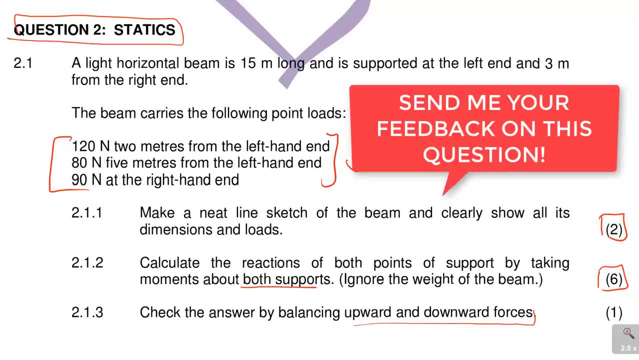 and downward forces, and then you do the same and we've been looking actually at all these. we've covered that. we've covered that. we've covered that now. i wanted to try this question now. give me feedback. if ever you struggled, and if you guys give me comments, that is when i'm 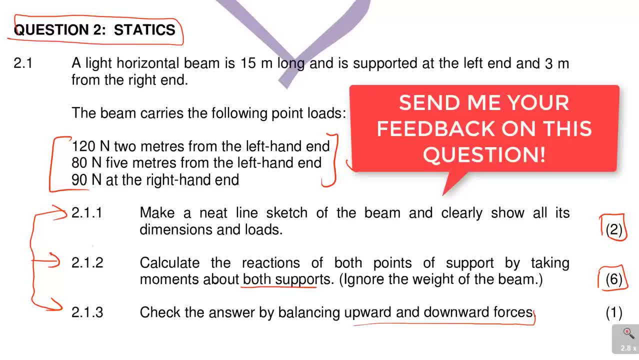 going to be able to bring this question to you, but if you're not going to comment that you're struggling, i will assume you guys managed to get this question correct. if you are struggling to find the answer to this question, remember to send us a comment, uh, or below this video, to say: please can you do the last question. 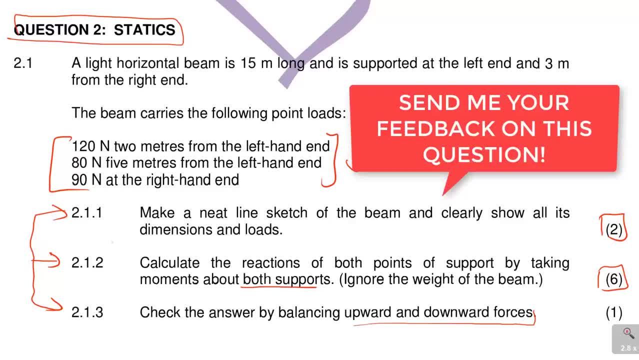 just remember to say: please, can you do the last question, or you can actually express where you are having a challenge, and then i'm going to do a video that i will post specifically for you. who is having a challenge on this question? and i think this is not the end, the last part of 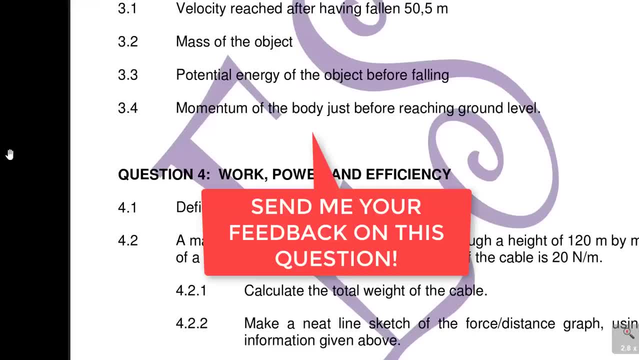 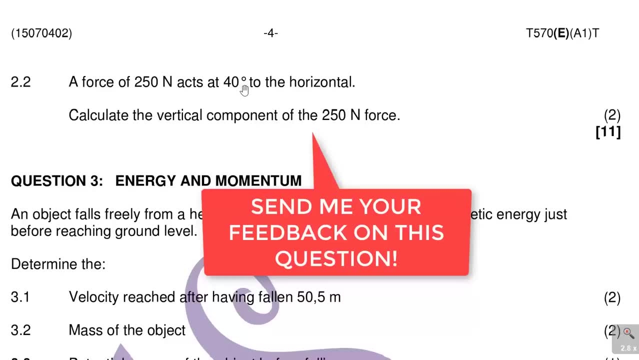 the question here because i don't- i didn't see the final mark, and then this is the end of the question- says a force of 250 newtons x at horizontal, at 40 degrees to the horizontal. calculate the vertical component, okay, of the 250 newton force. so this one they are saying you have. 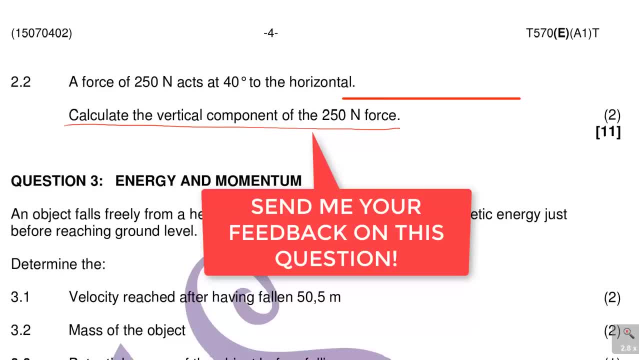 got, um, something like this: you have got a horizontal and in this horizontal we have a force that is acting at, uh, like that. see that we have a force that is acting at 40 degrees to the horizontal, as you can see that, and this force is 240 newtons. now they say: calculate the vertical component. nice, remember. 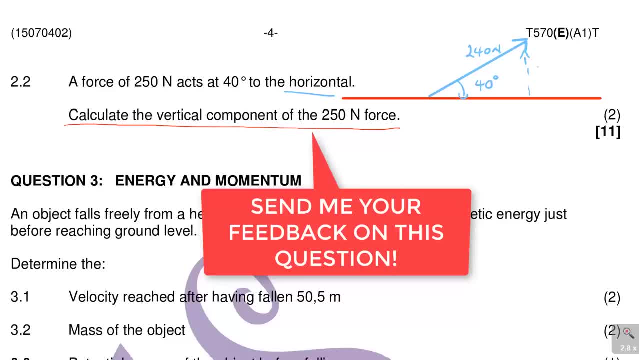 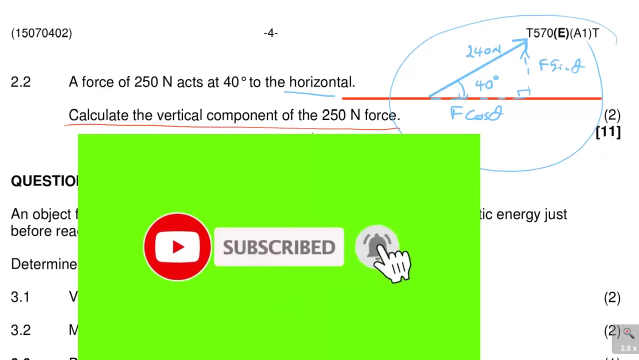 this force has a vertical component and this force has also a horizontal component. this is 90.. if you still remember, vertical is f sine theta, horizontal if it's f cos theta. now again, if you're going to struggle with this question, remember to send me and a message down below the video to say: please can you also do question 2.2, because 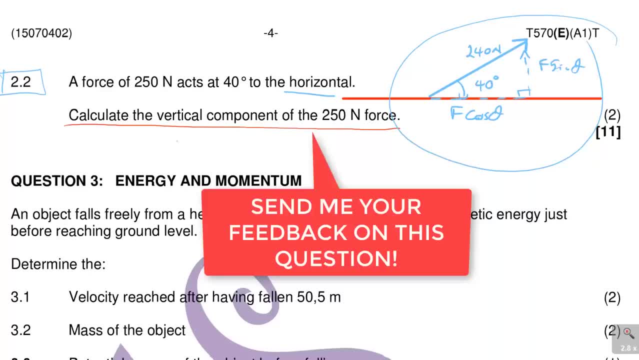 you're struggling is a good, simple question, but because of time, i'm not going to continue that, because i wanted to say much concerning that question. so, guys, we've come to the end of our lesson. remember to subscribe again to our channel if you have not done so.